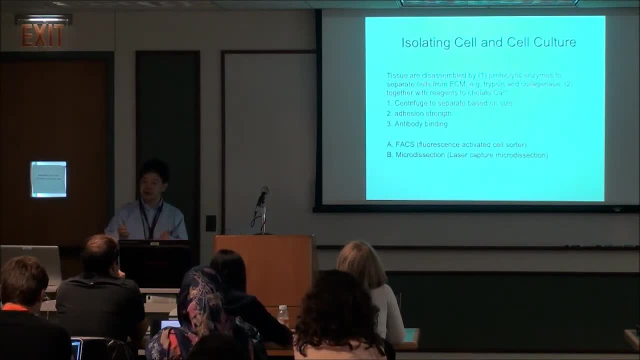 So they will cut certain receptors on the cell membrane, like integrins, so that they will no longer anchor on the neighboring tissue. Okay, Another thing: you will also include so-called casein. Casein will chelate. sorry, it's basically chelator to deplete casein in the exercise space. 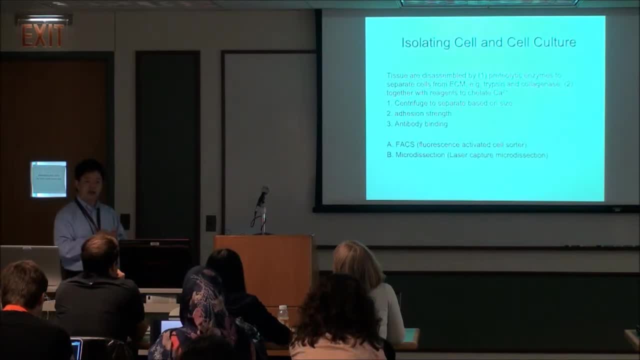 Whenever casein is gone, the cation which is helping to join the cells will be collapsed, okay, and therefore cells will be detached from each other. okay, So now you can cut the cell out as a sheet from tissue. You will separate neighboring cells using a tissue. 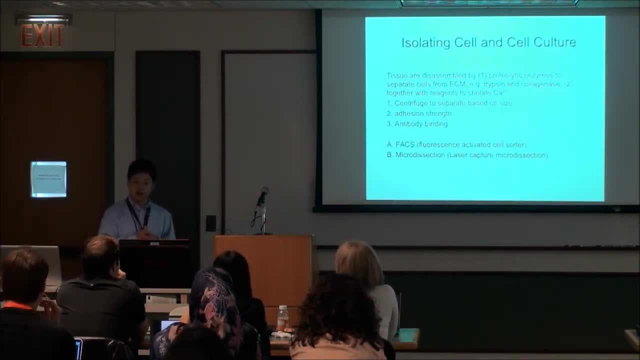 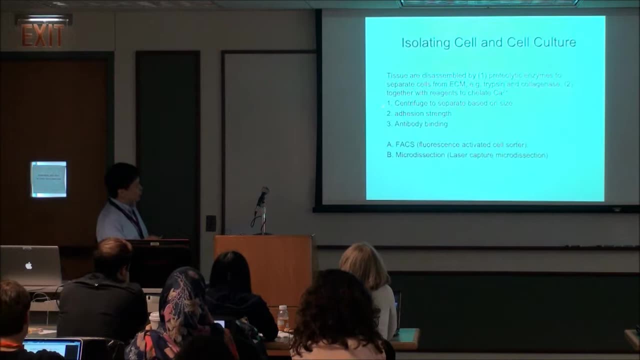 Using the chelator or casein, so they will be individual cells, okay. As long as you got different kind of individual cells, you have different ways to separate them, okay. The first one is very cruel and simple. You basically can directly subject the cell population on the centrifuge- okay. process. 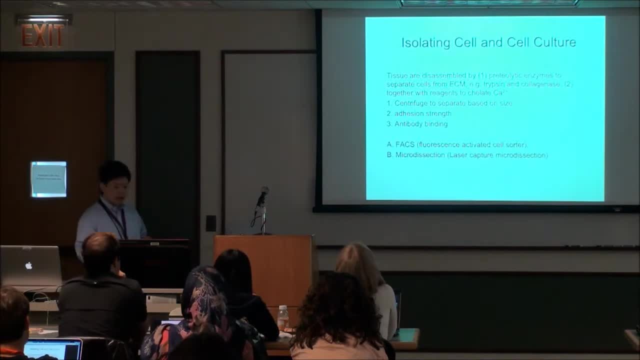 After centrifuge, based on size and shape. basically the cell will be separated at different speed, okay. Another one is called adhesion strength. So different kind of cell, their adhesion process is quite different. If you coat, for example, a dish with, you know, adhesion molecules and culture this mixture cell on the dish. some cells will adhere fast, some cells will take much longer, okay. 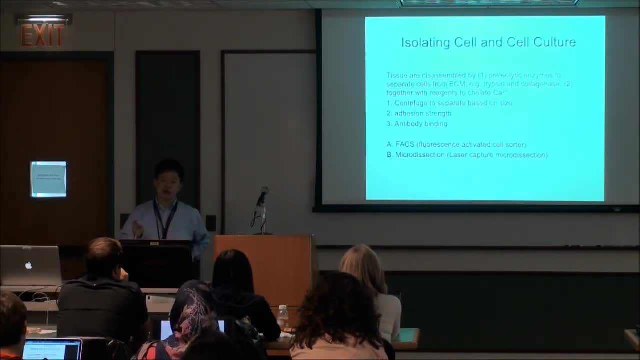 So you can allow a short period of adhesion and then wash away the rest. You will collect cells which adhere fast. okay, But these two methods are in general relatively non-specific. You can imagine right. Probably the cells adhere fast, contain multiple types, okay. 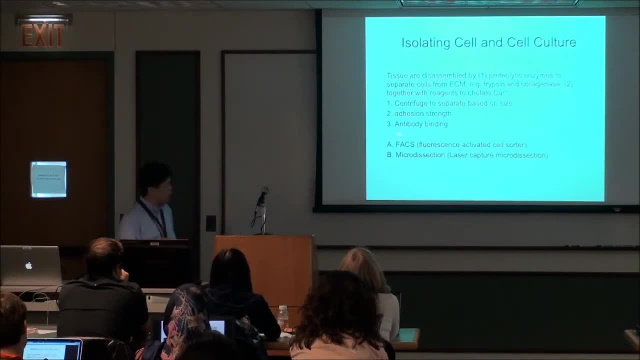 There will not be only one. So if you are particularly interested in certain specific cell types, usually antibody will be the way you want to. you know choose. So, for example, if you are interested in specific cell type and you know there are some specific receptor on cell membrane, 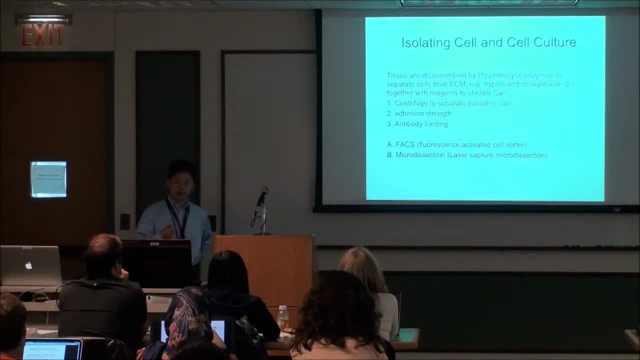 you can choose the antibody to label these receptors, okay. And then you can use like magnetic beads or other beads which will specifically bind to the antibody to extract and isolate the cell you are interested, okay. So these will provide relatively high specificity, okay. 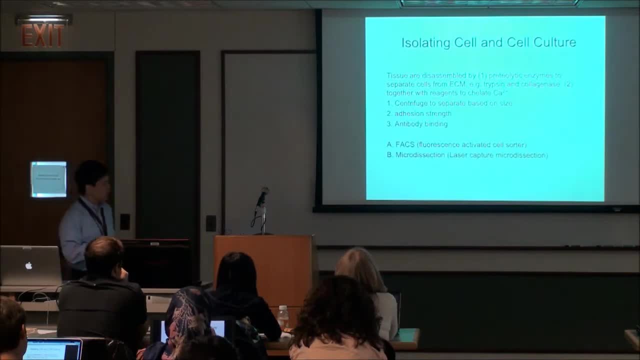 And there are other two advanced technologies. One is called FACS- fluorescence activated cell sorter- okay- which will provide very powerful and high specificity isolation of cells, And another one is macrodissection, which can be very useful for a specific or unique cell. 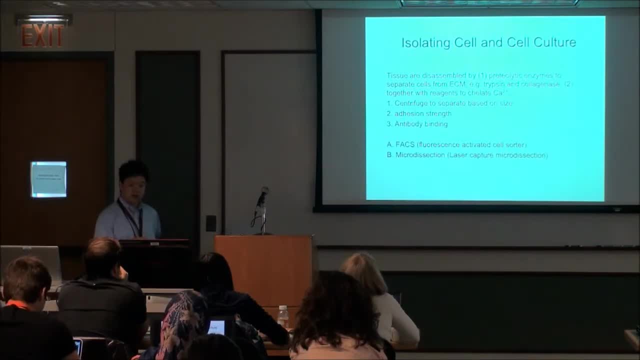 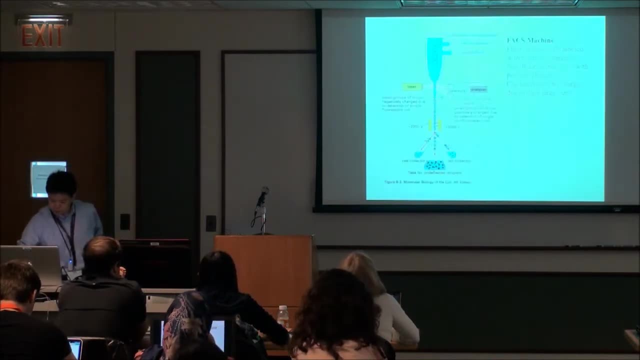 Unique isolation of cells, particularly for solid tumor cells. okay, This is called laser capture dissection. I'm going to introduce these two specifically in the next couple of slides. So first FACS machine. So FACS machine is called basically fluorescence activated cell sorter. right, 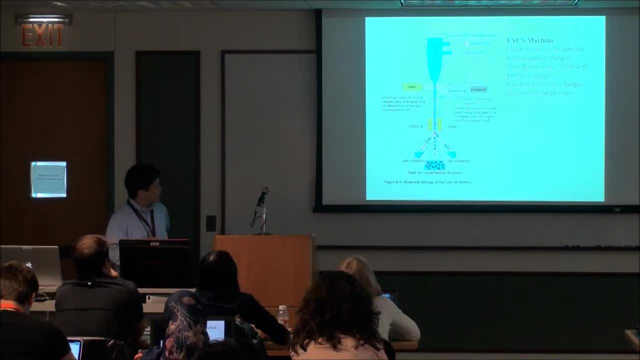 And this structure, this thing you can see. if you got a mixture of cell population, you can inject into this channel And then there will be a sheath flow. okay, High speed sheath flow will flow through this very narrow channel and wrap the cells going through this channel. 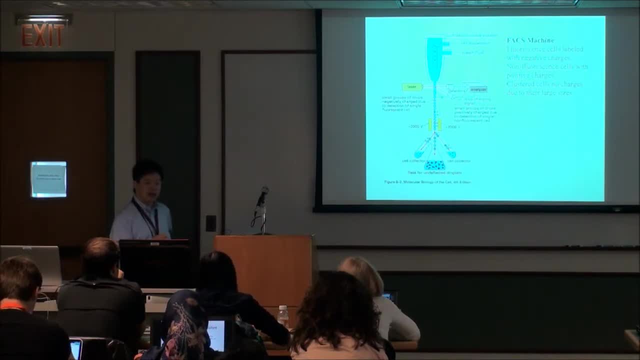 And in this channel, most of the cell will be in the single cell status, okay, although some of the cell cluster will also occur, But this will be discussed, as you can tell, later. So first thing, of course you have cell mixture. 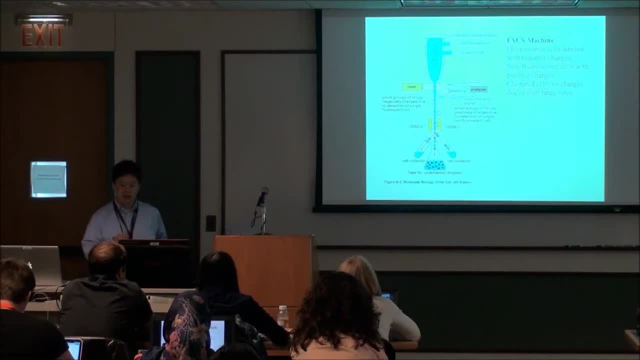 And if you are specifically interested in certain types, you can use antibody to label these respective cells, as I mentioned right, recognizing some membrane receptors And these specific cells will be fluorescenced. okay, And when? the cell mixture going through here? 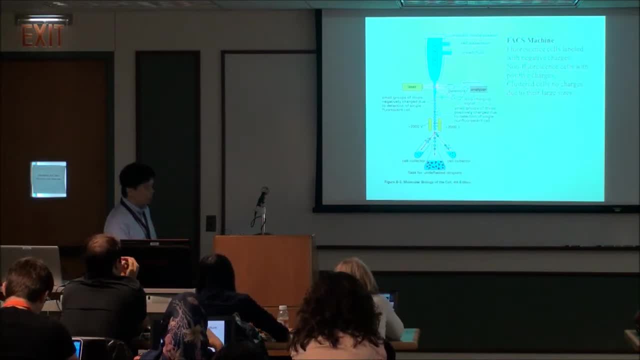 whenever they detect, for example, a laser, detect a fluorescence, that's the cell you want, right? And when they pass it, it will label with specific charge, such as in this case, a negative charge will be applied for the cell you are interested, okay. 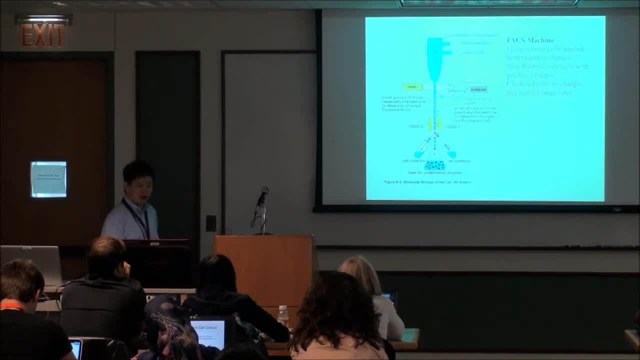 And other cells will pass through without being, you know, labeled with charge or labeled with positive charge. Okay, So when they go through, here there's another electric field, The cell you are interested, which is labeled with negative charge, right? 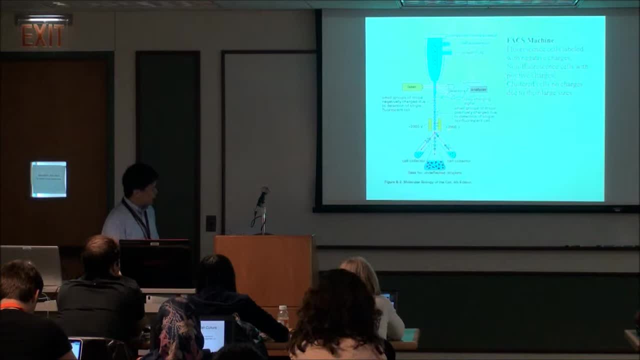 they will be pulled by this electric field towards the right. okay, I think the color labeling is wrong in this cartoon, but you got the idea right. If the cell you are interested in labeled with negative charge, they will go to the right side okay. 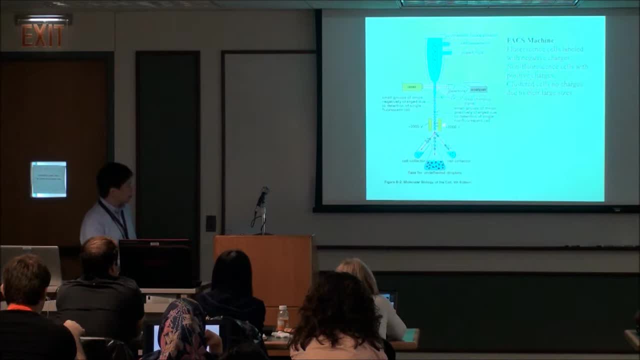 So these are cells you want to collect. okay, Other cells? they will either go to the left side or they will be- not, you know, charge labeled. They will go to the center place. This will all be discarded. in this specific case, 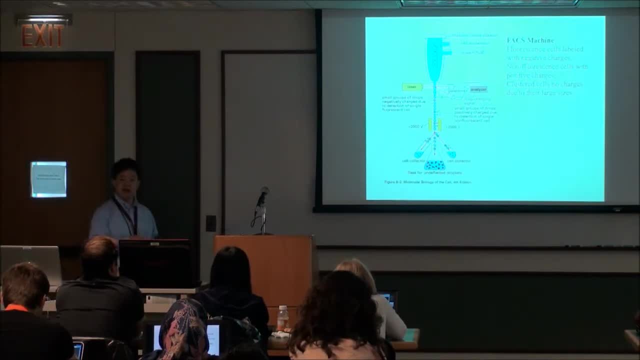 Is it clear. So you can imagine. if you want to simultaneously isolate two types of cells, you can do so as well, because you can use two kinds of antibody right labeled with different color fluorescence, So when they go through this laser detection first, 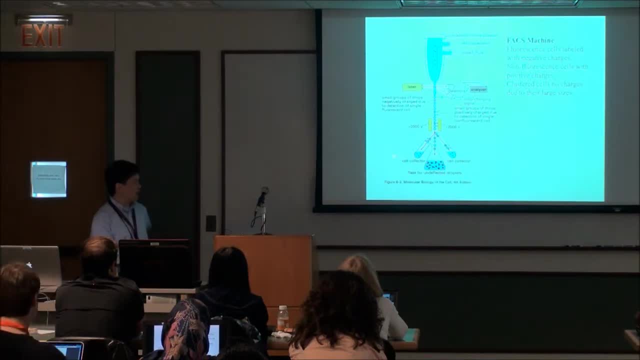 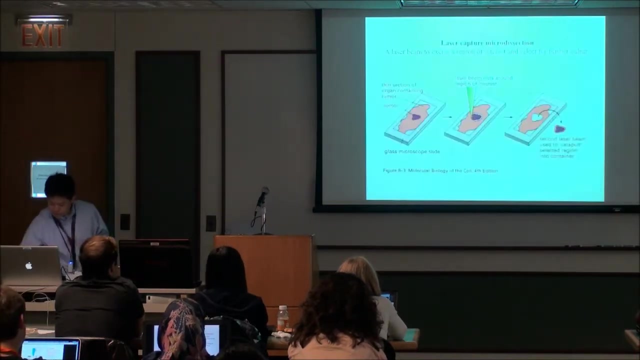 they will be labeled with like negative charge and positive charge. Then you can collect two cells at the same time. Is it clear so far on this? Okay, So this is a very convenient and powerful technology to separate and isolate the specific cell types you want, okay. 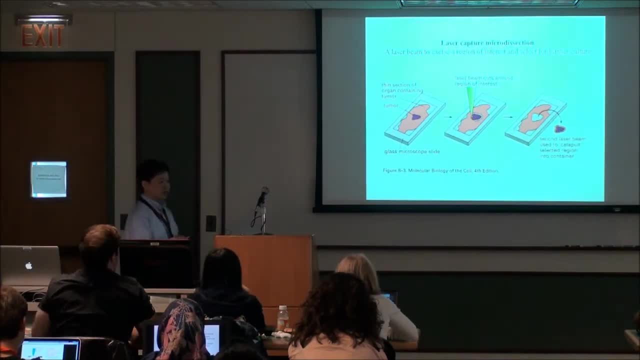 And for some specific occasions. for example, these are solid tumors. You can direct collect the species right And in the center you can. you know like stain these tumors And you know in this part they are concentrated with a very few tumor cells. 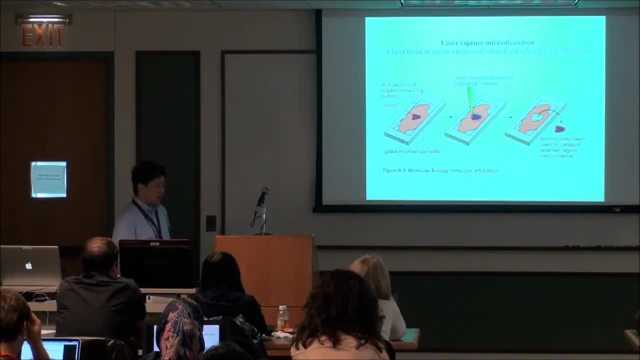 Then you can use this laser capture micro dissection easily just to cut out. Use one laser and use another laser to just flip to another. you know collecting dish. Then you collect all the relatively few, you know group of the tumor cells. okay, 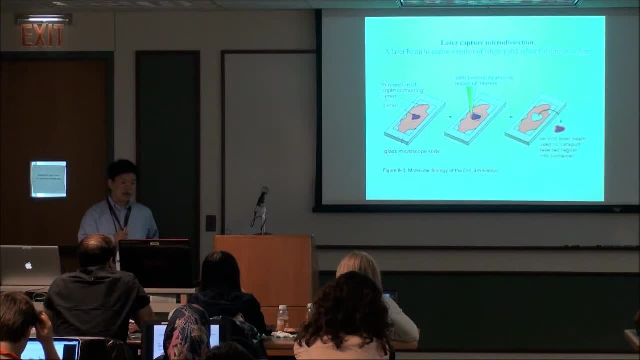 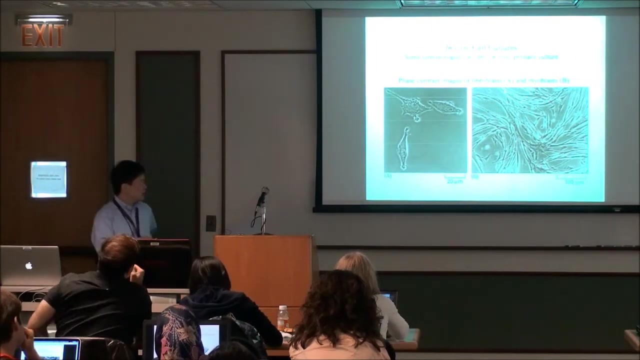 But this one is relatively limited, Only very useful if you are collecting the tumor cells- solid tumor cells- in a concentrated area. okay, So this is basically the cells. After you collect, you culture dishes. okay, I want to introduce some terminologies because some of the you know different fields. 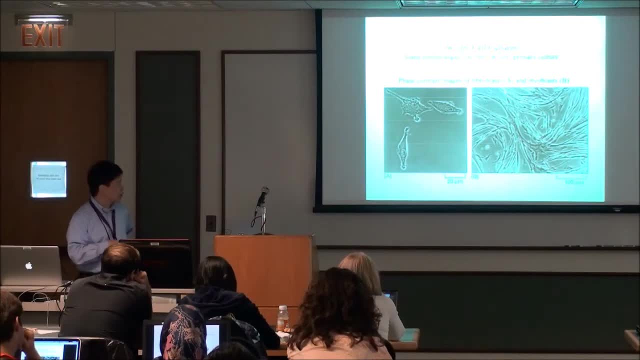 they call these different cells different names. So one is called in vitro. For chemists in vitro meaning protein in solution, right. But for physiologists or biologists usually in vitro, meaning the cells culture on dishes okay. In vivo means in the animals or in the body. 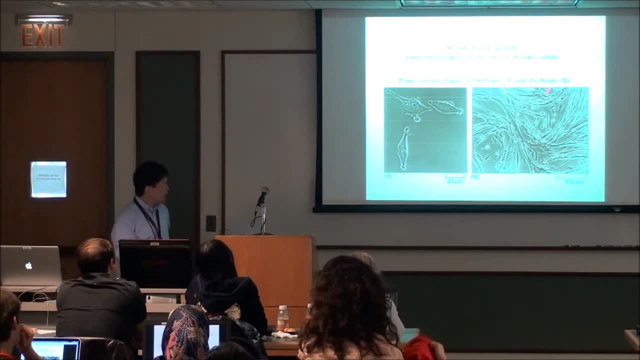 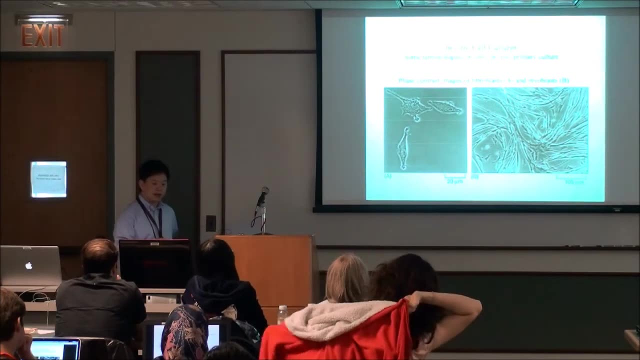 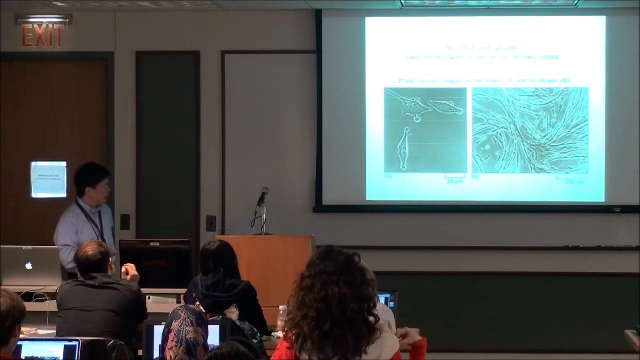 Okay, And the cells you directly collect from the tissue or animals- These are called primary cultures. okay, And you can already know if you culture a different kind of cell. they have different morphologies, such as fibroblasts on the left and myoblasts on the right. okay, 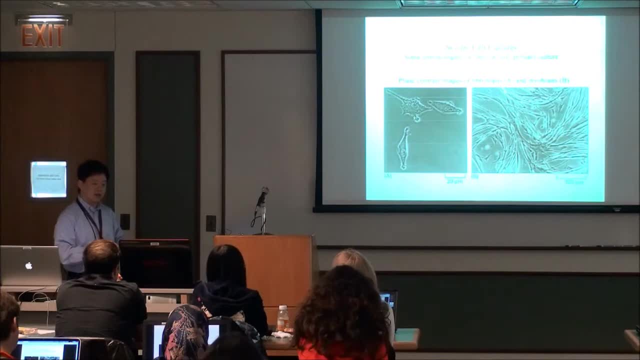 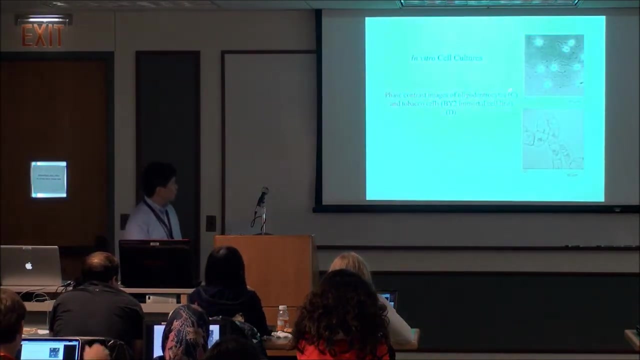 After you collect these specific cell types and culture them, they already have different phenotypes. Therefore, you can culture them, grow them and study the you know functions or these proteins inside them. Okay, There are another two kinds. One is called oligodendrocyte and the bottom one is called tobacco cells. BY2- immortal cell line. 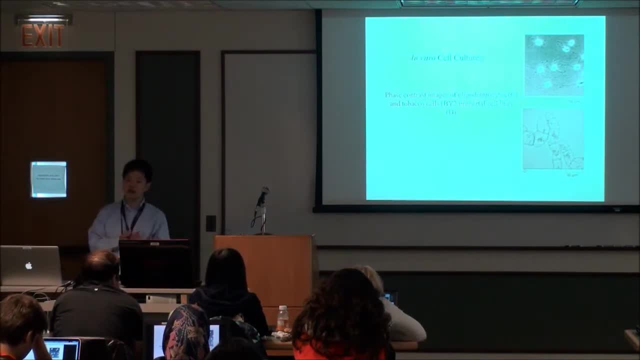 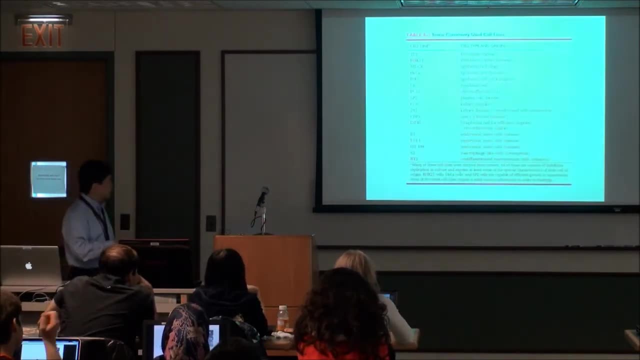 Okay. So with the cell isolation technology you can really separate different kinds and culture them and study. Okay, These are typical cell types you will encounter in the lab if you are working on cell cultures. So one is called 3T3 cells. 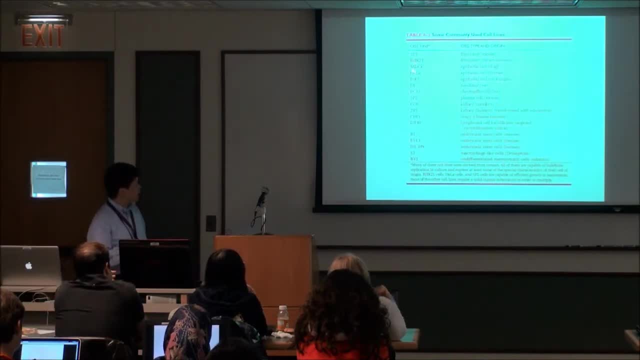 Basically these are fibroblasts. Okay, And I think MDCK is also very popular. These are from dog epithelial cells, Healer cell. if you are studying some cancer, you know research. this is also a cell type you will encounter a lot called epithelial cells. epithelial cell from human. 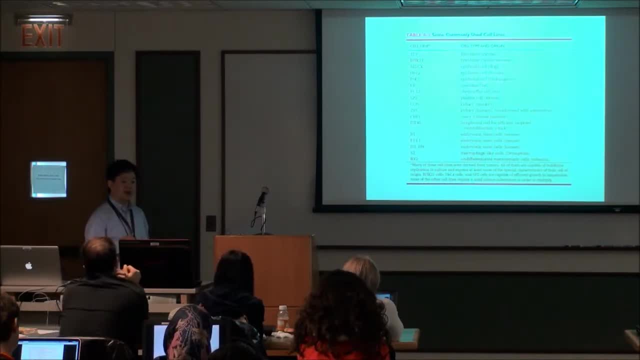 And recently people are more interested in stem cells And these are the typical ones, like R1, which you will encounter a lot if you are using the mouse embryonic stem cells, And H1, H9 will be the human embryonic stem cells. 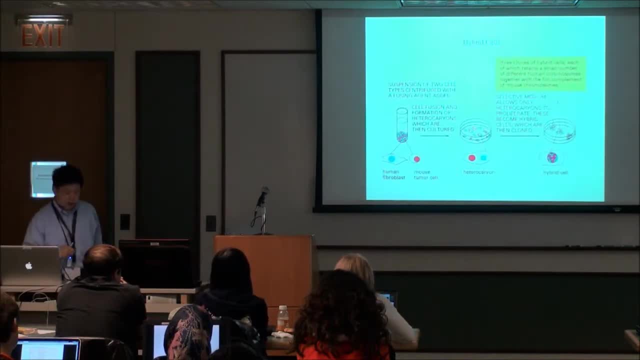 Okay. So these are regular cell types And there are another type called hybrid cells. Okay, Hybrid cell: basically, if you put two cells together, two kinds of cells together, and if you add some so-called fusion agent- okay, if you mix them together as a fusion agent- they will merge together to form so-called hetero. 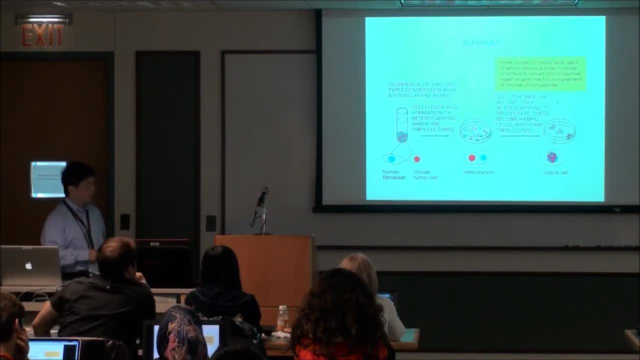 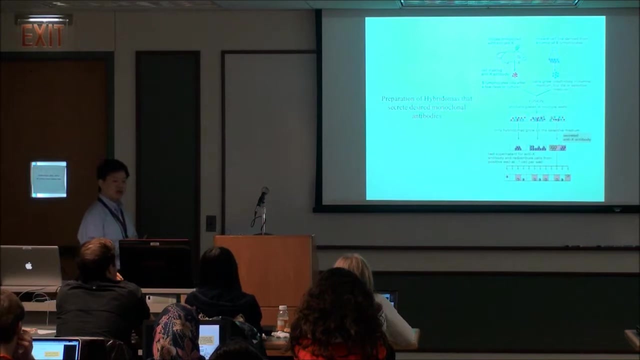 kaon. Okay, So these hetero kaon have two nucleus. Eventually they will integrate together to form so-called hybrid cells. Okay, So you might wonder you know what's the usage of these hybrid cells? Okay, Next slide I want to show you. it will provide very powerful tool for you to generate, for example, antibodies. 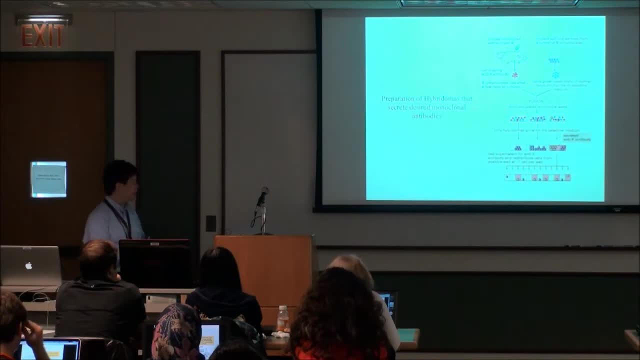 you know, continuously, without limitation. Okay. So, for example, if you want to generate antibody for a specific antigen X, for example, the typical way is you inject the antigen into an animal like a mouse and the mouse will have immune response, produce antibodies. Okay, And these are generated by B lymphocyte. But there's a problem: These B lymphocytes, they die quickly. Okay. Therefore, if you want to collect antibody, you have to do it quick and with limited quantities. And there's another kind lymphocyte which is collected from tumor: B lymphocyte. 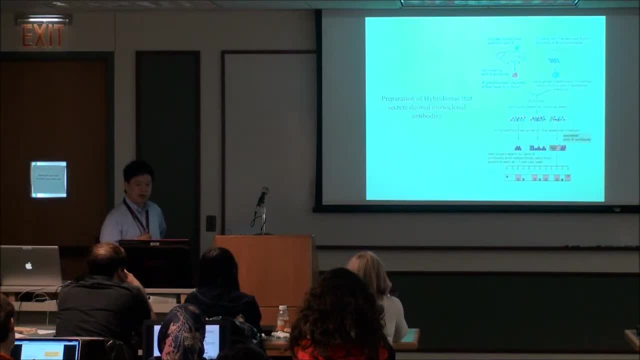 They can grow forever, But they don't secrete the antibody you want, right, But people can use the concept of hybrid cell to combine the benefit of both of them. So what you do is you put these- you know, B lymphocytes which can secrete antibody. 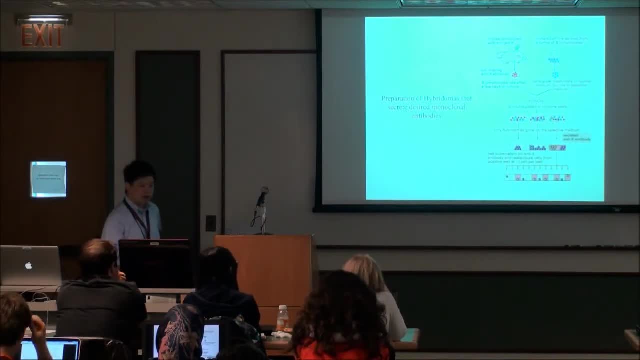 together with the tumor B lymphocyte, which can grow forever. You mix them together as a fusion reagent. Eventually, the tumor B lymphocyte and the B lymphocyte secreting antibody will be, you know, fused together to form hybrid cells. 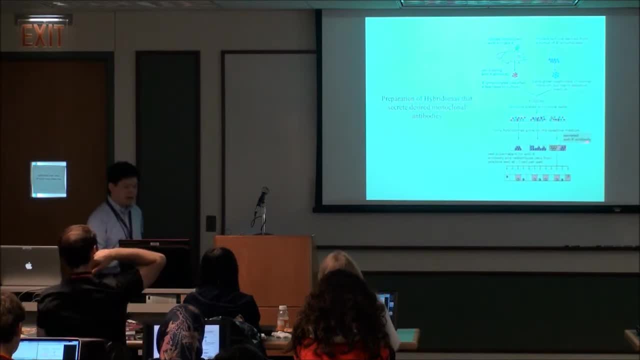 Okay, And then you can use selection medium. This selection medium, only the cell secreting the antibody will survive. Okay, After you culture a while and then split all these cells into you know small wells, Each will contain one cell. 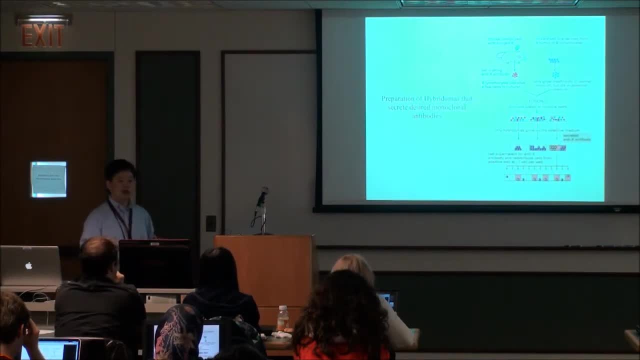 And you can use the selection medium to choose the hybrid cell which will secrete the antibody you want and will grow forever. Okay, So with this hybrid cell technology, you can do this. With this hybrid cell technology, you can collect these cells. 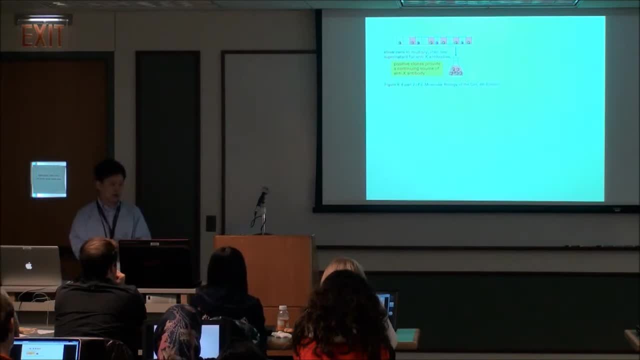 Okay, You can grow in the tanks or flasks. You can grow them, you know, all the time, And it will produce antibody. Okay, So you can bypass the problem that you can only collect limited amount of antibody in the animals. 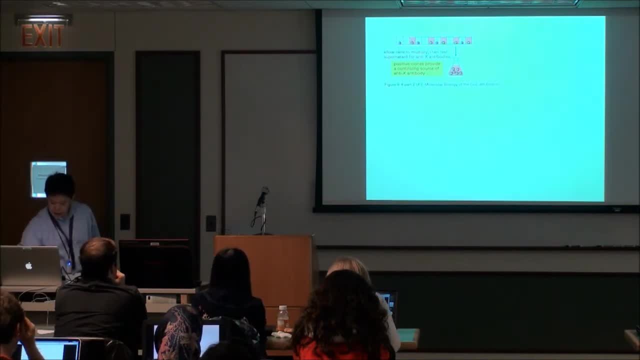 Okay, So this is the usage of hybrid cells. Now you have different kind of cells right isolated. How do you analyze the function of these cells, Or the protein function of these cells? For example, you want to know the protein profiles, whether they are phosphorylated in. 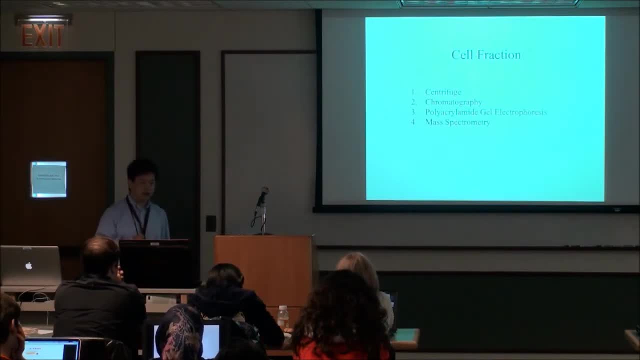 your tumor cells. How do you do that? Okay, The first thing you want to learn is you need to separate the cell component inside. Right, You have to break the cell, take out the cell content And because inside there are so many organelles, right, cytoskeleton nucleus, DNA, RNA proteins. 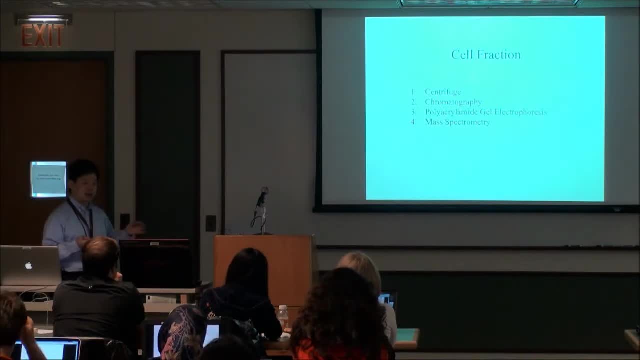 you need to separate them. Okay, To isolate the pure protein kinds for you to study. So this so-called cell fraction. you have to separate and sort them. These are the typical technology I'm going to, you know, encounter if we are working. 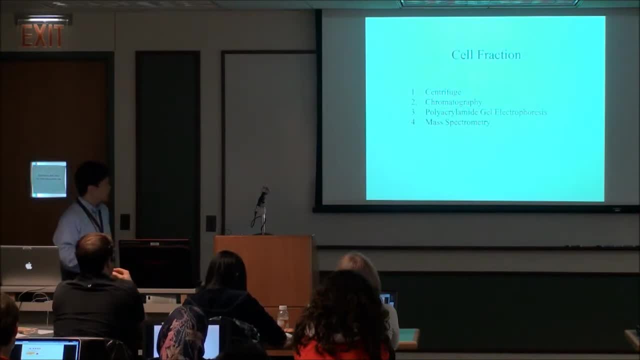 on the protein analysis from cells. Well, first is called a centrifuge- Okay, Very simple but very powerful. I'm going to introduce using a couple of slides. And the second is called chromatography- Okay, Which will provide pure resolution compared to the centrifuge. 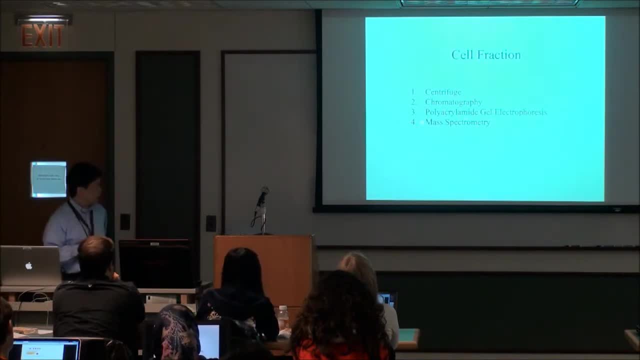 Okay, And third one, I will talk about polyacrylamide gel electrophoresis. And the last one will be the mass spectrum, which will really provide the identity of the protein you isolated. Okay, So first is the centrifuge. 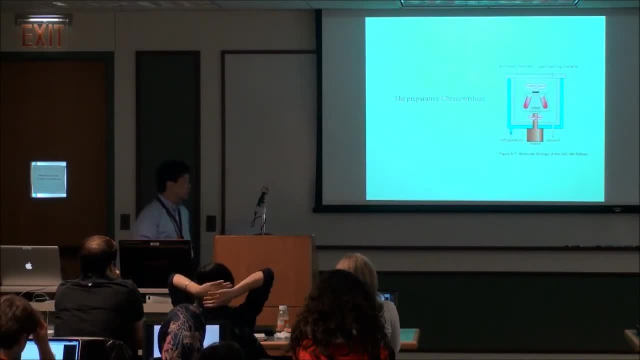 So when you are collecting proteins, this machine will be the one you will encounter in the lab a lot. It's called preparative ultracentrifuge, Okay, So it has a rotor And usually it will be in your refrigerator, Okay. 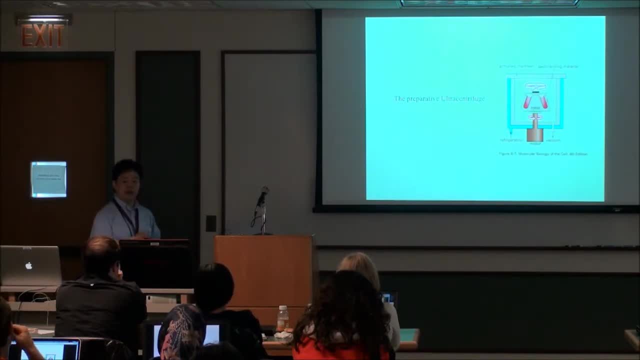 Because you want to maintain the low temperature so that the protein will not be denatured. Okay, And you also have a vacuum, to you know. keep this cover on top And rotors have to be tightly connected to the motor And it will generate a very high speed. 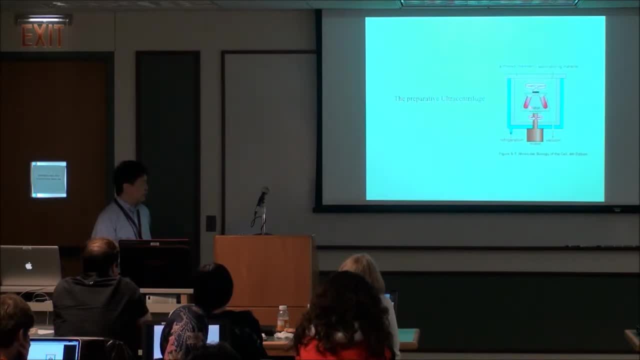 Okay, So this is a very simple technology. After centrifuge, different kinds of protein or organelles will be separated into different positions. Okay, And this actually is a very dangerous thing as well, although it's powerful because the speed is so high. you know 10 to, you know 10,000 or 20,000, you know RPM usually. 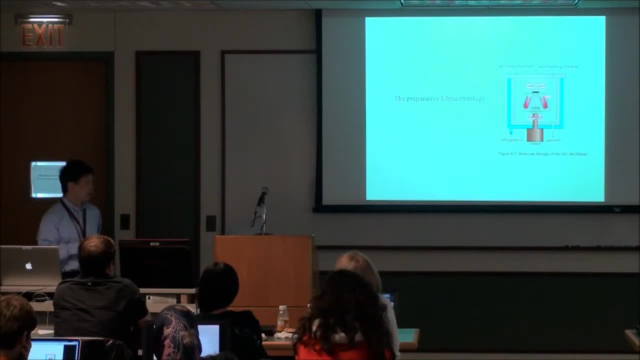 and generate a lot of force. If you're not careful, if the two tubes are not balanced, it will easily break the motor and rotor and actually fly out as well. When I was in San Diego we had an accident, you know, not in our lab, in neighboring labs. 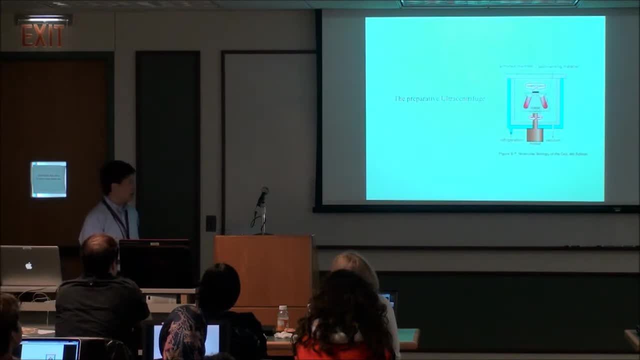 One day this rotor actually just fly out and hit the ceiling or the floor. You can imagine how much force it will generate. right, because the two small tubes are not balanced. Okay, So when you are using this, be extremely- you know- careful on that. 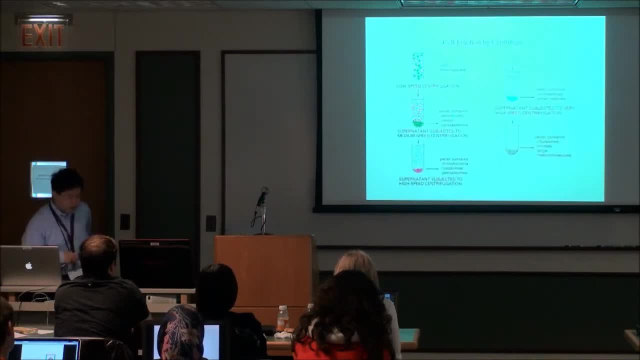 Okay, So with the centrifuge you can design different kinds of buffer and solutions to separate different components of the cells. Okay, So the first one is very simple: You can use a uniform buffer and use a low-speed centrifuge. Okay, 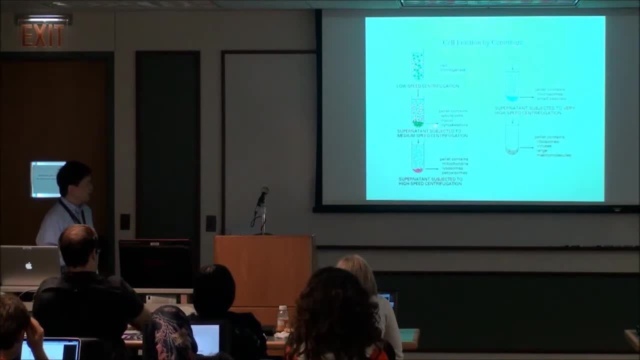 You kill the cell, put everything into the tube and low speed will already give you centrifuged pellet containing, like you know, nuclear or cytoskeleton. That's the first layer or the cell component you will collect. And if you further subject the supernatant into a higher-speed centrifuge, then you will 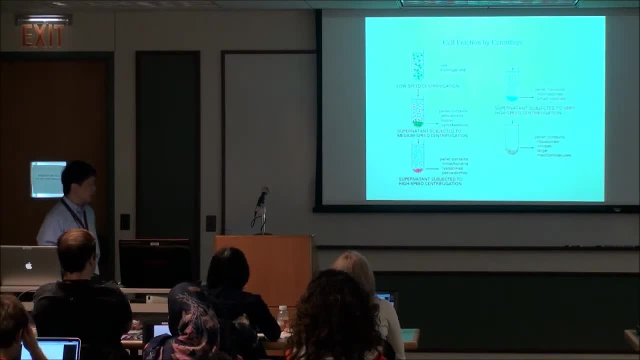 collect some organelles such as mitochondria linoleum, Which has mitochondria lysomes and parasomes, Okay, And then the supernatant can be further centrifuged. then you will collect some small like macrosomes. 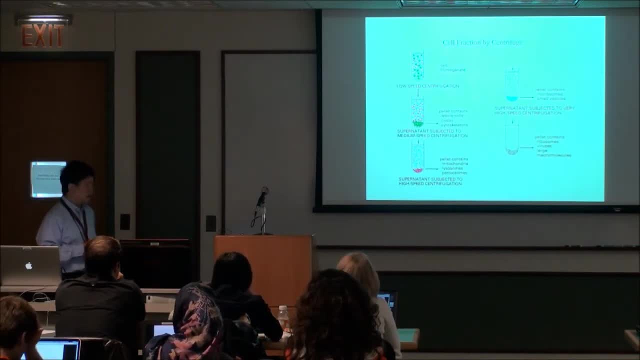 such as endosomes: Okay. These supernatants can be further centrifuged with a higher speed. then you will collect macromolecules such as ribosomes and virus- Okay, These supernatants still contain a lot of protein with different size. 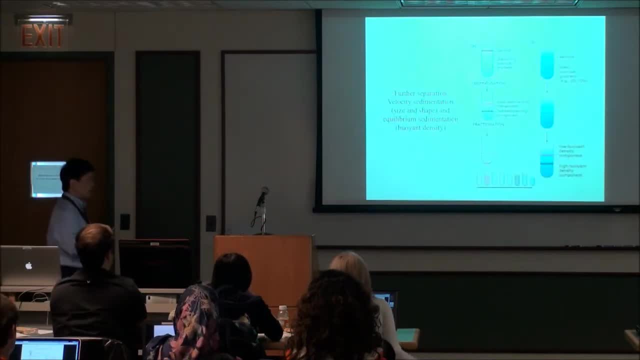 And then you can use another buffer called the gradient sucrose buffer. In this buffer you load these. now, these proteins are already relatively pure, right? There's no like cytoskeleton, no nucleus, right, And if you centrifuge using a relatively shallow sucrose gradient, you can separate these. 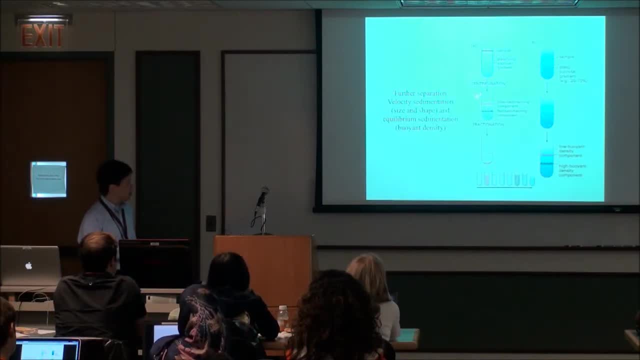 proteins in the mixture based on their size and shape. Okay, They will be separated into different positions And then you can punch a hole on the bottom and collect at different time. You can separate these two populations, Okay. Or you can subject these samples mixed with a relatively steep sucrose gradient. 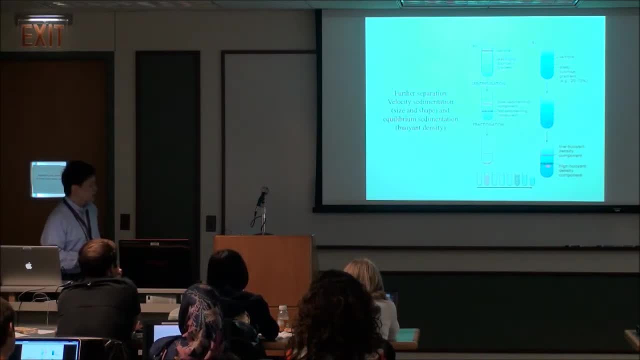 Okay, And do the centrifuge. These different populations will be separated based on their buoyant, you know, density. Okay, If different molecules have different buoyant density, they will be located in different positions. Again, you can do the same thing to punch a hole to separate these two proteins. 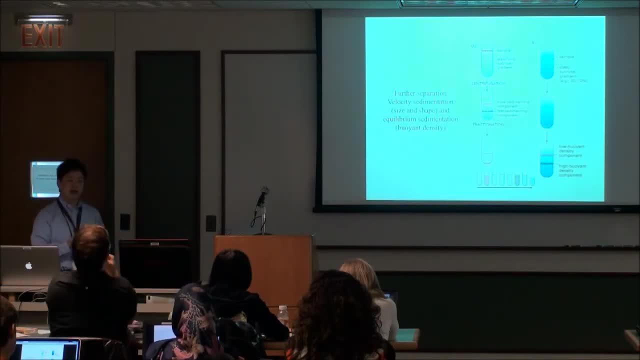 Okay, But still, as you can imagine, because there are million kinds of protein in the cell, these each layer will still contain multiple kinds of proteins. right, Then you can use other technology to further purify that. One is called chromatography. 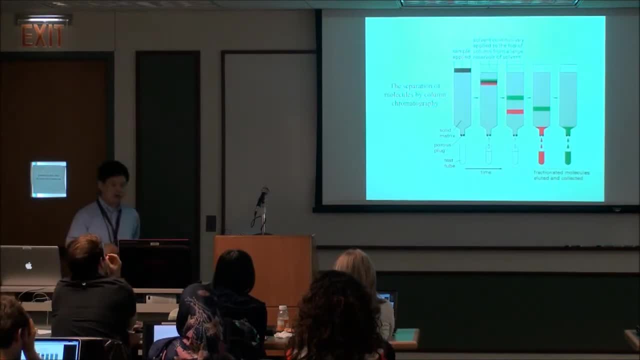 Okay For chromatography. it's also very simple technology. What you do is you have a column and then you load the sample on top. Okay, And this protein solution will be run through the column And because the size and charge of different proteins they're different when they pass. 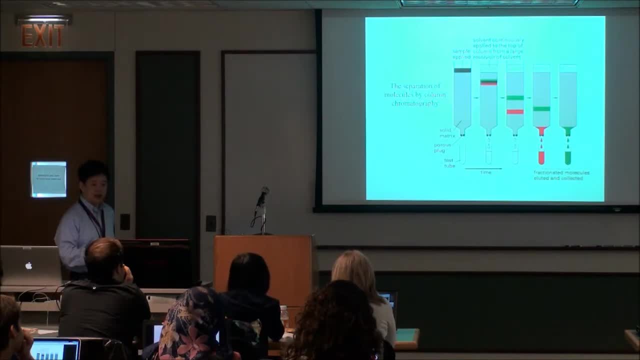 through this column. they will be separated, okay, based on their size or charge, And eventually you can collect them at different time and the different protein will be collected at different tubes. You separate them Right And for this chromatography there are typical three kinds. 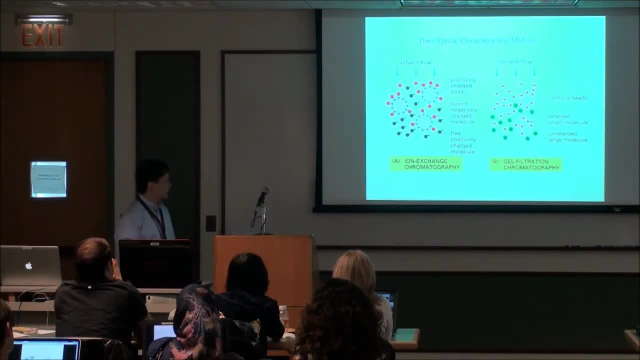 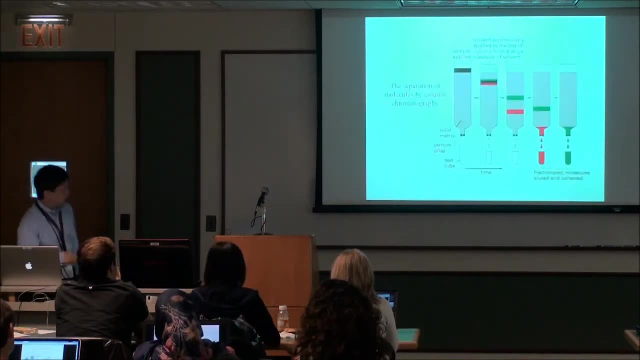 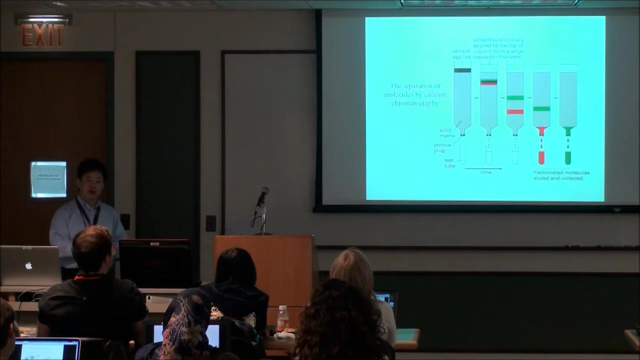 Okay, The first kind is called ion exchange chromatography And the concept is also very simple, As you can imagine this column, basically they are filled with beads, Okay, So you can change the beads' property to modify this chromatography. 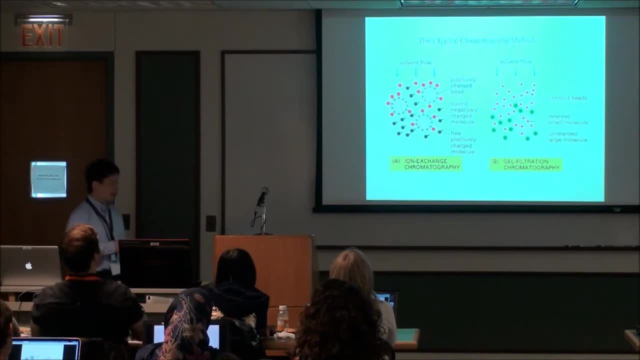 Okay, The first ion exchange chromatography is basically the beads are charged on the surface. Okay, If the beads are charged with positive charge, Okay, When you run through the protein mixture, all the protein with negative charge will be relatively sticky and absorb on the surface for a while, whereas all these protein with 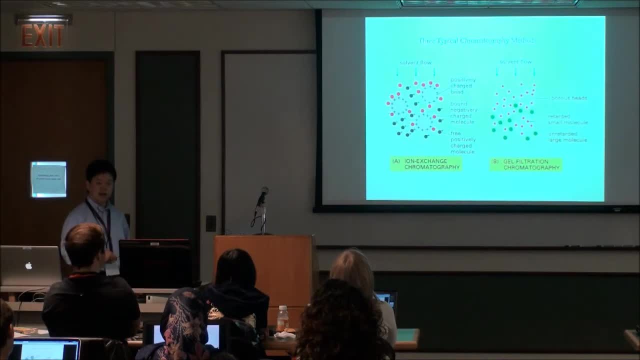 positive charge or non-charge will be run through quickly. Okay, Therefore you can separate the different kinds of proteins. Okay, This is ion exchange chromatography. Based on the charge, you can separate the proteins. Another one is called the gel filtration chromatography. 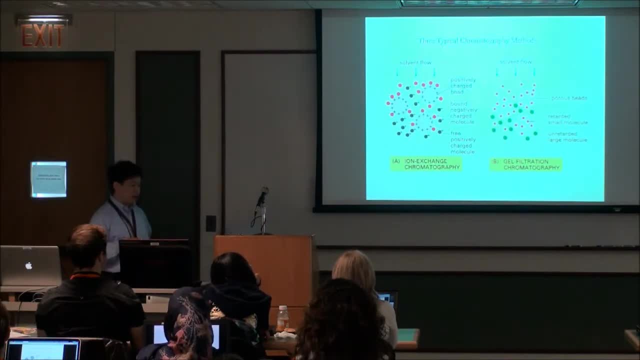 Okay, So in this gel filtration chromatography the beads are basically cracked, meaning they have some holes on the surface of beads. So when the protein runs through, some small protein will be trapped in these- you know holes a little bit and the larger protein will be run through quickly. 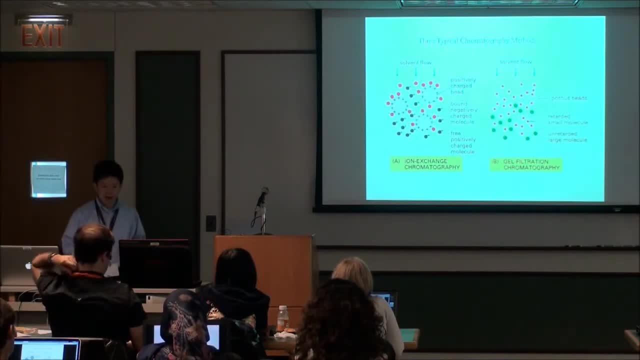 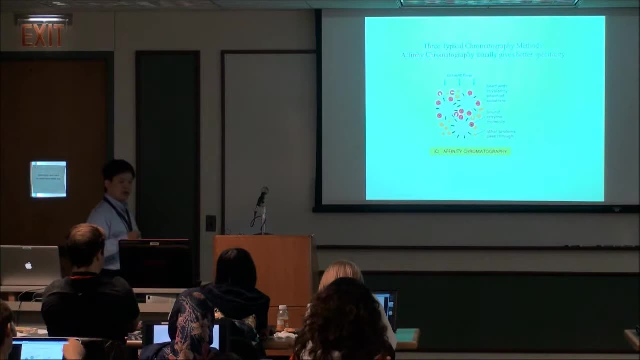 Okay, Therefore you can separate right based on their size. That's the gel filtration chromatography. And last one is more specific: All these you know holes on the beads. All these you know holes on the beads. or charge on the beads, still they will not. 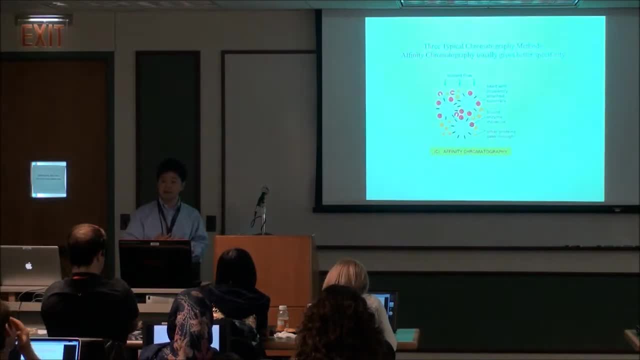 give you extremely pure purification right, because many protein will have negative charge. Okay, I mean many protein will have similar size, But this affinity chromatography will provide higher specificity. Basically, in this affinity chromatography, you have the beads which will be coated with. 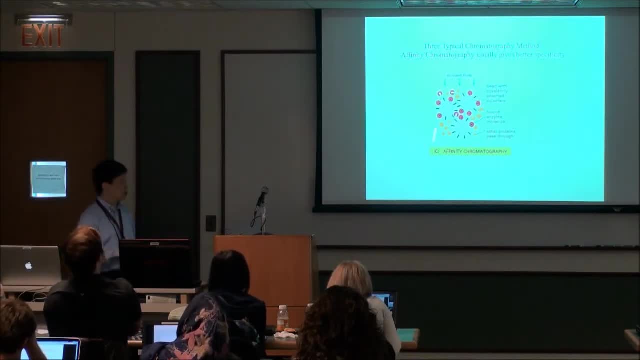 specific antibody. Okay, So when you run through the protein mixture, all the chromatography will be run through. Okay, So you can see here on the column the protein with specific receptors on surface. oh sorry, the specific recognition motif on the protein will be recognized by antibody and absorbed. 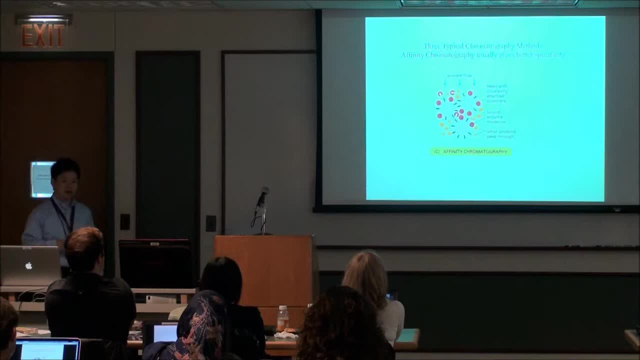 on the beads- Okay. All the other proteins will be run through faster, Okay. And then you can use high salt buffer to elute the protein absorbed on the beads at the last stage. Okay, So these are typical charts When you are doing chromatography. that's how you will encounter and collect the protein. 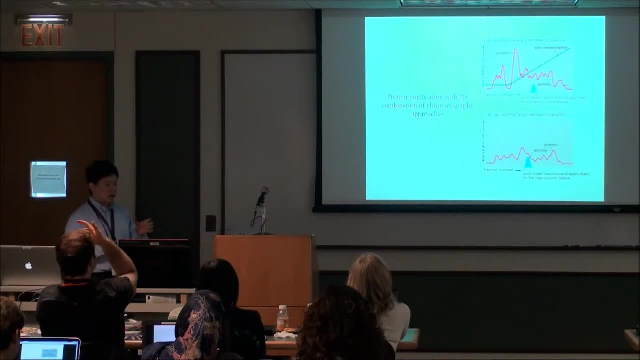 you want. So usually because the cell lysis, the protein mixture, are quite dirty, meaning there are too many kinds of proteins, Okay, And people usually combine these three kinds chromatography together to purify protein step by step. Okay, So first, usually people use ion exchange chromatography. 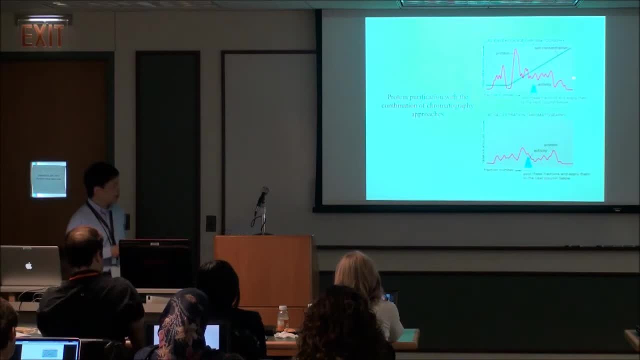 When you run the protein solution through this column, you can imagine. you know these different peaks represent the kinds of protein elute or pass through. Okay, So you can already see, based on charts, different protein will be eluted at different time. 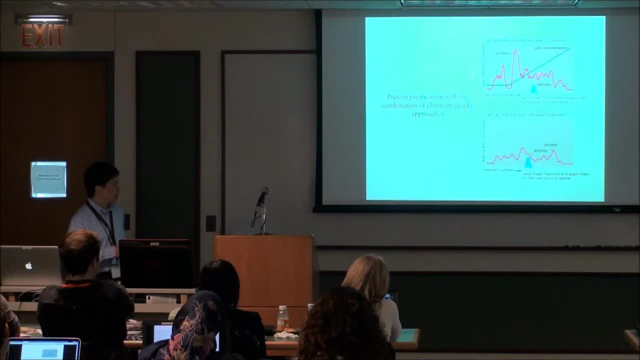 If you have some knowledge on your specific protein, you can collect, for example, this population which will contain your protein. you are interested? right And discard all the rest. Okay, So it's already with one step purification. However, as you can imagine, even in this peak, they will still contain a lot of different. 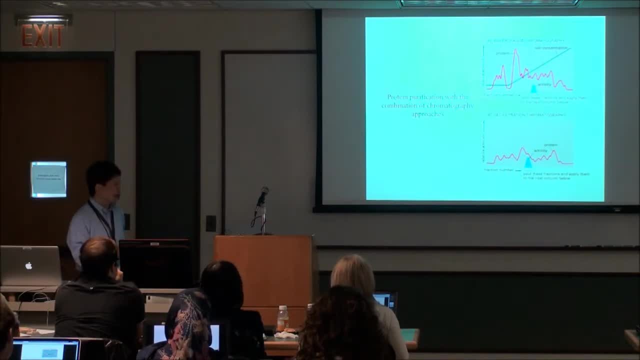 kinds of proteins with similar charge. Right, Because ion exchange chromatography will separate protein based on their charge. Okay, If different kinds of protein have similar charge, they will all encounter and group together in this same peak. Same peak, Is it clear? 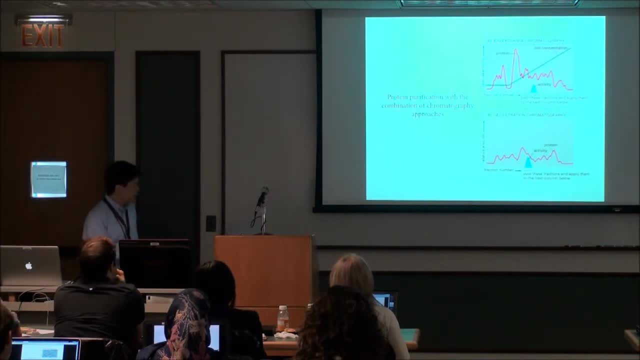 Then you can collect this peak and subject to gel filtration chromatography. Okay, For this one you will run through again and although all these protein will have similar charge, but they will have different size, right, And based on size you can further collect these. 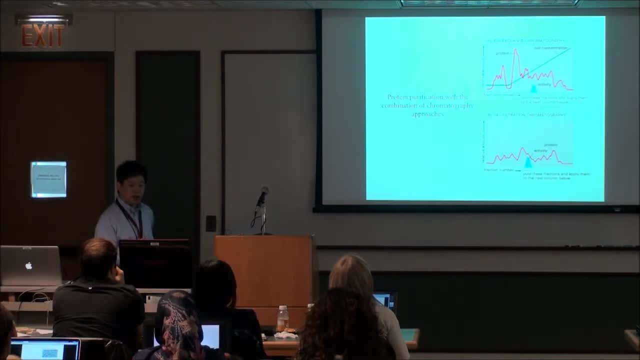 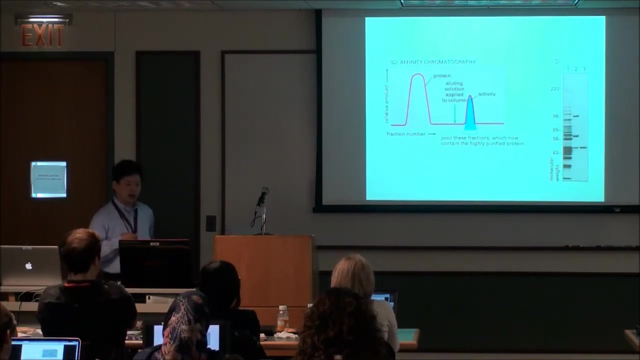 For example, this is a protein. you are interested. You know some knowledge about this protein. you are interested, right, So you collect this peak. Okay, Still, it will not be completely pure. Then you subject this protein solution into so-called affinity chromatography. 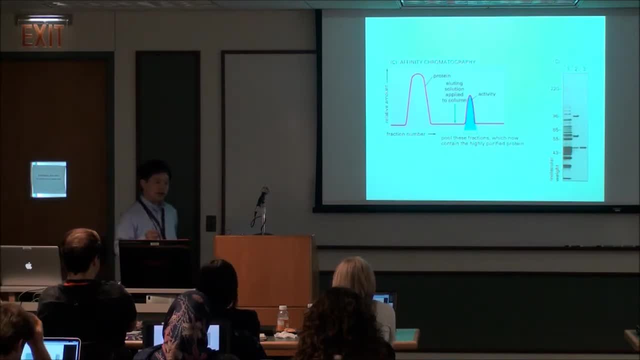 So, as you can imagine, usually for affinity chromatography usually you got two peaks right, Right. Why two peaks? Anybody can answer Okay. In the previous chromatography you see many peaks, right, Usually, But for this one usually you only see two peaks. 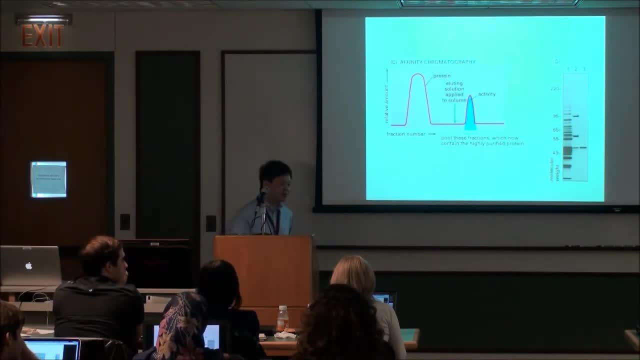 Say it louder, Maybe because of molecular weight of proteins? I think that's not the answer. I saw that other people said, yeah, you want to, Because it's very specific, so you only choose one protein, with the coated beads and the. 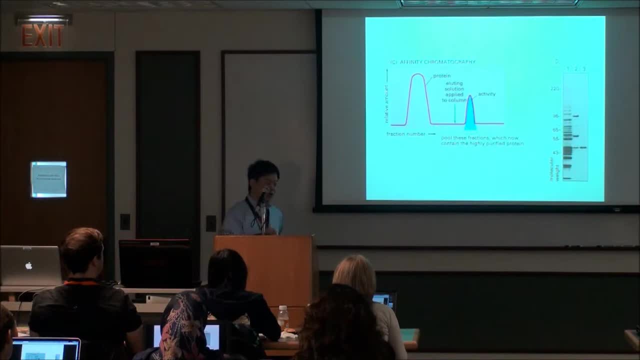 others. just Exactly, You have two kinds now. Either they bind with specific antibody or they don't. Because this there's no selection against the size, against charge, you know Everything else will be on the same peak. The ones with specific recurrent size will be bind to the antibody, right. 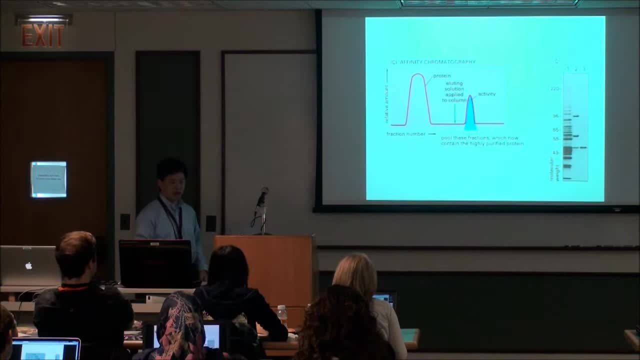 This will be eluted here, or the other will be another peak, Eluted faster, usually, Okay. So after this you have relatively high specificity Collective proteins. Okay, And this is the next step which I'm going to introduce, called electrophoresis. 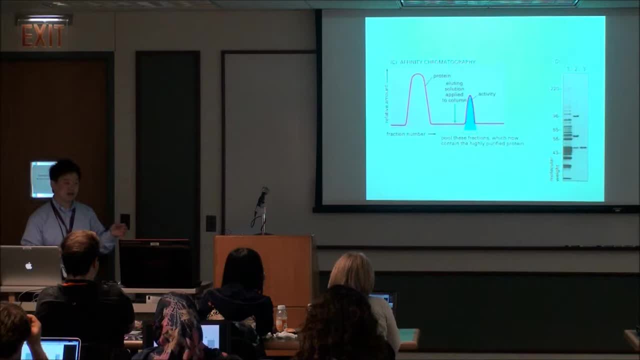 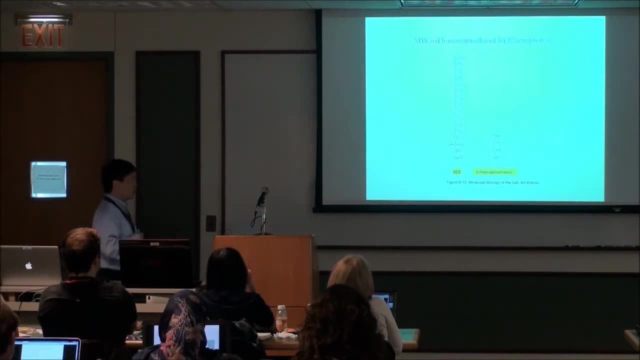 You can run into a gel and use antibody to identify the protein you purified. Okay, Before I introduce a page so-called polyacrylamide electrophoresis gel, I want to introduce these two chemical compounds which are essential for the electrophoresis. 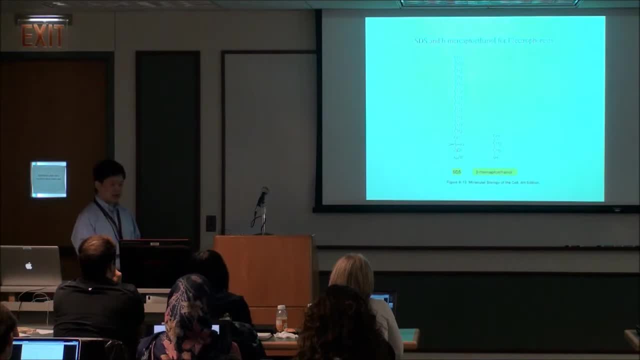 One is called beta-mecapital ethanol. Okay, So this beta-mecapital ethanol is essential because all the proteins, as soon as they collect from cell in the cell body, they usually have reduced environment, Meaning all the sulfate group on the protein. they will not form disulfa bond. 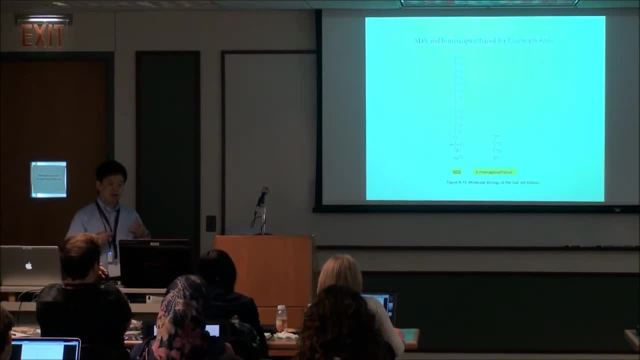 Okay, But as soon as you collect them from the cell body, they will be exposed to the oxygen right, So they will be oxidized form disulfa bond, And the beta-mecapital ethanol will be needed to add a solution to break this disulfa bond. 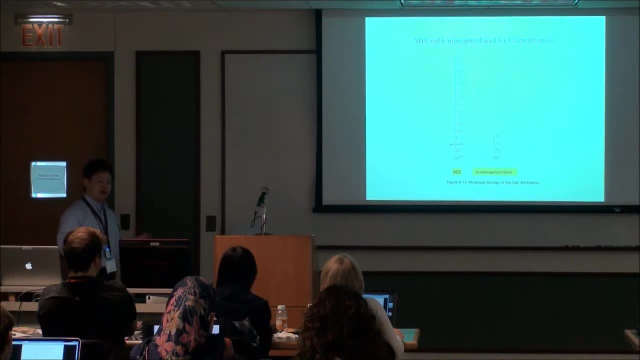 so that each intact protein will be separated. Otherwise, many proteins, as soon as they have this sulfate group, they will stick together. Okay, And another one is called SDS. SDS, they will basically bond to proteins and coat this protein with negative charge. 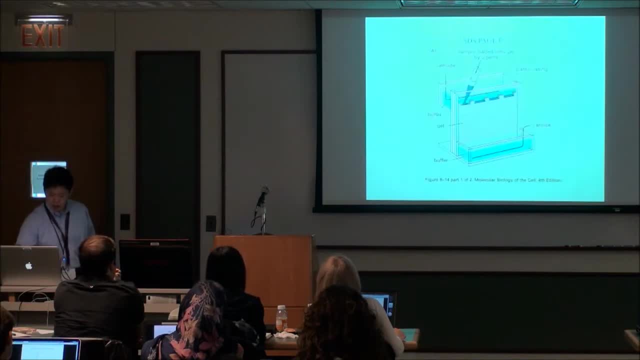 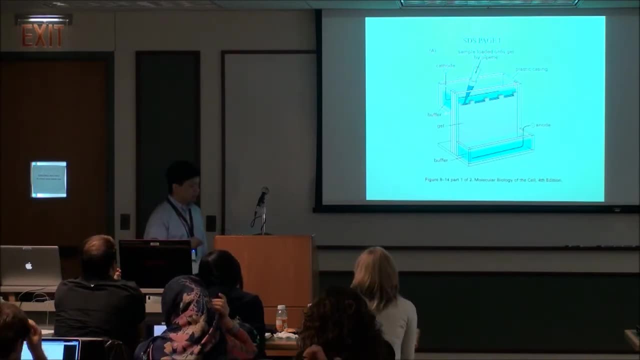 Okay, You will know why this coating will be important. So this is the electrophoresis system. As you can imagine, if you already add the beta-mecapital, ethanol and SDS, right, all the proteins will be break apart, right. 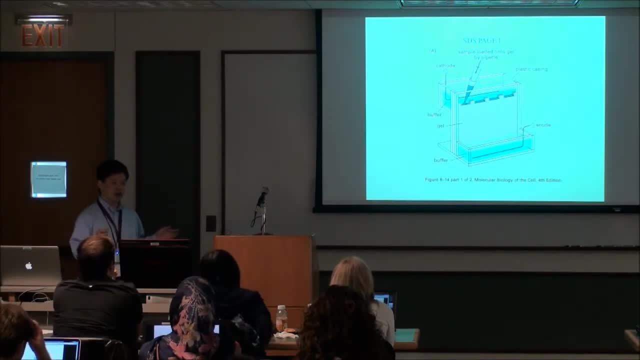 They will have intact proteins separated from each other, Okay, And they will be lightly coated with negative charge because of SDS, Okay. And then you. Now you load this protein onto a gel. Okay, There are different wells. You can load the protein on the gel. 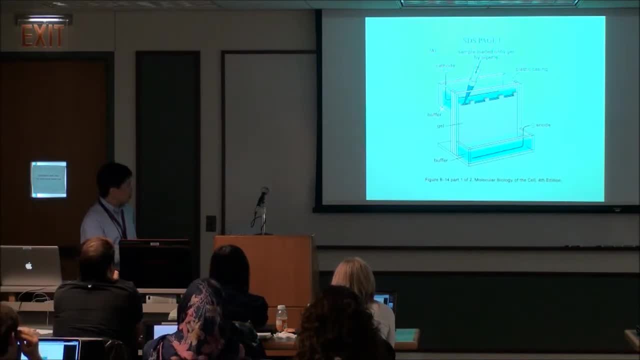 And these gels are connected on top by a cathode through a buffer. On the bottom connect to anode through a buffer. So if you load the protein on the top and run the electrophoresis, what will happen? The protein will go down right. 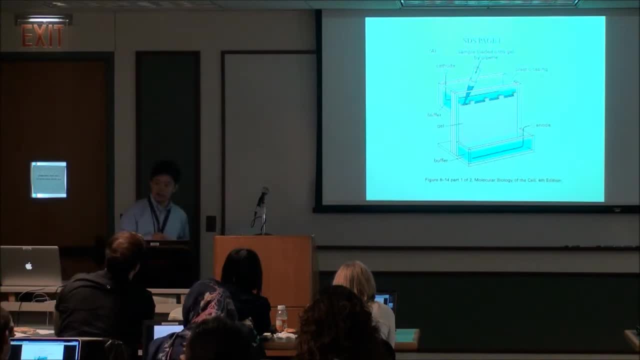 Why? Yeah, Because they are coated with SDS, So they are negative charged. right, They have to go to the positive charge side, So they will run through the gel, And these gels are essentially very tiny, small beads in the gel. 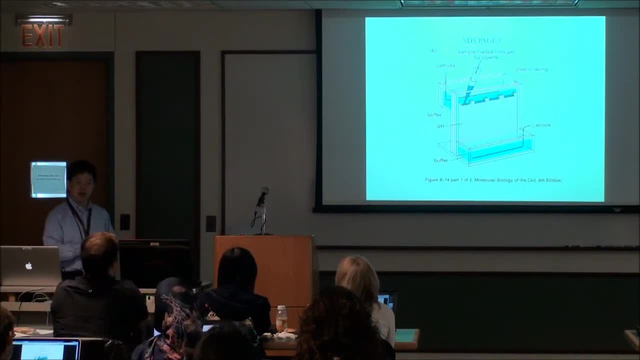 So you can imagine smaller protein will run slower or faster, Faster, right? So smaller protein with size will go faster And larger protein will stay and run slower. Okay, Therefore you can separate these proteins, Okay, So this is the principle of the electrophoresis. 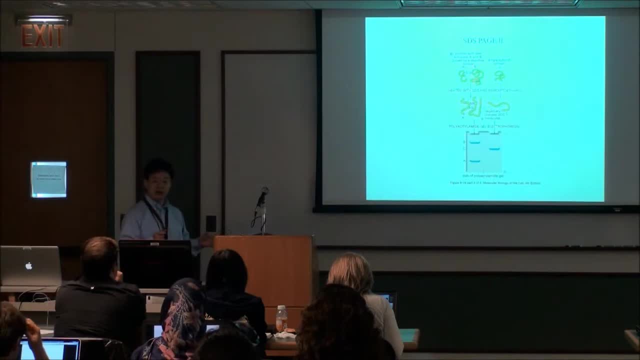 So this will basically tell you what will happen if you have two samples- Okay, Two groups of protein. One is light to pure- Okay, And one is, for example, formulate clusters because of the disulfide bond. But if you add the beta-ambicapylethanol, this disulfide will be break. 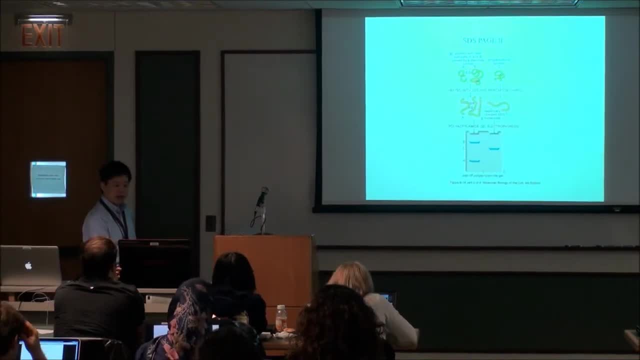 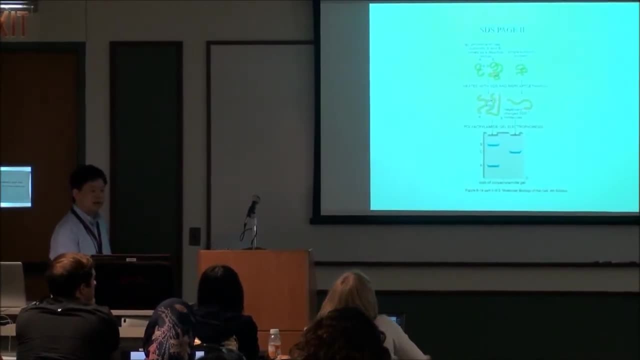 So the two protein will be separate proteins, right? And they will be further coated by SDS with negative charge. Okay, If you run through the gel, you will see this pattern. You will see these patterns, right. The smaller one will run faster. located here. 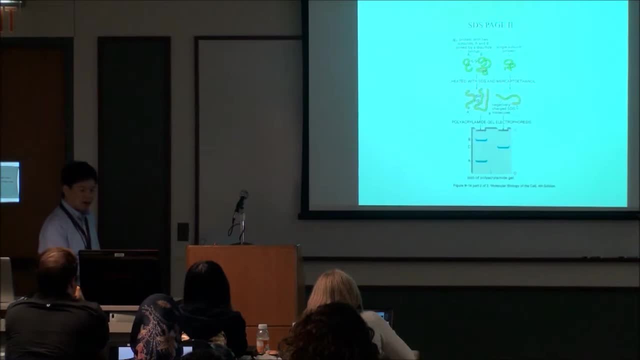 The bigger one will run. you know, slower on top, Okay. And for this one, because you have one protein, you can see one band, Okay. So these are typical. you know gel after you run the electrophoresis. 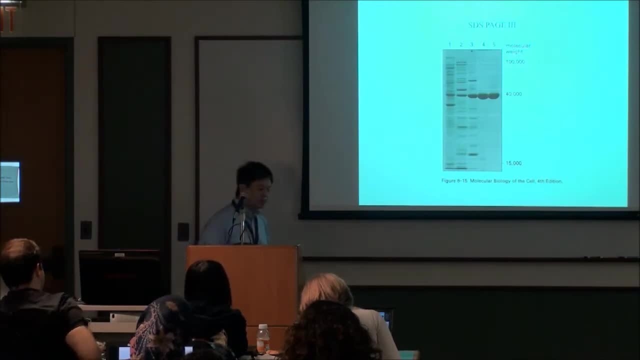 If you die to stain the protein. that's what you can see. Question: Why is it that some of these ones they don't use the recaptural ethanol but they get the same? Usually you have to, Or you can use other like DTT, you know. 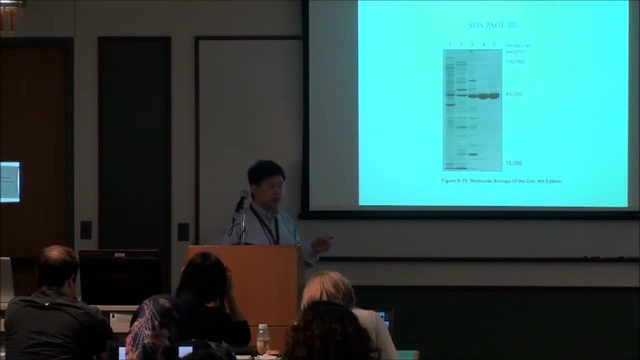 But you can use different reagent. The principle is to break the disulfide bond. If disulfide bond is not break, a lot of protein will cross together. Because I ran a gel with and without the recaptural ethanol, it doesn't get the same result. You have to use other reagent which will also break disulfide bond. Otherwise they will not in general, Because all the protein will be oxidized And they will ligate together through the disulfide bond, So the protein size will be changed. 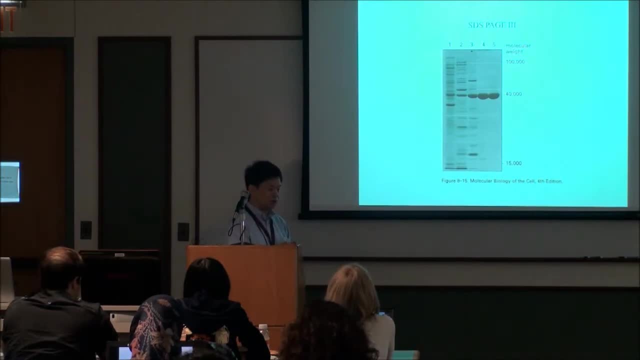 Supposedly you should see different patterns. Yeah, Unless they have specific. you know these proteins have no disulfide group on the surface. Then you will see the same. you know pattern. Okay, Any other questions on this? 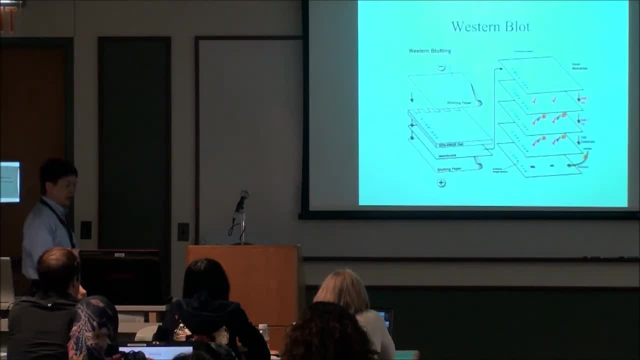 Okay, So now you have the gel right And you already have separated protein on these gels. But you can imagine these electrophoreses still. the basic principle is based on size, right? There are still a lot of protein which will have same, similar size. 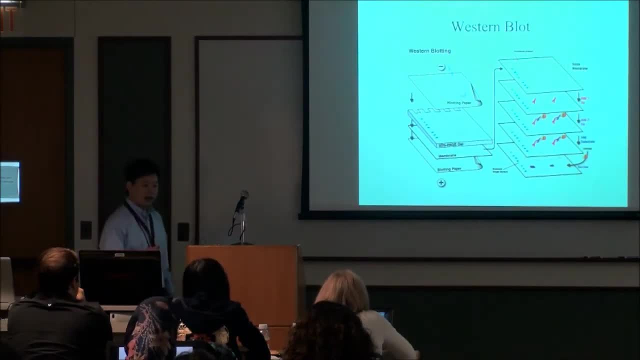 So they will be located in the same spot, And then another technology called Western can further help you to identify the protein you are interested. Basically, the principle is: you assemble a sandwich So you have a gel in the middle, Put a very tight membrane on the bottom. 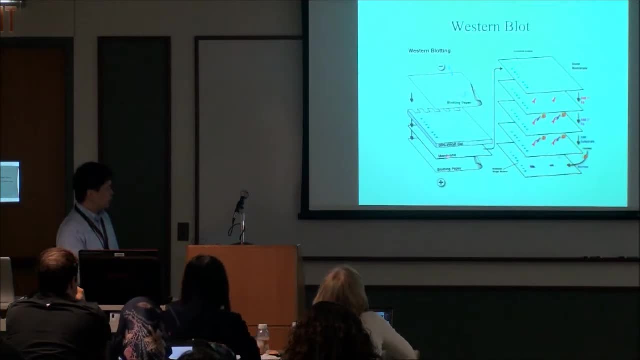 And a filter paper on the two sides. Okay, Then you apply an electrophore on top of the negative. On the bottom is positive, right? So you can imagine the protein will be transferred to the membrane, right? Why Exactly? 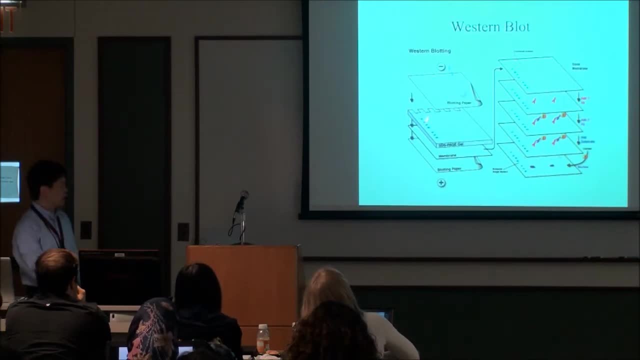 Because they are again negative charge, right. Whenever you apply an electrophore, it will go down and stick to the membrane, Right? So this is actually an important step. you know, You have to make sure your membrane is put in the right side. 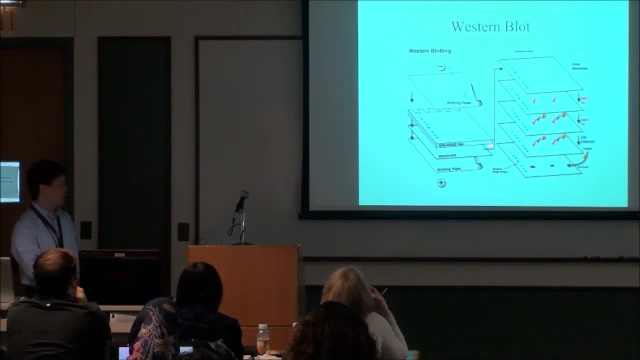 Many times we are doing experiments, right As assembling a sandwich. if your membrane is put on the positive side, then all the protein will get into the tank. you know It will be lost. Okay, This actually happened. you know, to me too. 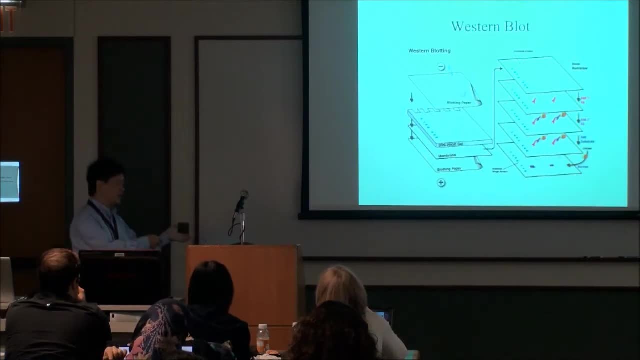 When I was first doing Western blood, you know, Because at that time, if you are not so careful, you are not sure which side is the protein, And easily the protein will be just run through. Okay, Now, after you have protein, stick to the membrane. 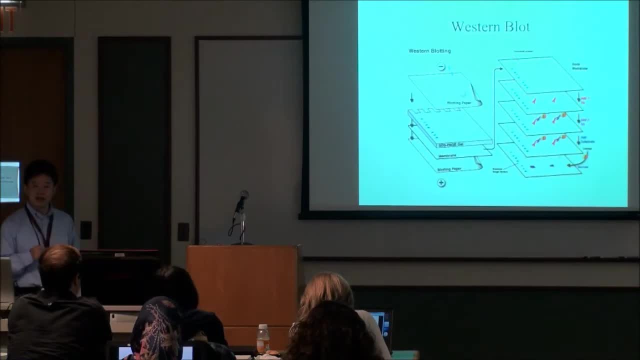 you can do further. you know standings to identify protein. you are particularly interested. So if you have membrane, take out, then you can apply so-called primary antibody, first antibody which will specifically recognize protein. you are interested, Okay, So the protein band will be identified. 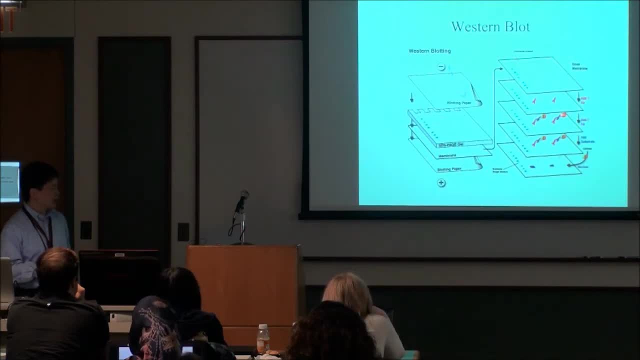 And then you can further add the secondary antibody, contain some enzymes And then add some chemoluminescence substance which will be modified by enzyme to emit luminescence. Okay, Therefore, you can subject this gel to a detection machine. You can see the color of the luminescence. 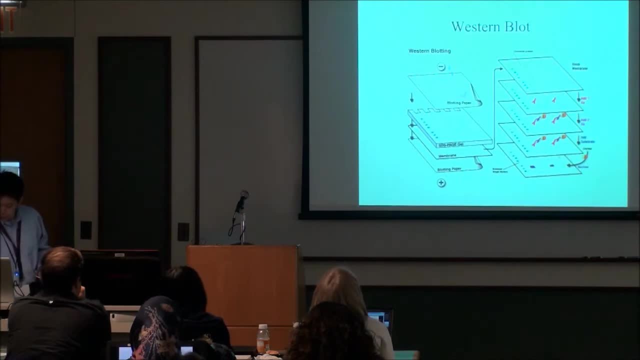 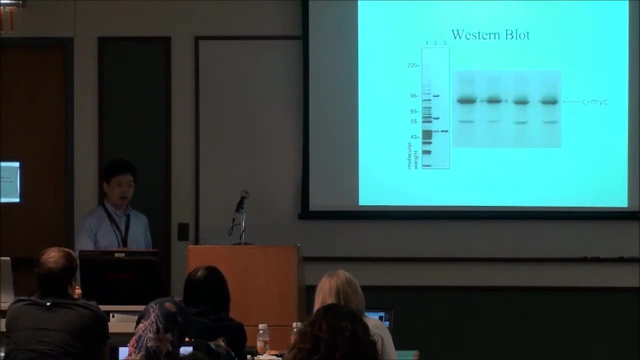 Okay, And therefore you know the location of the proteins. So these are typical. you know Western blood gel: Okay, You already incubate the membrane with specific antibody, for example CMYK, And you can identify the specific proteins already isolated. 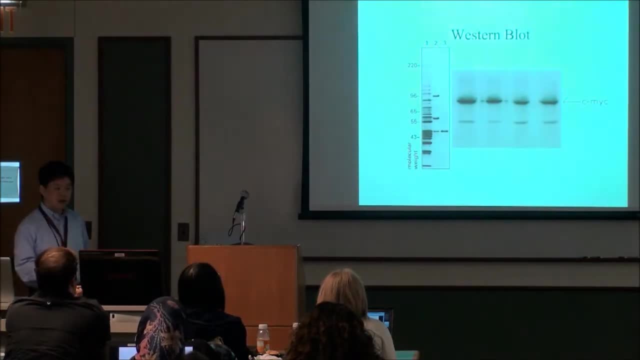 Okay, As you can see, there are also some minor bands. This is, you know, also quite common in the laboratory, because you know all the antibody will be that specific, Only recognize the specific protein. There are some similar motif for protein with different size. 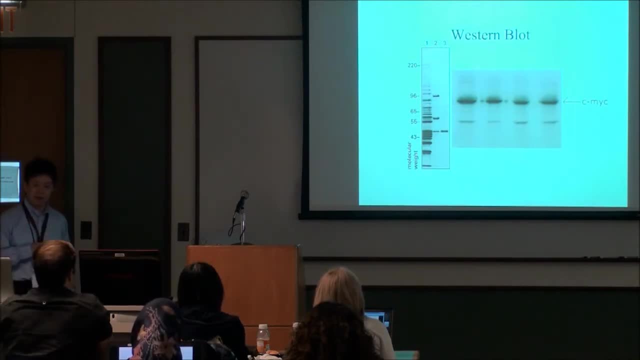 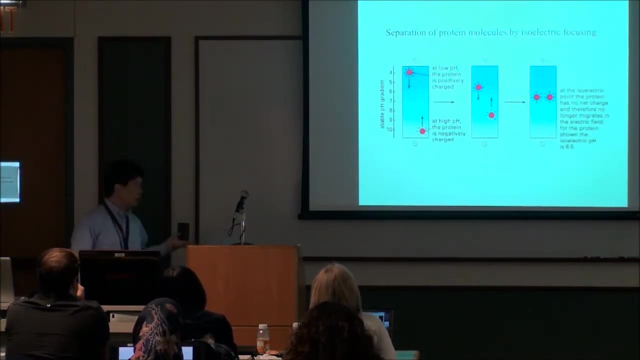 They will also be picked up by the antibody. Okay, So we are talking about the electrophoresis based on size. There are another one which you can also utilize, called isoelectric focusing, So the principle is also very simple. If you can create a gradient of pH in the gel, 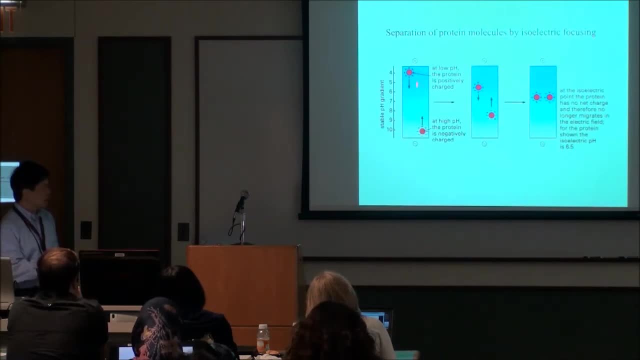 okay When the same protein is loaded in the gel. you can imagine, at a low pH it will be mainly, you know, positively charged, Right, If it's at high pH, it will be negatively charged If you apply electrophoresis. 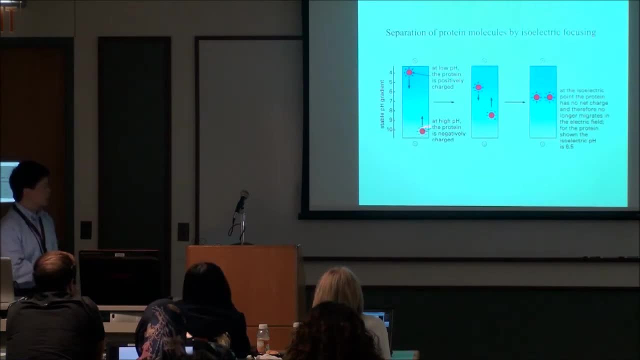 negative on the bottom, positive on the top. these proteins will start to migrate until they reach a point where they have relative equilibrium of electricity. Okay, So based on this concept, you can also separate proteins based on their charge, Right? So if you can combine this isoelectric focusing, 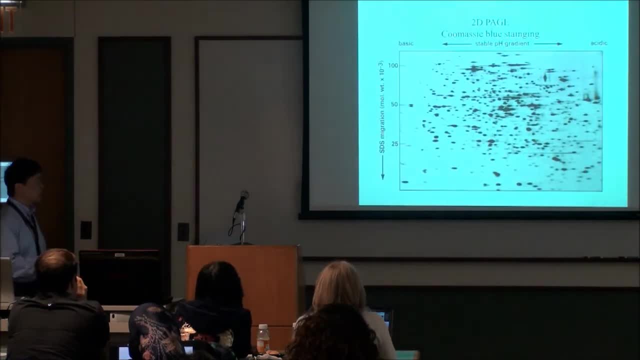 and SDS page. then you can have so-called 2D page separation. Okay, You can use isoelectric separation based on their charge to separate all these X-axis. Then you further run SDS page on the Y-axis. All the protein will be separated. 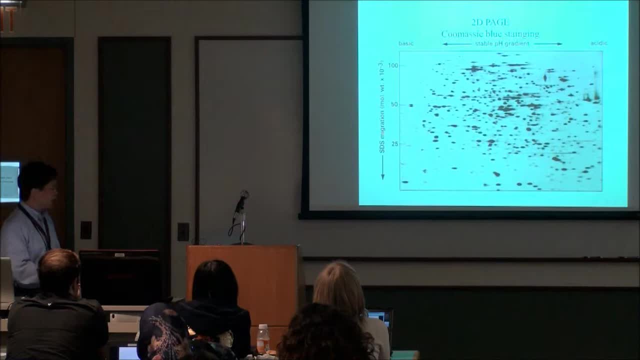 on each single dot in general. Okay, As you can imagine, if you only use 1D SDS page, then all these proteins with similar size will be, you know, located on the one spot, Right If you add another 2D isoelectric separation. 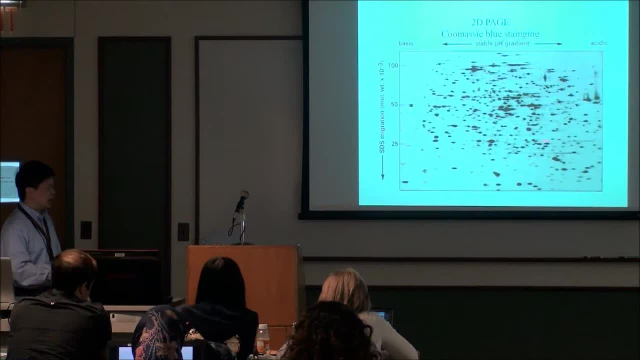 then they will be separated into different spots, Although they have different size, but their charge are different, And they will be separated along this isoelectric gradient. Okay, So then, if you have this 2D gel, you can further use the antibody. 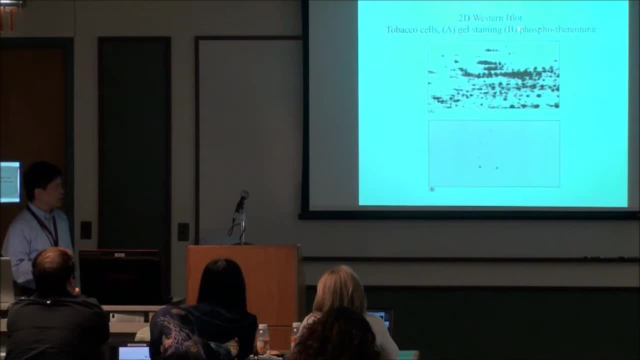 using like combined with the Western, for example, phospho-serine antibody can further pick up these dots, You know. so you can, in this gel, after you add the phospho-serine antibody, you will pick up these couple dots. 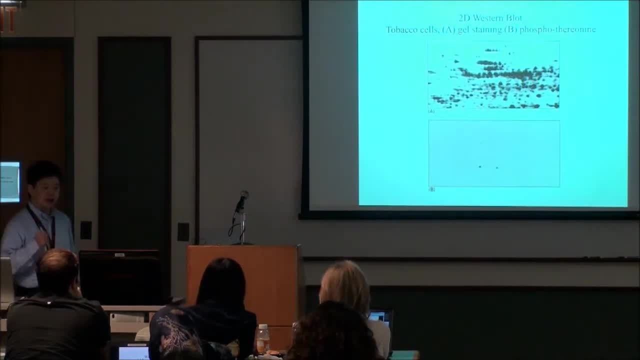 So these dots represent proteins which are serine phosphorated, Right. So this will be a very powerful technology for you if you want to study, for example, some cancer cells. Right, You isolate the proteins and you add this antibody Cancer cell versus normal cell. 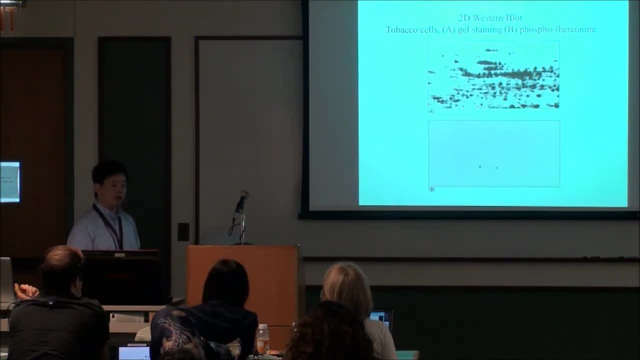 you can really see how different the proteins are. serine phosphorated: Okay, But at this point you still don't know. although there are multiple spots, you still don't know what they are. what proteins are serine phosphorated? 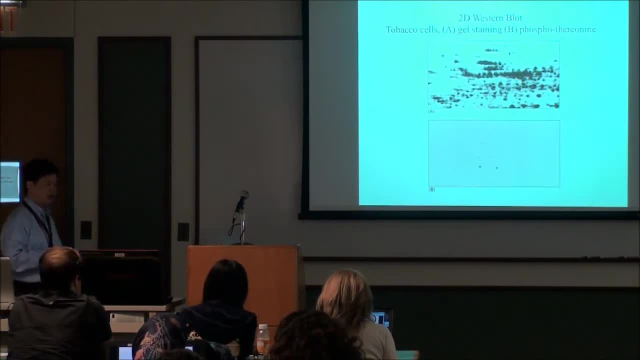 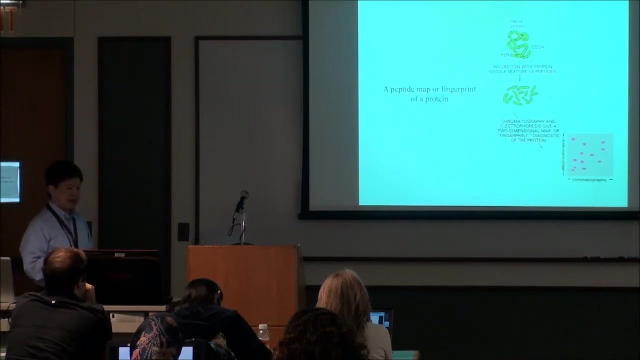 Okay, And next couple slides, I will introduce techniques which will help you to identify each dot, what the specific protein you are detecting. Okay, So the principle is basically very simple: Use an enzyme protease to digest and cut. 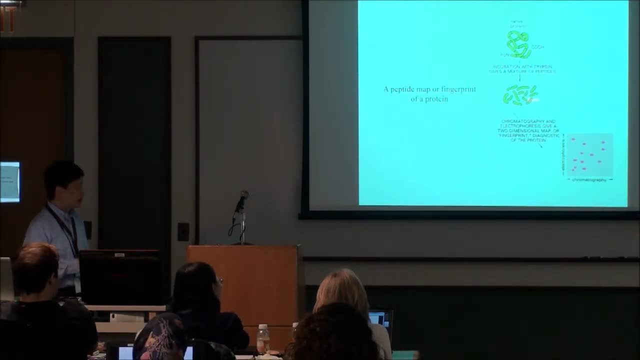 the protein into multiple pieces. Okay, So they become a group of peptides And then if you run a 2D gel, you will see these profiles in 2D Right, As you can imagine if you use the same enzyme. 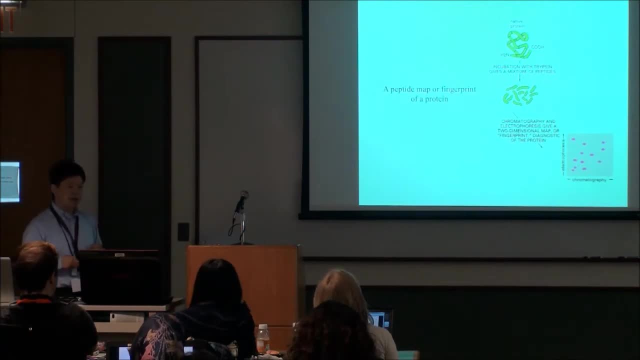 to cut the different proteins and run this 2D gel. different protein will have different features, Right? If they have the same pattern, likely they are the same proteins. Is it clear about this concept? Okay, So if you have a library, 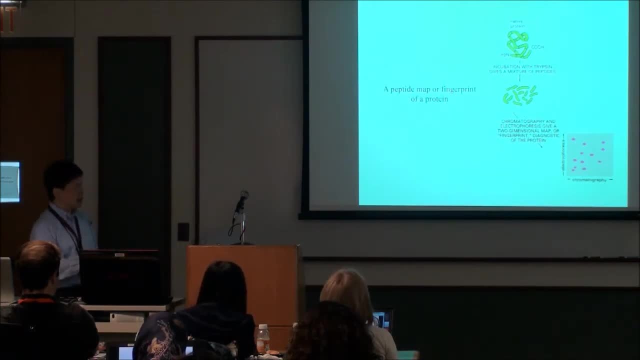 of the protein profiles already there. you can get these unknown dots of protein, isolate them, digest them and run the 2D gel If you get a pattern of these peptides and subject to the library and match to the library of known proteins. 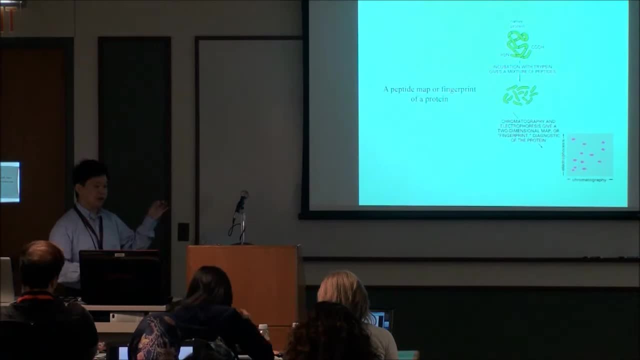 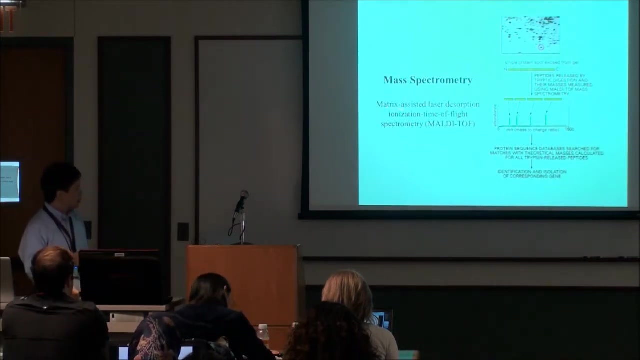 you know which protein you already isolate? Right With 3-inning fast ration, Is it clear? Okay, And another technology then is basically a similar concept. It's called mass spectrum. It's a matrix-assistant laser desorption isolation time. 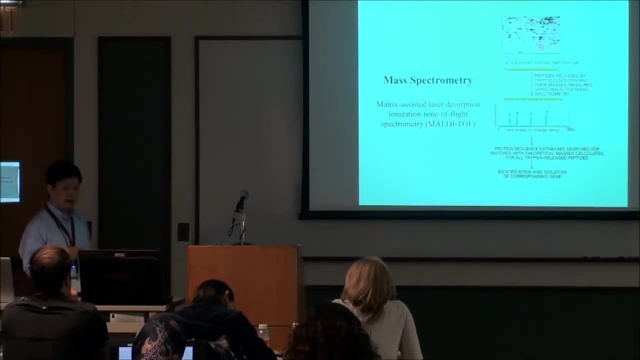 of flight spectrum match. Okay, People just call it MODYTOF. Basically, as I mentioned, if this panel you already use antibody to identify or phosphoantibody and this dot, you want to know which protein it is. 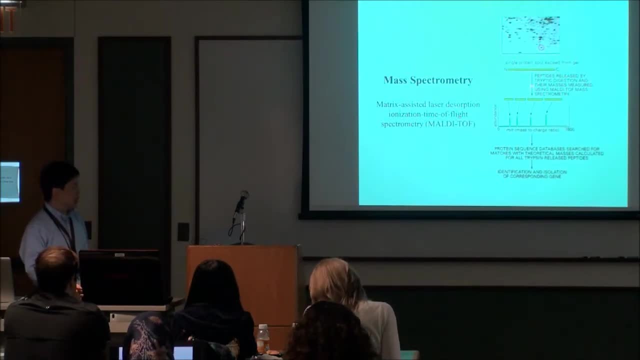 You isolate this dot and purify the protein and digest with enzyme and then run the you know spectrum And these are peaks of peptide right with different molecular weight, And there's already a library available for you. You can match this pattern. 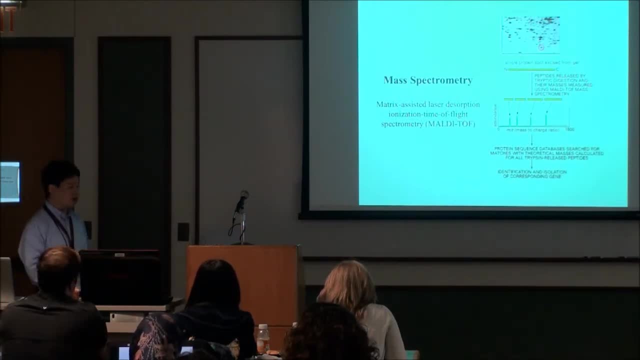 to the library And if you match a protein, known protein, you already know which protein you are looking at. Okay, So so far we already talked about you can isolate cells, right, You can collect a protein. You can subtract. 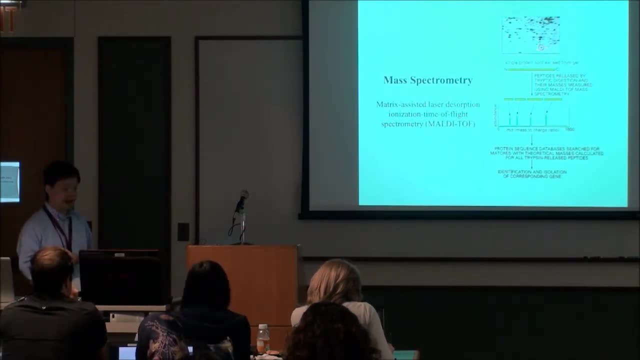 and separate all the proteins And eventually you can select protein which is specifically modified and then use mass spectrum to identify which protein it is. Okay. Therefore, you can really study what kind of microenvironment or stimulation can modify the cells. Okay. 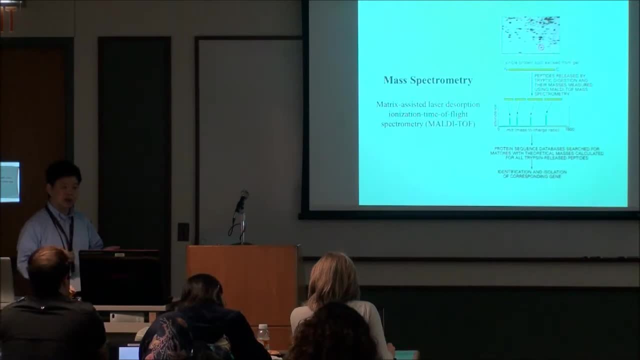 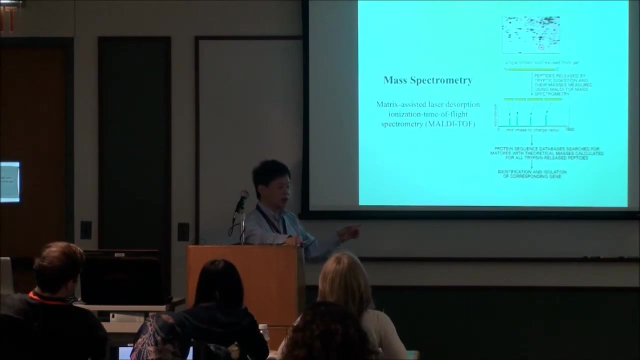 Modify all specific proteins? Okay, Right, Based on this technology. Is it clear? Okay, Yes, So, for example, all the proteins right people have. for example, if a known protein right, you can generate like: 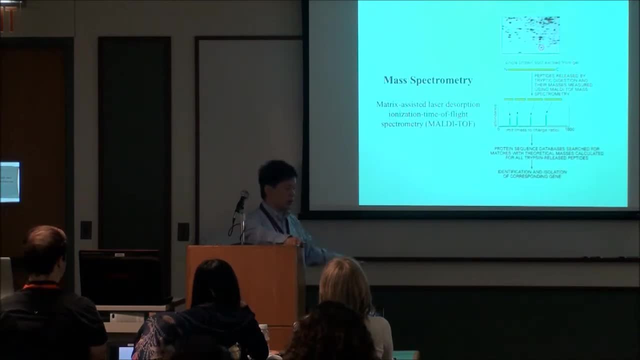 you know the gene sequence I already know In the next couple slides. you can amplify all these known proteins And then each protein you can subtract to this mass spectrum. They will generate their own unique feature. right, Each different protein. 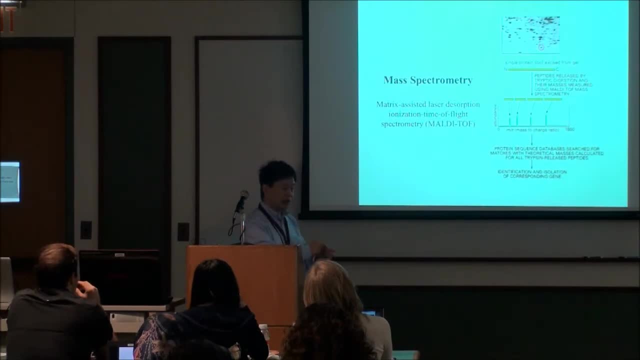 they will have different features Because the amino acids are all different. right? If you use the same enzyme to digest, they will give you a unique pattern. Is it clear For all the known proteins? Okay, So you would go to a certain website. 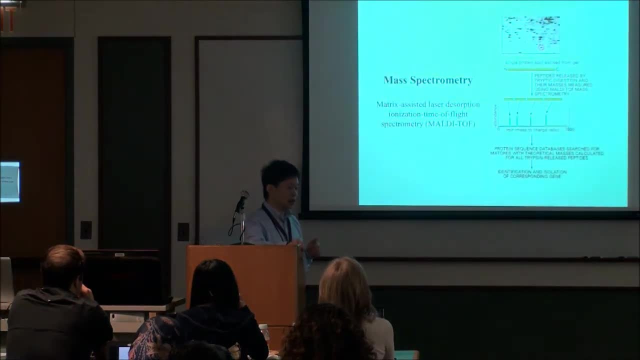 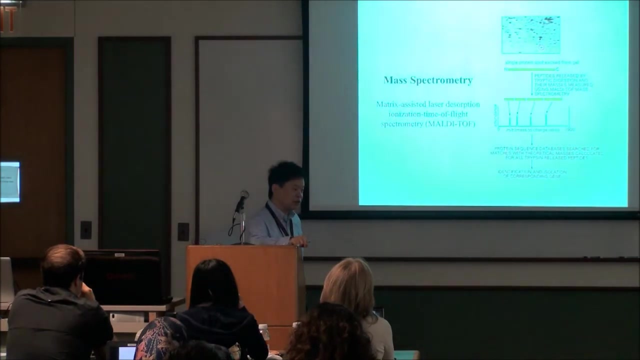 Yes, Yes, exactly, NHBI, they will provide this Right. So this is the library already known existing right. And then in your own experiment, for example, you are interested in certain stimulation, for example serum stimulate. 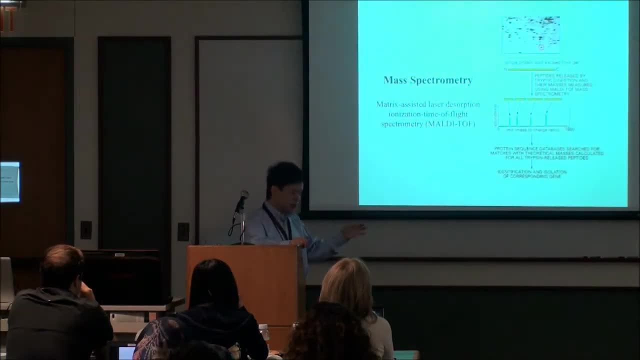 you know certain protein modifications And you isolate protein. right, You grow this, isolate protein and run through the gels And you identify there's this dot which is particularly phosphorylated. right, And you don't know which protein it is. 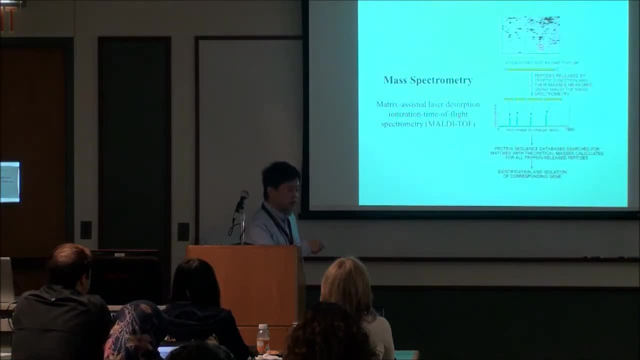 right. You purify the protein, digest them, subtract this mass spectrum, you got a profile And then you run this profile to match the known library or the proteins. If they match, then you will know which protein it is, Because 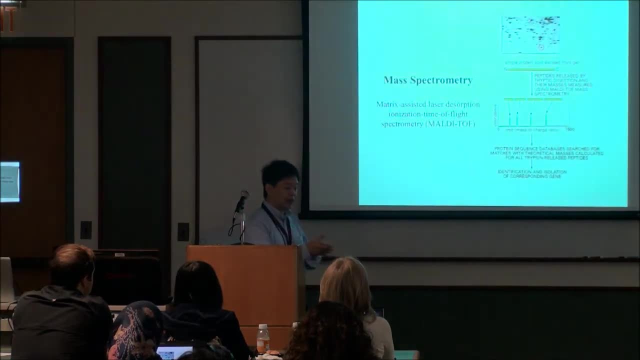 based on the match, you can find out which protein identity is in the library. Is it clear to you already? Yeah, it's just that I'm worried that, um, you know, mistakes do happen. and what if you probably did not run? 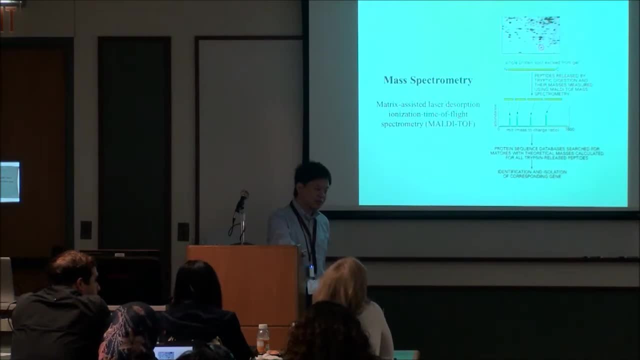 your gel long enough to get the correct spot size, the correct spot size, Then you happen to mismatch. Uh, you know, you don't care whether you run correctly in this case, Because in this case you are particularly interested whether certain 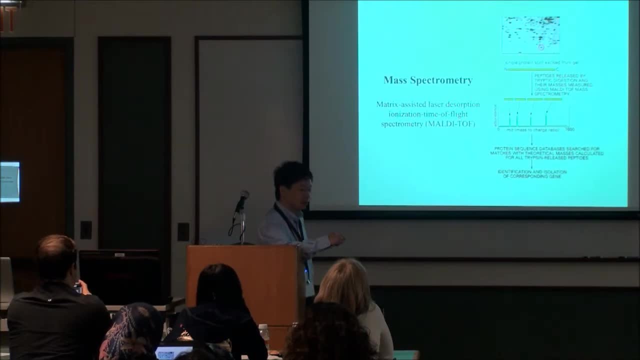 proteins are phosphorylated and you want to know what identity it is. You just pick up this, any point which you are interested. you know it's phosphorylated, for example. right, Just pick any point and run through the match spectrum and match. 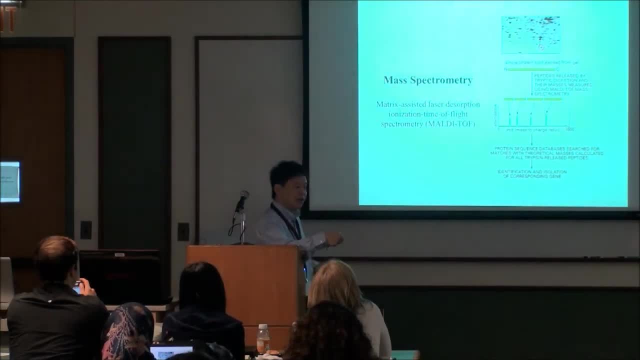 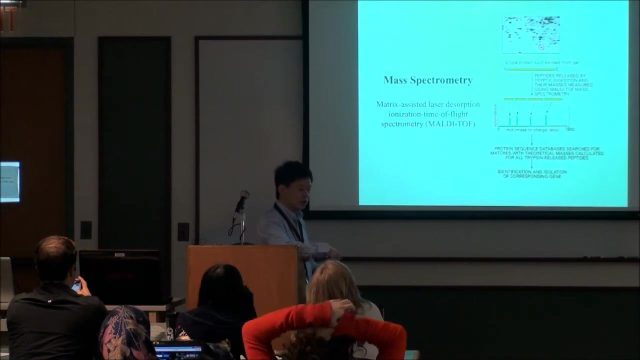 It should match, Just like if everybody has a fingernail or fingerprint already in the library right, And you identify a fingerprint from, for example, a crime site right And you run this, you know, collected this, It's the same. 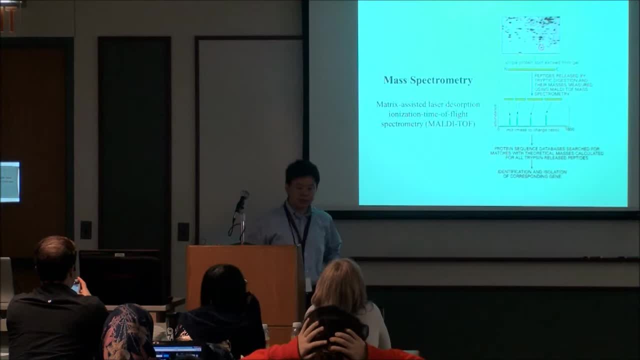 concept? Yeah, very good question. Oh, you are very, extremely lucky you identify a new protein. you know people never know before. Oh, there are some mistakes, you know, in the process, Like, for example, this mixture of proteins. 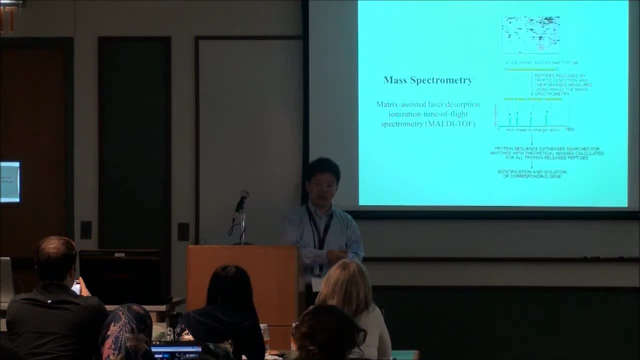 You remember, there are two proteins together. Therefore, when you digest the mixture of the profile- but still there are software which can help you to, you know, identify whether it's a mixture of different proteins superimposed on each other. right? 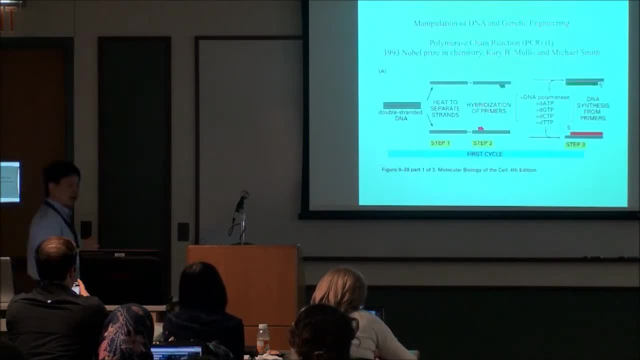 Okay, so so far we already know how to handle: isolate, purify cells. isolate cells and isolate proteins. analyze proteins right. And for the next or rest, we will focus on some DNA technologies which will help you to modify a cell or design. 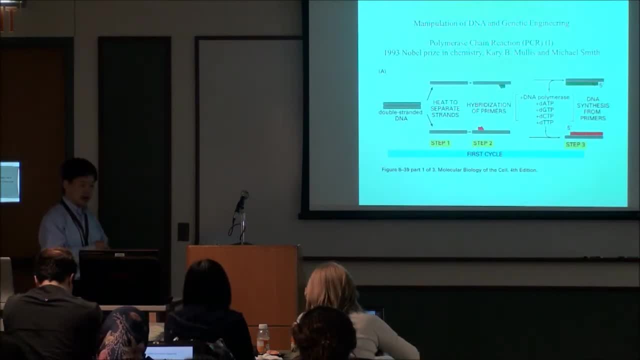 techniques to monitor and detect proteins using like advanced technologies. okay, So before I talk about these DNA technologies, I want to first introduce some simple, you know, techniques which are really well established, called polymer chain reaction. okay, So it's a. 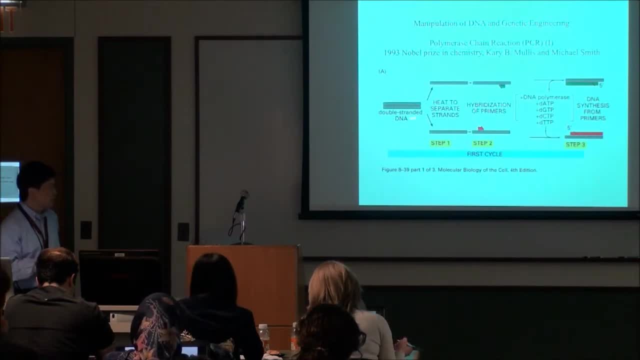 very complex concept and the concept again is quite simple. okay, So it's already known. DNA form: double helix, right? So double strain DNA. If you use heat to separate them, usually it has to be almost 95 degree. 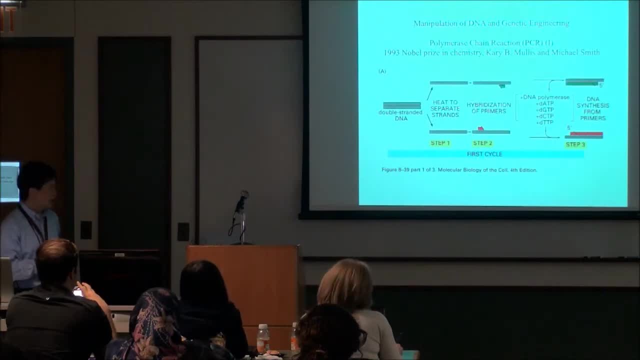 based on sequence of DNA. you are interested, Then they will be amplified. if you add DNA polymerase and all these nucleotides, They will eventually grow until to the end. This one will be the same. So this will be the first cycle in the PCR- so-called. Then you can imagine that's the starting. 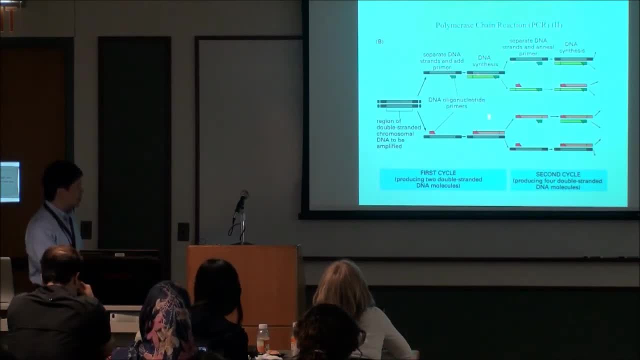 material. After your first cycle, you already have these four DNA sequence right And if you heat them again they will be separate, serving as the new template. If you have all these primer, we call it primer. these are DNA segments. 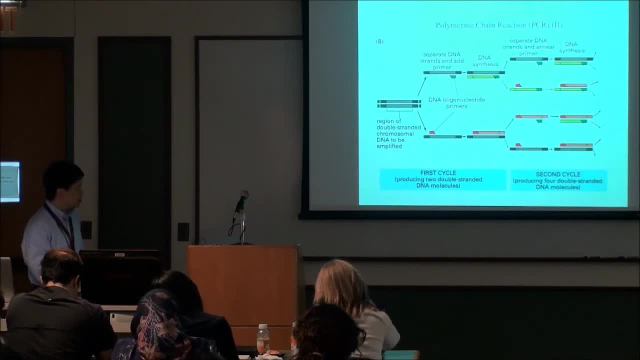 which have annealing on the plant DNA sequence. You will run another cycle, second cycle. you will get- okay, the plant DNA will still stay the same- two pieces right, And this DNA with one sticking end will now become six. Sorry. 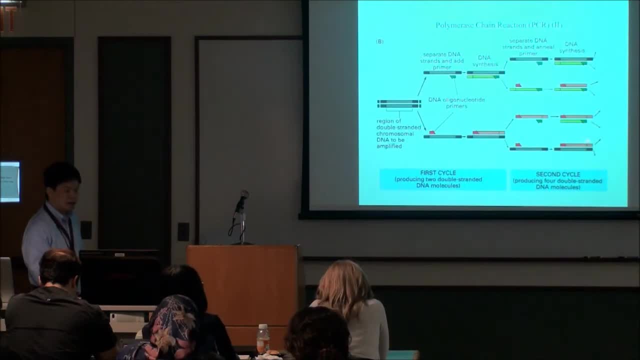 it will become one, two, three, four, four pieces right, With only one sticking end, And you will get two pieces which will be covered by your two DNA primers right Which, covering this, you know, light to light gray zone. okay, These two, That's after. 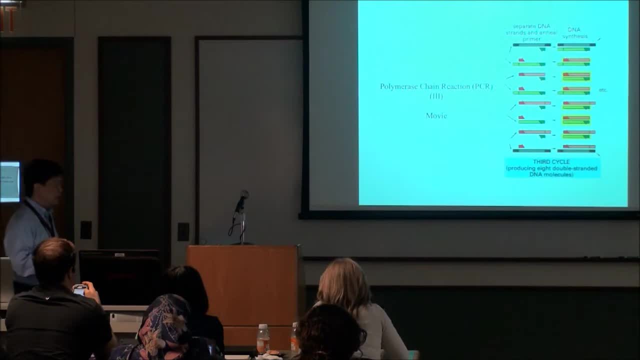 second cycle. So the trick is: after you run another cycle, then you can tell the difference. Now all these template will be separate again and the DNA will be annealed. DNA primer will be annealed and synthesized again. Then you finally got this product after second cycle. The DNA pental sequence will be staying the 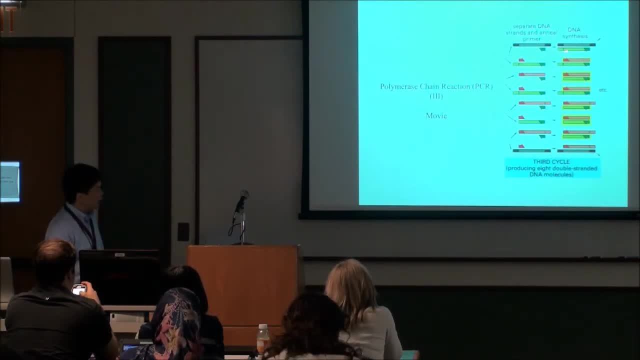 same two pieces right And the DNA with one sticking end now will have one, two, three, four, five, six right. So it's linearly growing. But the product you are interested in which will be, you know, covered in this gray, in the light gray? 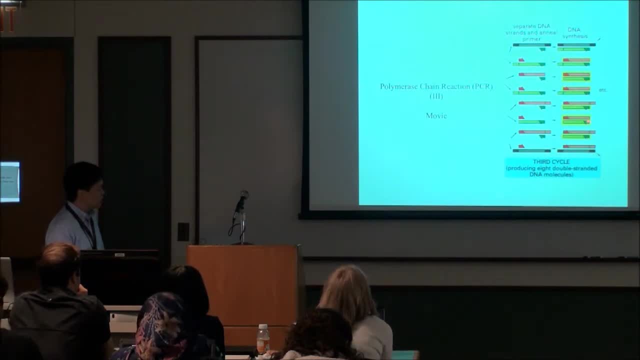 zone will be 1,, 2,, 3,, 4,, 5,, 6,, 7, 8.. So if you can imagine, if you run this cycle continuously for like 30 cycles, after 30 cycles the majority of the DNA product. 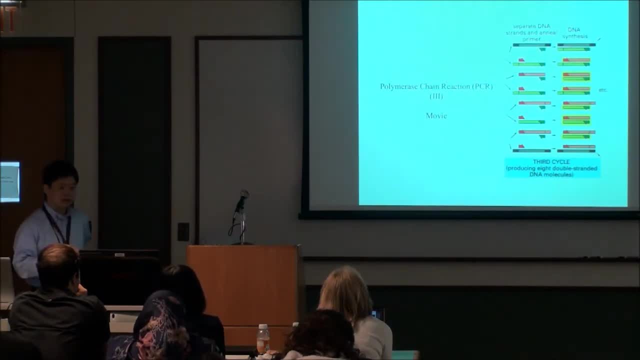 will be the one covering this zone, Is it clear? Because it will grow exponentially, Okay, Whereas the DNA with one sticking end will grow only linearly right And the parented DNA with two sticking ends. they will always stay the same, only two. 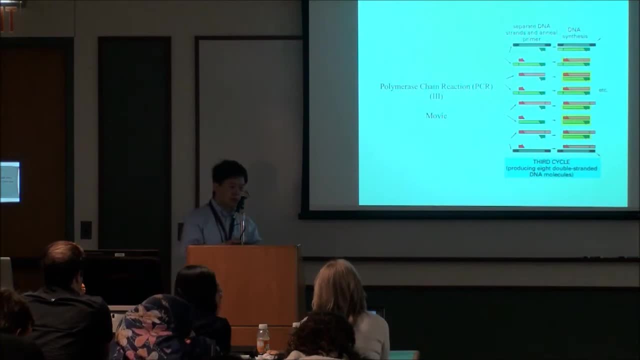 copies. Okay, so basically, the wall basically is outside of this. you know PCR zone. I call it sticking end. Okay, Is it clear so far on the concept of the PCR. So you can imagine with very tiny little material, DNA if you use the PCR. 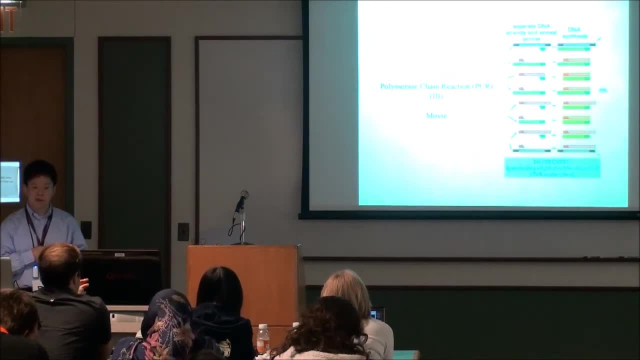 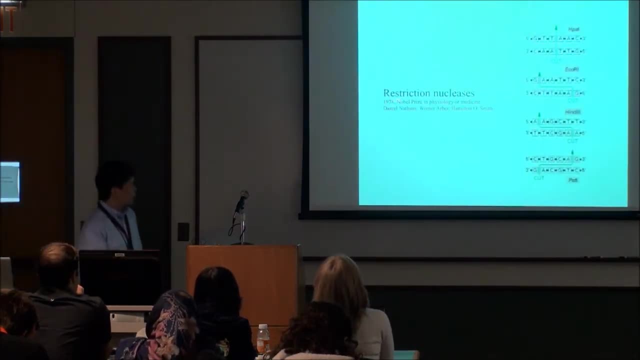 you can amplify to many, many copies, right? So this is the first technology, And the second one to introduce is so called restriction nucleus. okay, So restriction nucleus is also very unique feature. basically, it's kind of protein protease- sorry- nucleus- which can cut. 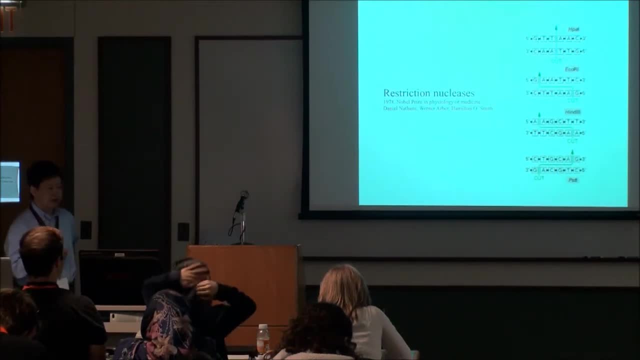 DNAs, but they will cut at specific sequence, Okay. So, as you can imagine, each enzyme or each nucleus will create a unique interface at the cutting side of DNA- okay, and the DNA with the same enzyme cutting will be able to anneal- okay, meaning they can be put together. if they are cut by different enzyme, they 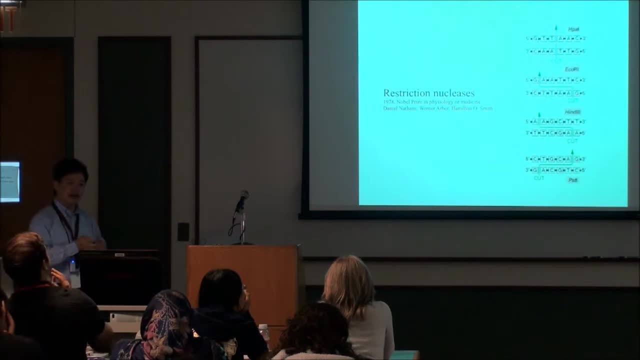 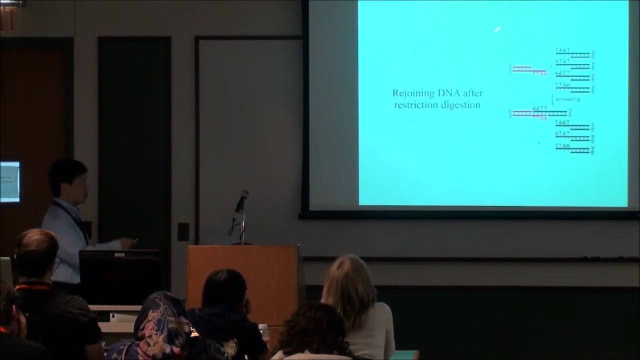 cannot be put together. okay, so this will create a very unique feature: you can use the same enzyme to cut two kinds of DNA and then, if you can join them together, you piece two different protein or two pieces of different DNA together. right, this can be shown here: if you cut one group of DNA with one enzyme and if you 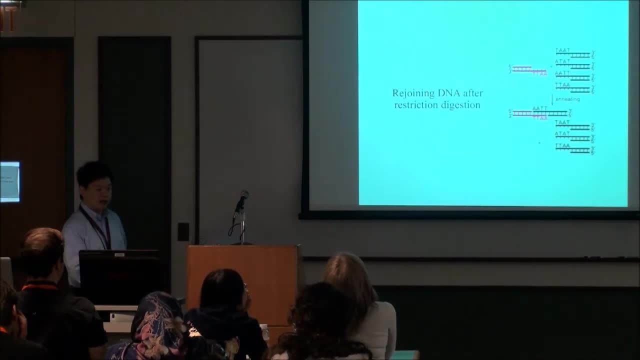 cut another group of DNA with different kind of enzymes, these black DNAs. they will be put together with the red one only when these DNA are cut by the same enzyme. okay, is it clear? only the same enzyme cutting will have same interface. they can be cut by the same enzyme, okay. 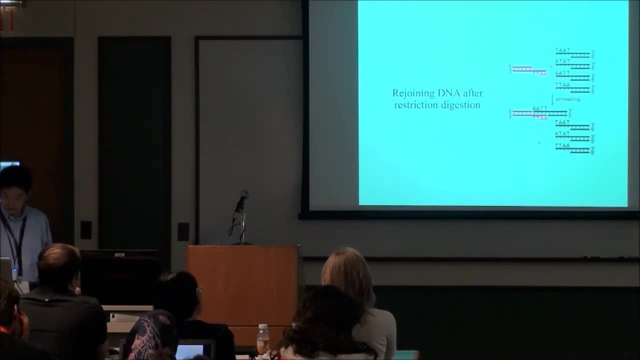 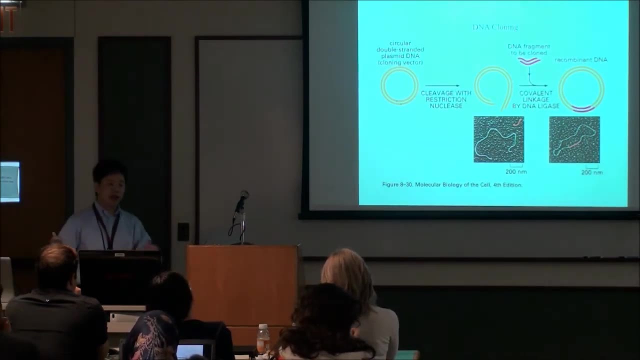 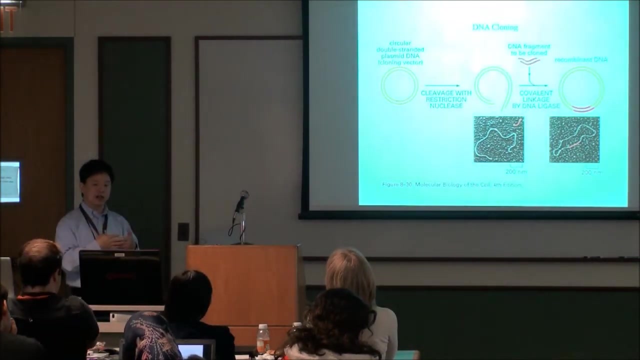 join together. all right, so with this technology there, you can imagine it's easy for you: teller or cut different pieces and piece them together. as long as they have enzyme, same enzyme cutting, they will have same interface, they can be drawn together. their questions: okay, right, yeah, like this will basically you. 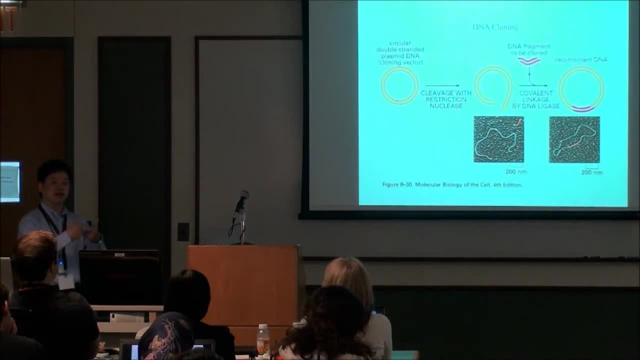 know, have no specificity choosing as long as they have same interface. they were a new and like it. okay. so this is basically among going to: do you use the concept of like it? so, for example, if we have a, you know, a circular day which can be amplified in the bacteria, right, you can cut with one enzyme. okay, if you can do a. 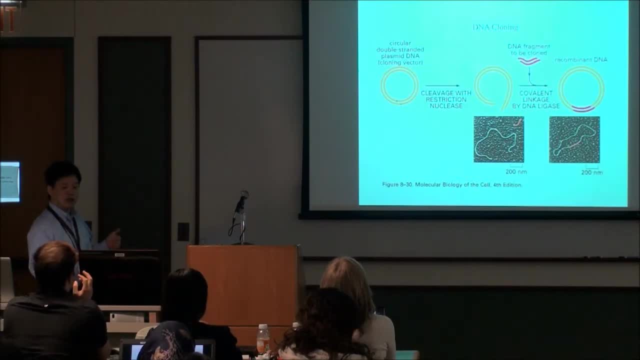 PCR or a specific gene sequence you are interested, and the cut with same enzyme, then these two pieces can be put together, right. right, because they will create same interface. right, they can be joined together by like it and become a new circular DNA which has this rat, you know, enzyme, rat sequence specifically. 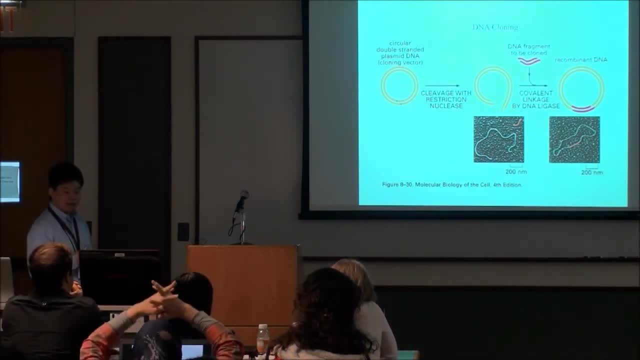 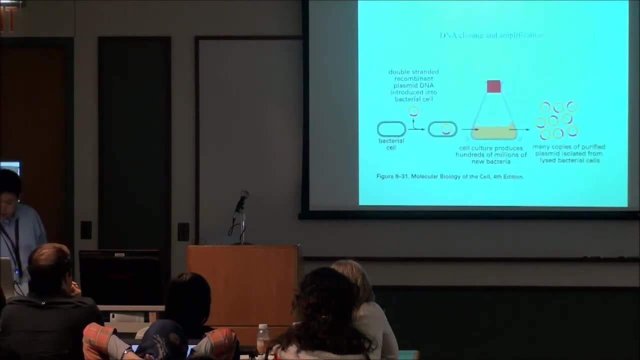 inserted into the DNA vector. okay, then this DNA vector can be put into bacteria. right, if you put into a bacteria, you just transformation and you can grow them. it will create a new DNA, isn't it? is it possible? millions copies of DNA and this DNA now will have the new DNA sequence you are 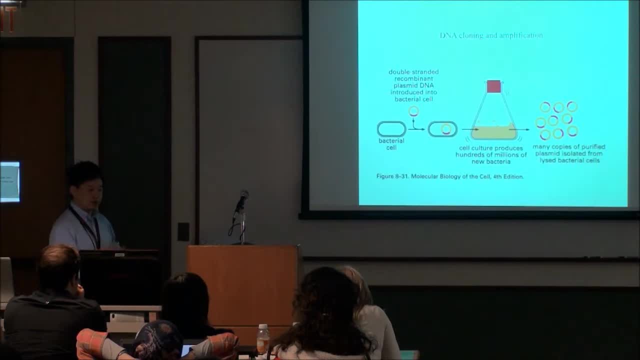 interested in So you can amplify the DNA sequence whatever you want. Is it clear about this molecular cloning, Using restriction enzyme to cut right, to insert into the big circular DNA to allow them to grow and multiply. Okay, now this will be utilized again for the next couple slides. okay, to amplify and. 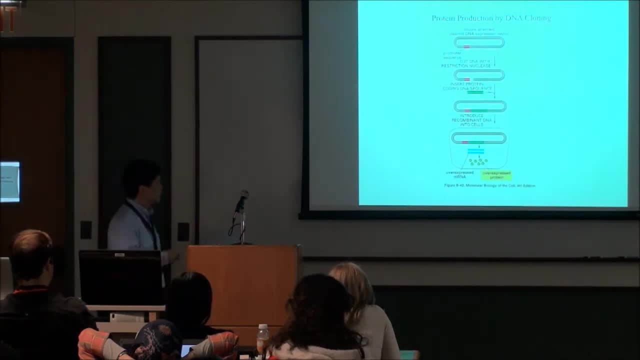 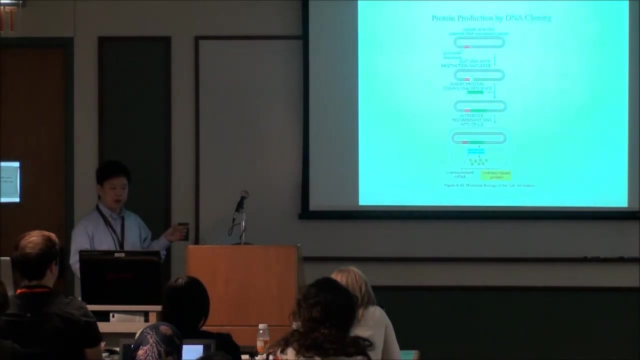 synthesize specific proteins you want. Okay, so in this one, for example, you already have a DNA circular vector and some promoter sequence. okay, and you want to amplify or grow specific protein you are interested. First, you can generate a DNA segment which, if it's expressed, it will produce the protein you want. 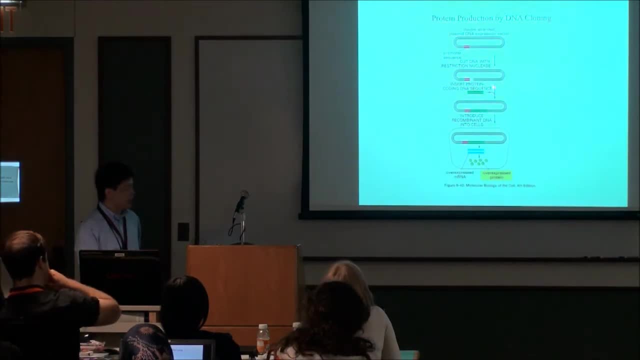 Okay, Then this DNA segment can be cut with the enzyme you designed. With the same enzyme, cut the vector. these two can be pieced together, right and promoter, and the DNA sequence you are interested will be joined together into the integrated circular DNA, And then this DNA can be put into bacteria If you add chemicals to. 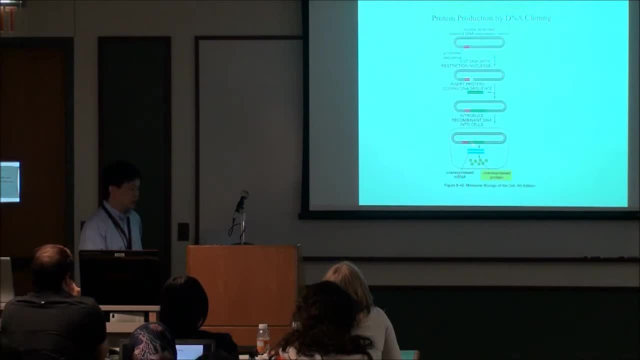 turn on the promoter. the DNA will be transcribed right into the RNA and translating the protein. Okay. Therefore, you can specifically amplify a protein you are interested. right, If you know the gene sequence controlling the protein production, you can do this. 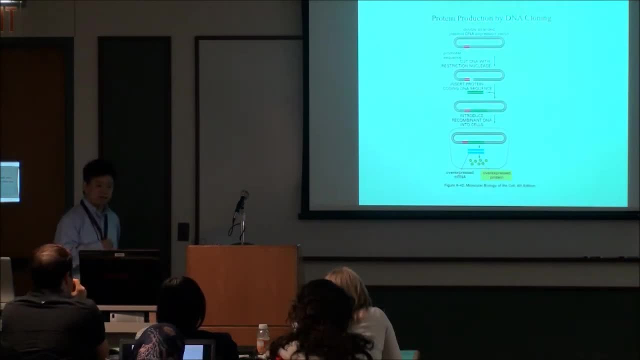 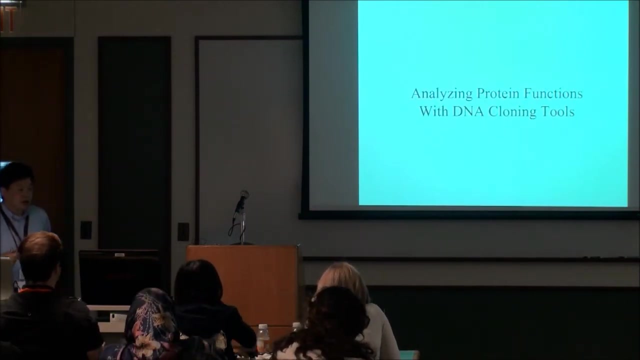 procedure to amplify a protein you are interested. So far, so good, Using the restrained enzyme side and DNA ligation to create this so-called DNA plasmid to produce a protein you want. Okay, So now, with all these DNA technologies, you can do some very tricky things to the 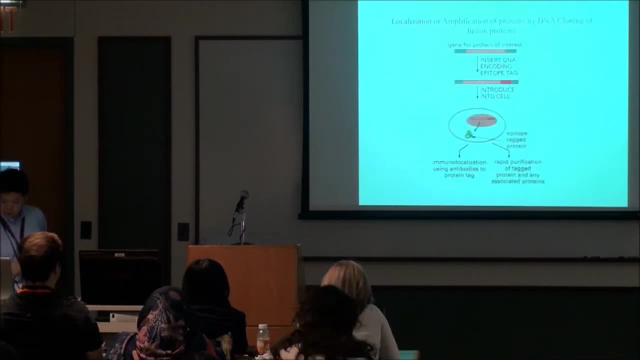 cell to analyze the protein functions. Okay, The first one is you can basically identify a specific protein location, for example Right, If you don't know the antibody- for example some you know relatively new proteins- you don't have antibody available for it. 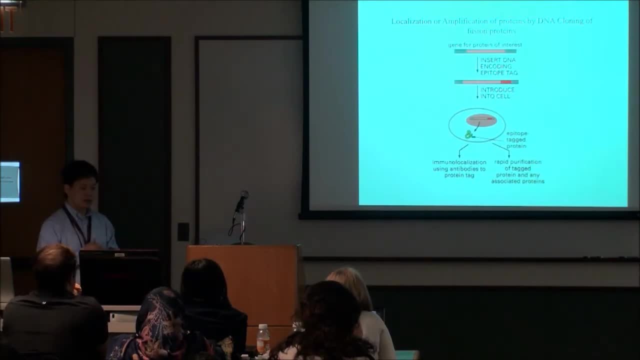 Okay. do you know where this protein is located? DNA technology can help you on that. So usually if you know the protein but you got to know the gene sequence as well- These are all library there- You can directly identify the sequence of the protein and then you can do a gene engineering. put a 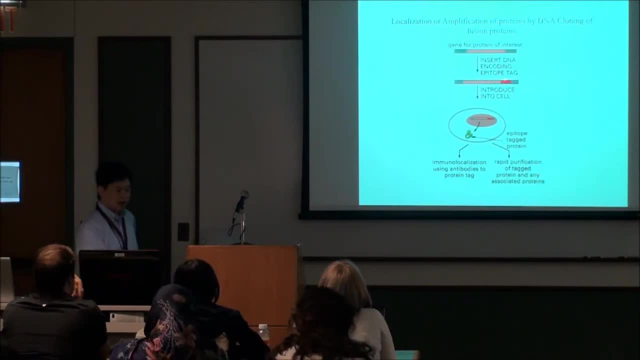 known tag of the DNA sequence. and this DNA sequence will produce a protein or protein motif, which you already have existing antibody to recognize it. So if you use DNA technology to combine these two together, it will eventually put it into the cell and produce a protein. This protein, which doesn't have 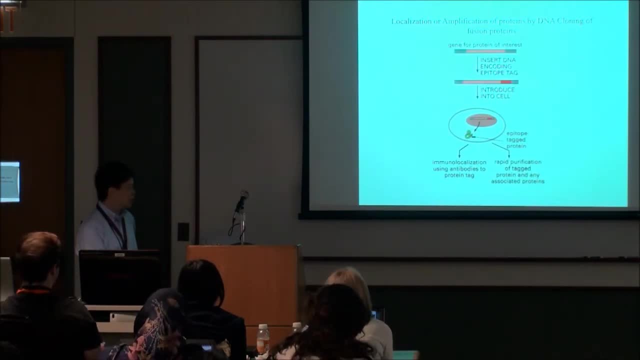 antibody. so you don't have antibody to stare and know where is located. But this motif, which will be created at the same time, has the known antibody right, So you can use antibody to directly detect this motif, to know where these proteins are located. 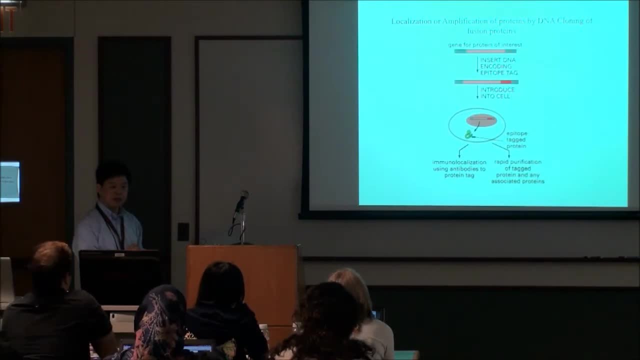 Is it clear to you. Although this protein you are interested in does not have antibodies available, you can use DNA technology to insert a known motif into it so that you can use an existing antibody to recognize the location of this protein. This further will allow you to use the known antibody to recognize this motif. 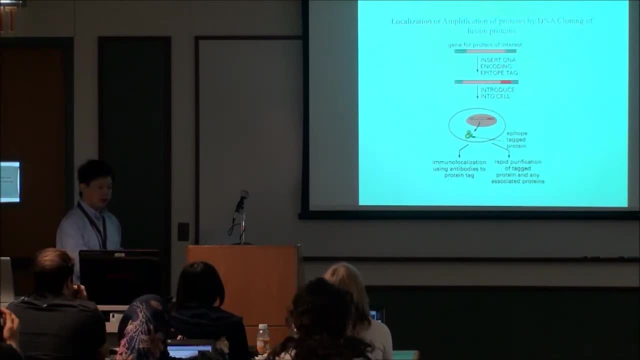 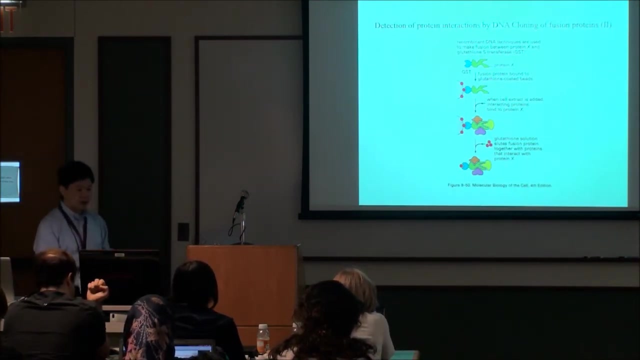 and pull down this protein to analyze the protein you are interested in. So this is one of the technologies You can do the protein interactions by DNA technology. For example, there is a protein X which is relatively new, Although the sequence is known. the DNA sequence controlling this protein X production is known. 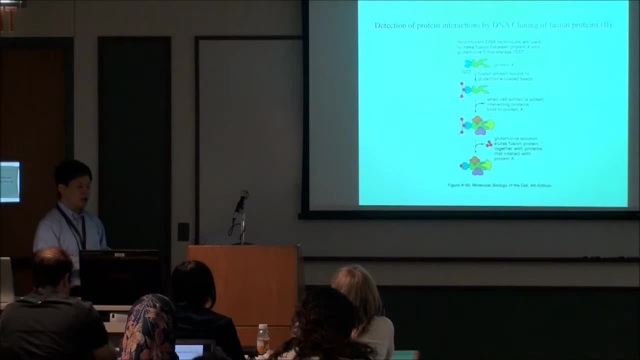 but there is no antibody available. How? How do you study what kind of protein is interacting with the protein X? One way you can do it is you can fuse a known so-called GST glutathione S-transferase tag to it. This you should already know- using DNA technology. 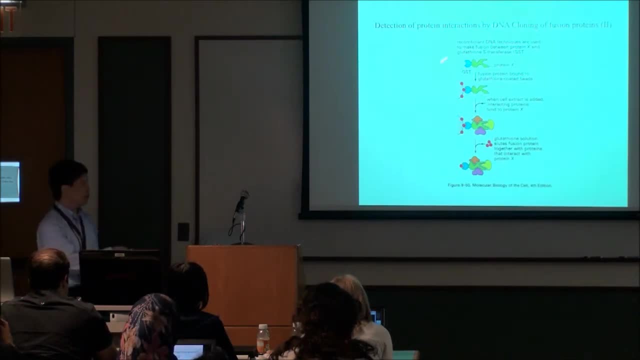 You can join two DNA segments together, It will produce this hybridized protein. So this protein will contain protein X and a GST motif, And there are Bs already available- glutathione Bs- which can specifically bind to the GST And therefore you can centrifuge to collect this protein, protein X. 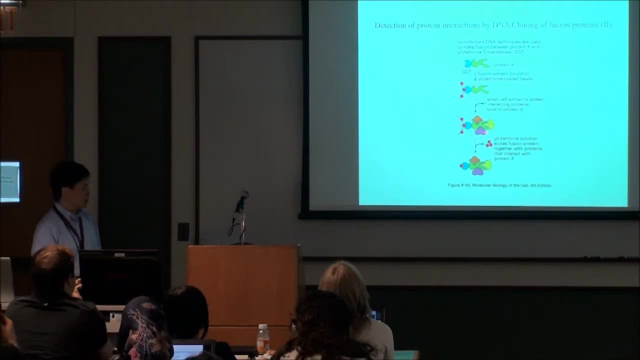 If this protein X is intact with other proteins, like Y, Z, this protein is intact. with this protein, all this whole complex will be pulled down. Is it clear? Is it clear? So if you use beta-mercapital ethanol and SDS to break apart this complex, 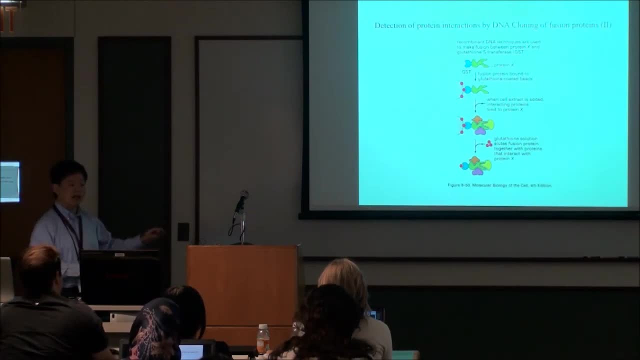 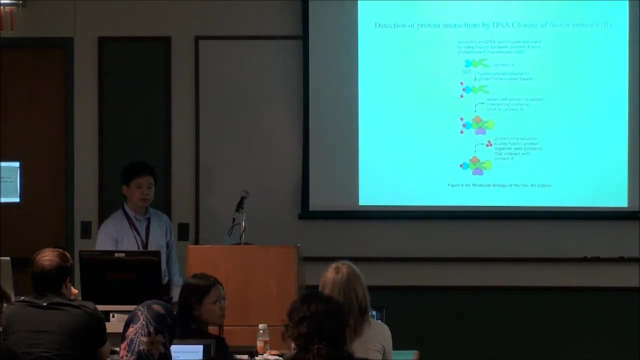 run the SDS gel, okay, and then collect all these DNA dots and, subject to mass spectra, you can identify the identity of all these proteins. Question, Question. So how do you purchase a specific protein interaction in the cell versus, like it just kind of oxidizes in the sulfur? and that's not what I purchase outside of the cell. 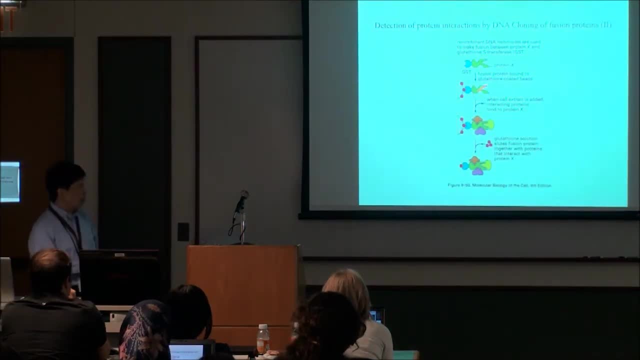 Yes, that's very good. So usually you know, when you do this right, you have to add: when you pull down it, it's the inner cell, lysis, right, It already contains all these, you know, reagents which will prevent, okay, oxidation during the process. 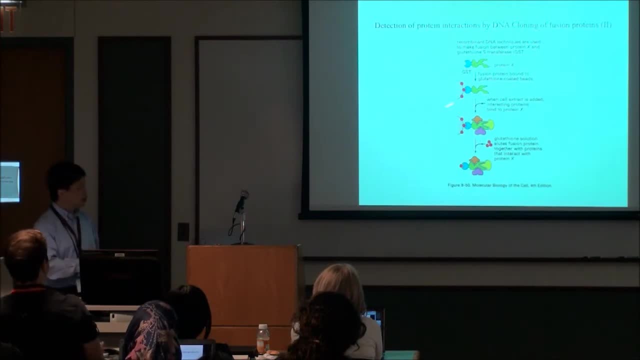 After you pull down, right, you already will separate them and the solution you pull down will only contain these proteins. okay, And when you run the gel, you don't worry about oxidation. You don't worry about oxidation or anything else, because it already contains beta-mercapital ethanol. 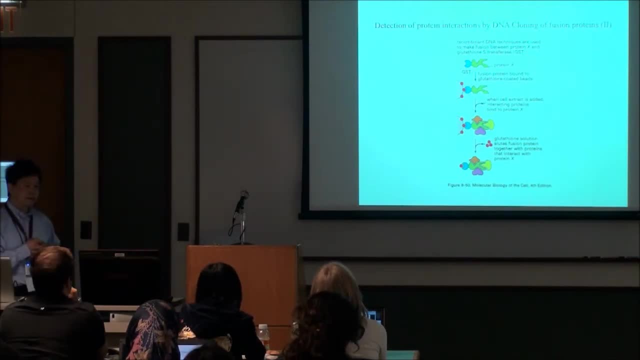 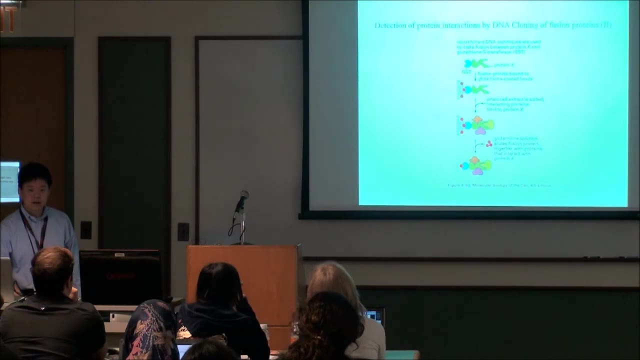 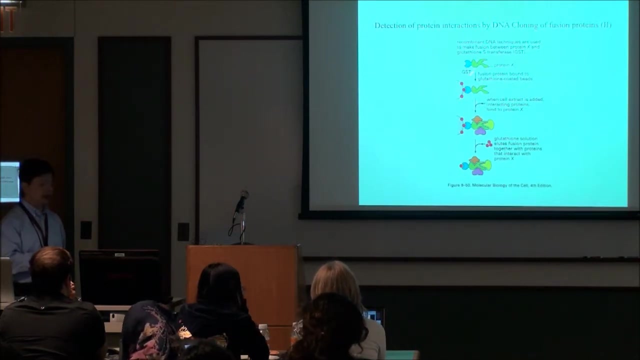 Does that answer your question? Okay, How specific? SDS? No, the GST tag. Oh, GST tag is quite specific. For example, glutamate beads in general will only bind to GST with high affinity. It will not bind to other proteins because this GST actually is not generally produced in the endogenous cells. 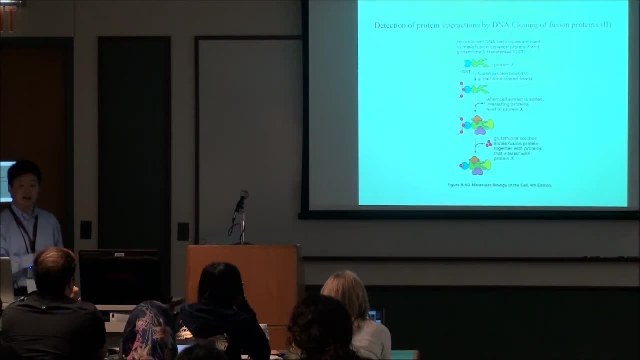 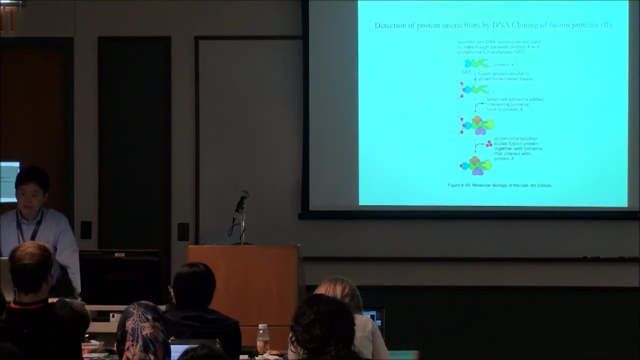 so most of the other proteins. they don't have this tag. They will not be pulled down. Is it clear? This GST is an exogenous motif which you don't have in the native cells. Okay, So does GST affect the protein function? 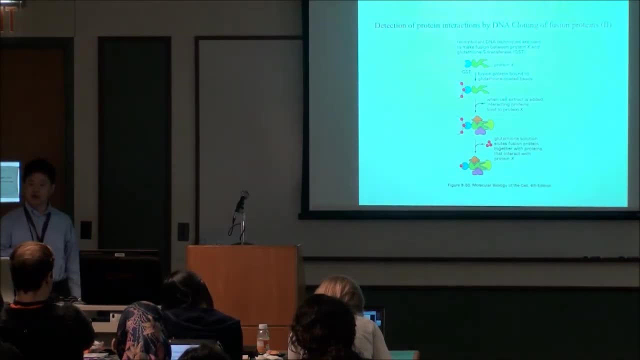 Very good question. For most of the proteins people tested it did not, Okay. But you cannot deny that this, of course, will affect the kinetics. how fast they move, you know. But in general it's not. But in general, their binding, their location are similar. 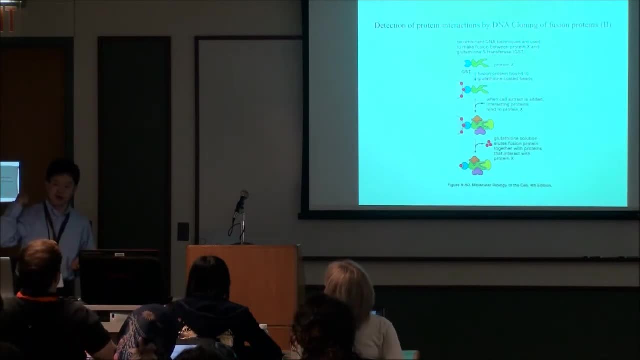 Okay, You know, this GST obviously will put a bag on this protein, right? So it will probably walk or move slowly. You have a question? No, Okay, So is it clear: If you have a protein which does not have antibody available, you can still use genetic technology, right? 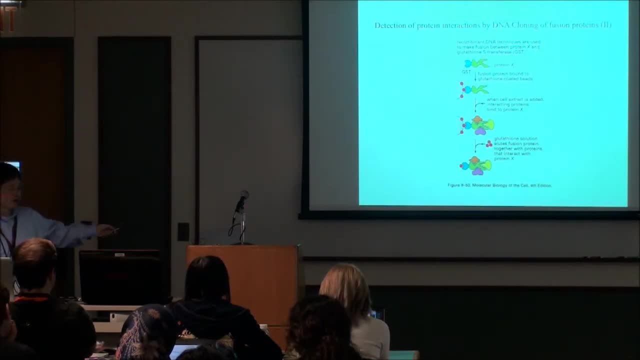 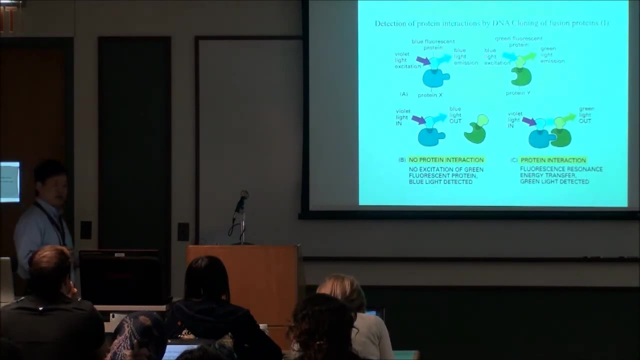 To design a hybrid protein For you to study how this protein is intact with other proteins, Okay, And you further can use another technology, so-called FLAT- fluorescence resonant energy transfer technology, to study that. So the idea is, you want to know whether a protein X and a protein Y, they are intact with each other. 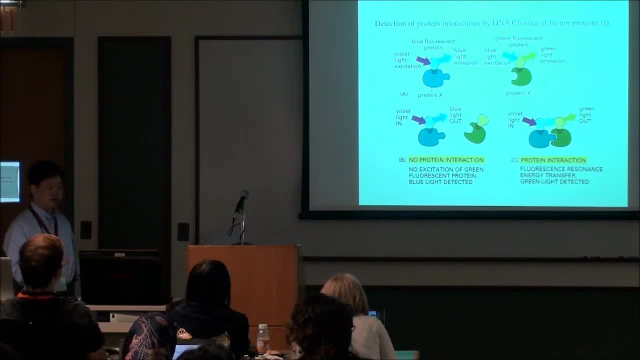 Okay, How do you know? How do you do that? Right, If there's no antibody available for these proteins, Genetic technology can also help you to do this. Basically, what you can do is: you can do this: Basically, what you can do is you fuse a fluorescent protein. 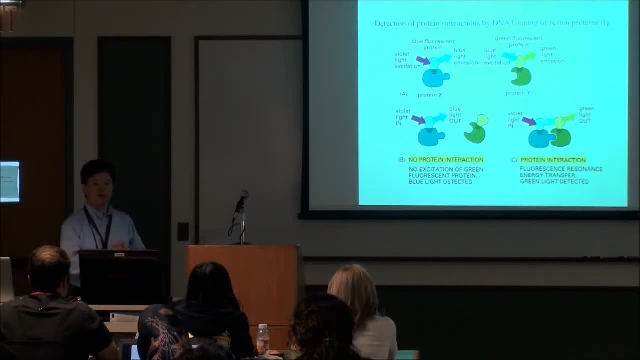 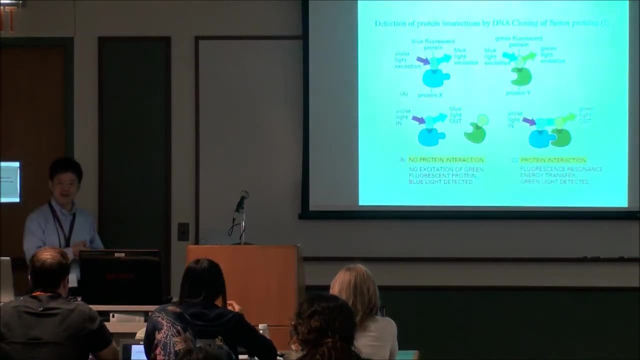 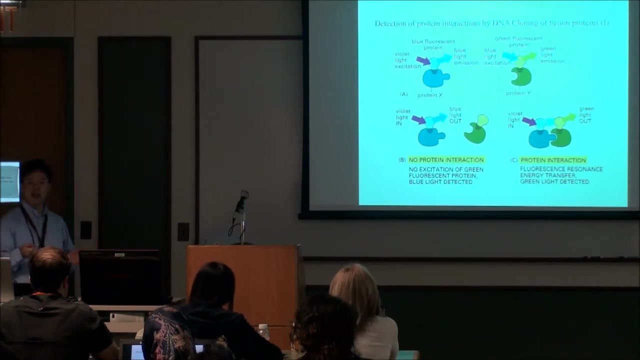 How many of you heard about fluorescent proteins? Green fluorescent proteins? Okay, Not many. Yes, GFP, GFP. Okay, Got a couple more. So, basically, these are proteins which are genetically encoded, Meaning you can use a protein DNA sequence to put in the cell to produce a protein. 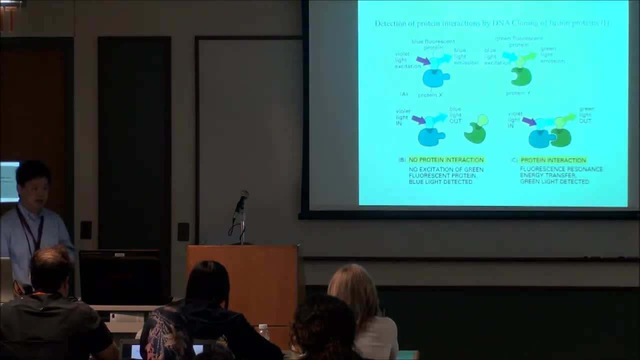 And this protein will be fluorescent Because it will form a chromophore in the cell. Okay, These are called fluorescent proteins And there are different colors of fluorescent proteins. Okay, So the technology basically showing here is: you can put two DNA sequences together. 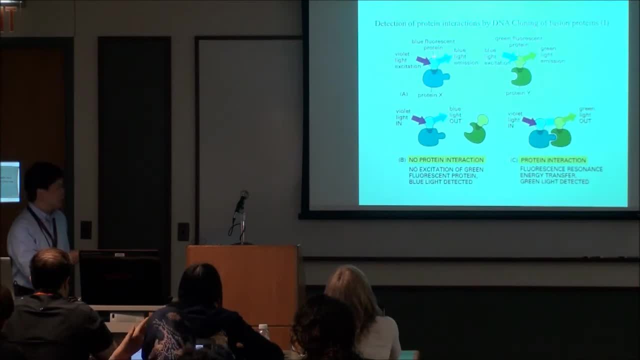 One is a sequence for the protein X, One is a DNA sequence for the so-called blue fluorescent protein. If you put them together, you will have hybrid protein right, Containing protein X and blue fluorescent protein, And you can do the same thing for the protein Y, with another color of fluorescent protein. 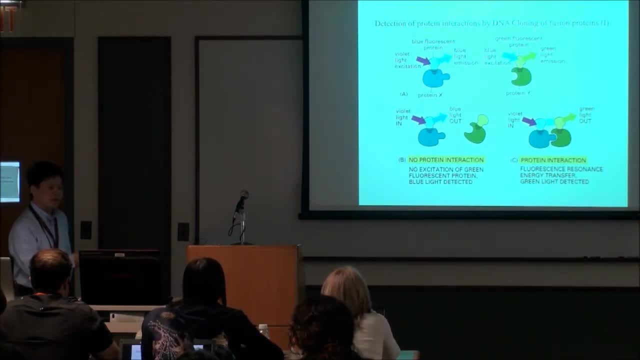 Okay, So you have two hybrid proteins, right, If these two proteins, if X and Y, are not intact, then if you directly shine on the blue fluorescent protein, because there's no energy transfer, okay, the blue light will come out because it will be directly excited. 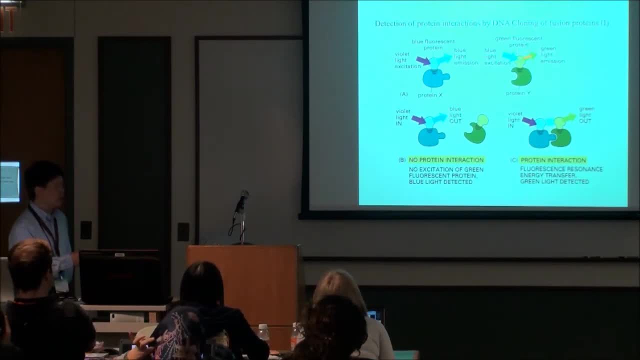 But this yellow one will not be, or green one will not be excited. So you don't see the green color out, Is it clear? However, if protein X and Y are intact to each other, they will get together. Then, if you directly excite on the blue one, you will see a green color out. 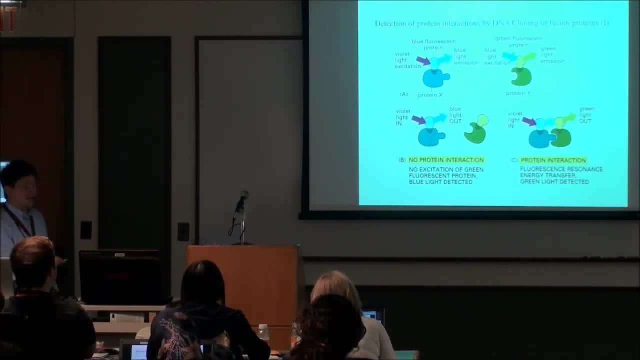 So it's a very simple concept. If you generate these two sets of hybrid proteins put in the cell, you shine the cell with like purple or violet light. if you see a blue color, you know these two proteins. they. 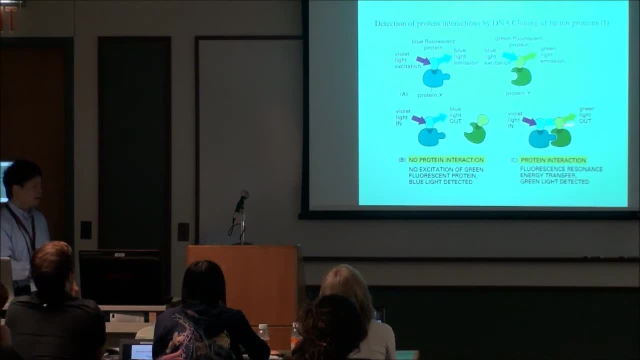 are only intact. Okay, If you shine the cell with the same violet color or the light and you see a green color out, you know protein X and Y are intact to each other. Is it clear? Genetic engineering can tell you, help you to do this analysis. 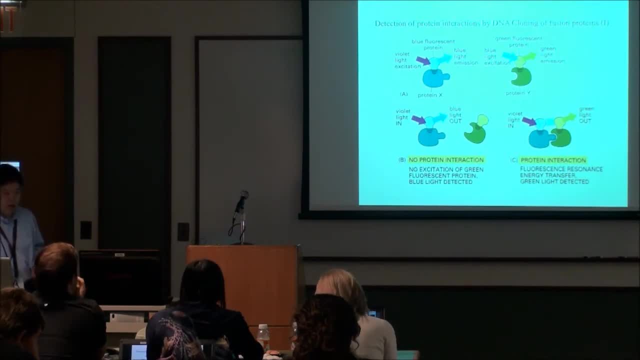 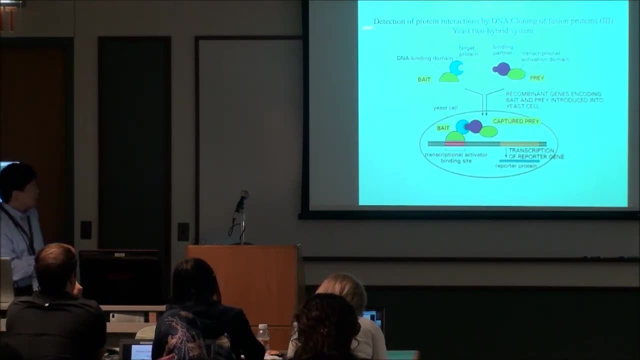 Okay, Otherwise you know, there's not much way for you to do that. Another technology which can help you to do the protein interaction is called yeast to hybrid system. Okay, It's also a similar kind of idea, but it contains a bait domain which can bind to. 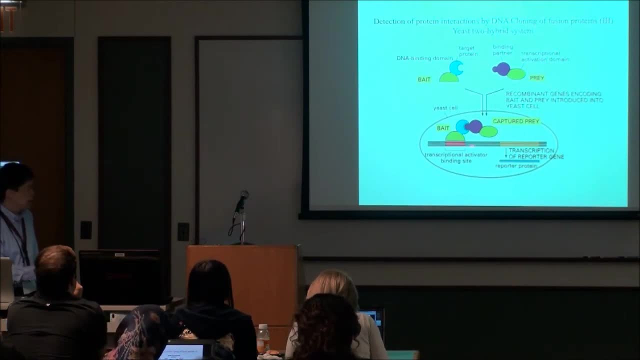 a specific DNA sequence. Usually it's located close to the transcription site And it will have a target protein and a binding partner. You want to test whether these two proteins are intact to each other? Okay, And this binding partner will be fused to a pre-protein. 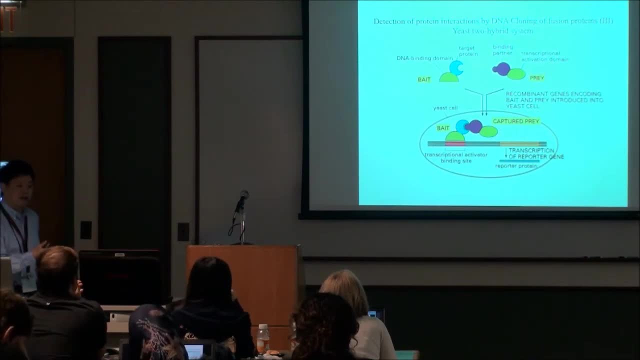 Pre-protein. basically, is a transcription factor okay, or activator to turn on the gene expression or protein expression Okay. So if these two proteins, they can intact to each other. if you put these two things into the cell, this bait domain will bind to a specific transcription activated binding. 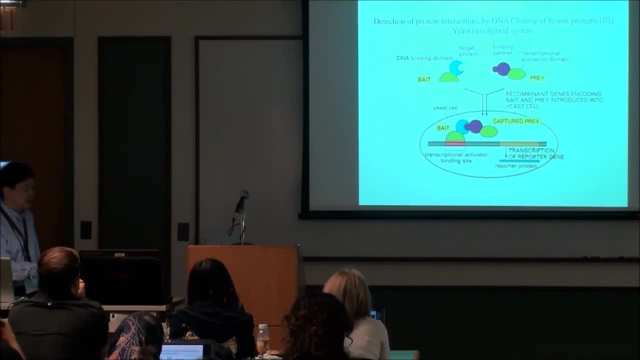 domain right. So this target protein will go there. If these two intact to each other, this plate will also go to turn on the specific reporter protein. So if you see a reporter protein coming out, you know these two intact to each other. 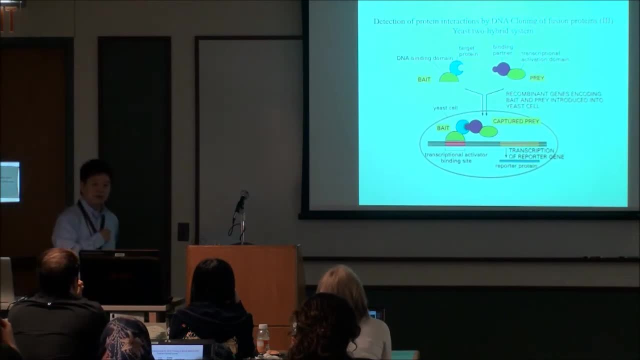 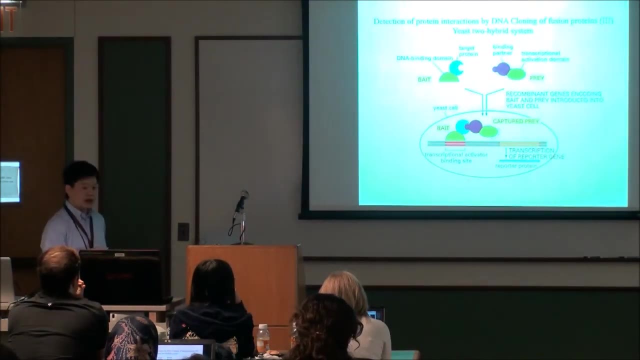 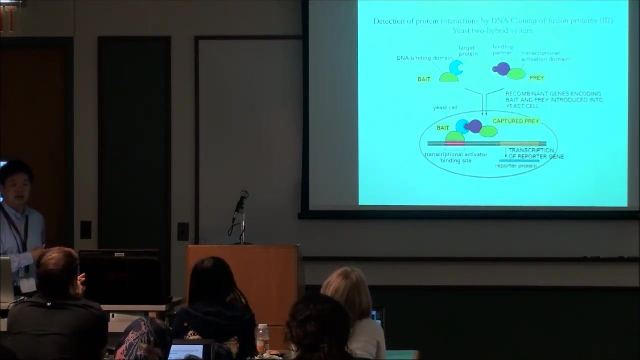 Question: male in audience question. male in audience question. Okay, Very good question. So these are proteins, right? They will be all encoded by a specific gene sequence, right? What you do is just introduce two genes into the cell, So the cell will produce these two proteins, okay? 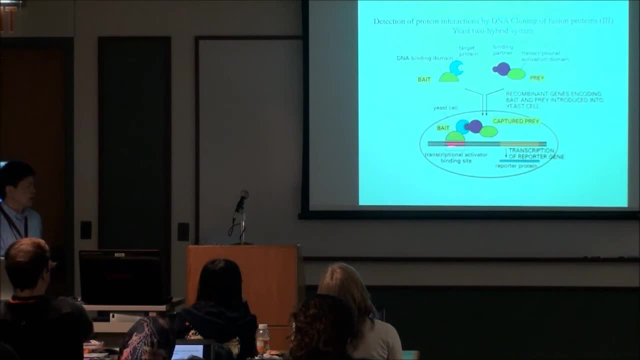 If they're intact to each other, this bait bind to DNA will be in the DNA. bind to the DNA will pull the prey to the side to turn on the gene expression. If they don't bind, then this bait will go, but prey cannot be pulled together so that the gene expression will not. 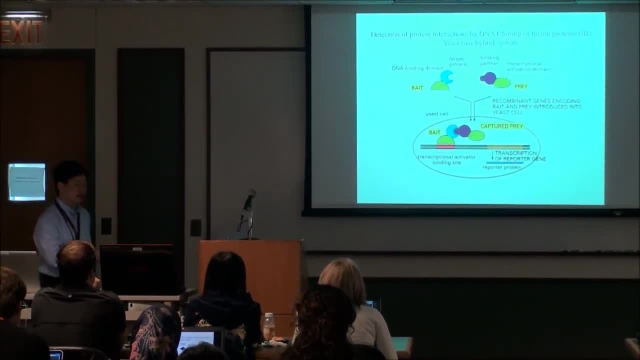 turn on? Is it clear? So, based on the reported gene expression, you can know whether these two are intact to each other or not. This is called the yeast-to-herbivore system, Another system which can help you to study protein-protein intactions. 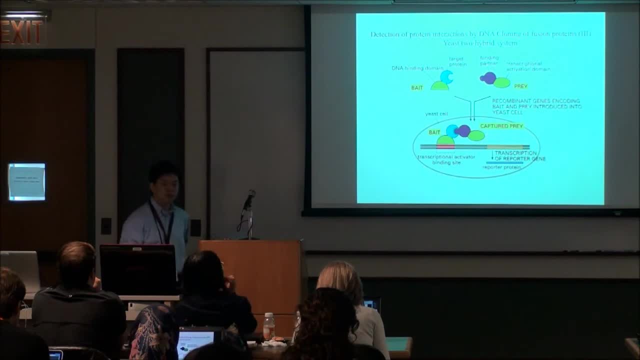 Question: So, in order to use this, you need to have the knowledge of where they interact. You don't, You don't need to know. So when you fuse the proteins, how can you be sure that the interaction regions are actually exposed to that? 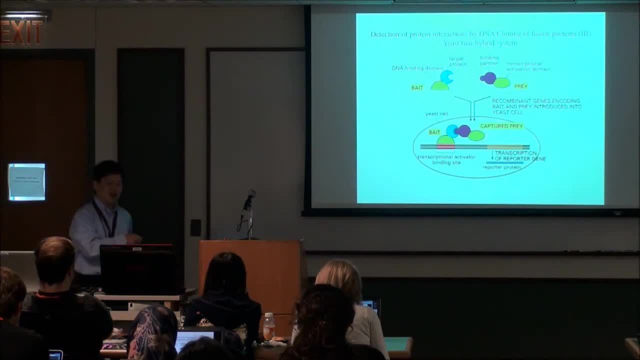 Very good question. That's more advanced technology. Of course, this is a very simple technology. People say: fuse them together. But in general when you fuse these two DNA segments together, people will put a relatively flexible linker. You can put a flexible linker between them with like glycine, which doesn't have side chains. 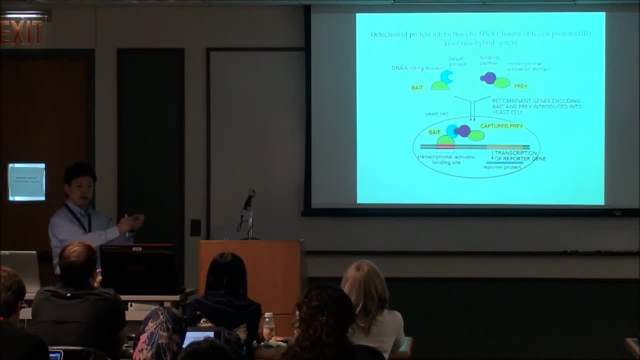 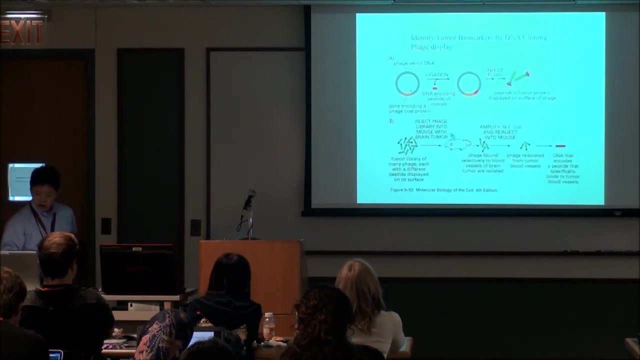 So these two domains are relatively, you know, free or flexible between them. You will not mask any functional domain of these. OK, That's what typically people do. Use a short peptide containing glycine mainly- I think this is my last slide about research- So this DNA technology can also help you to design specific peptide. 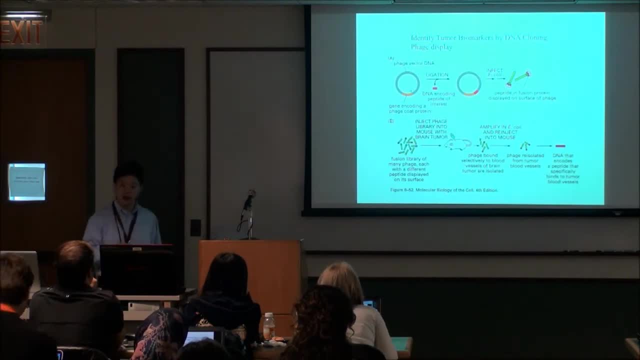 which can have some functions, such as block the tumor growth or produce some toxic substance to kill the tumor, for example. So this technology is called phage display. Phage display: the concept is basically you have phage vector DNA and also a gene encoding. 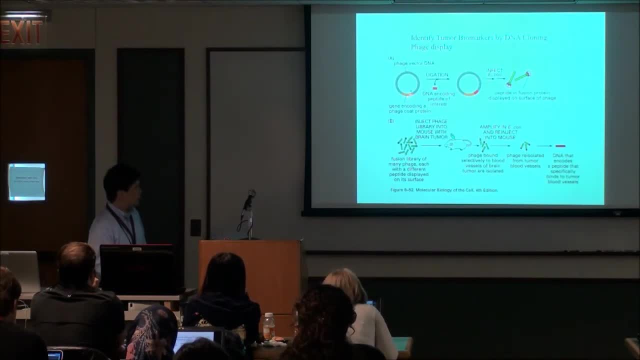 a phage code protein Here. this code protein will help to deliver. if you have a protein produced, it will go to the surface of the bacteria. So if you insert a DNA encoding peptide, DNA encoding peptide, join them together, you will have a bacteria which has this peptide exposed on the surface of the bacteria. 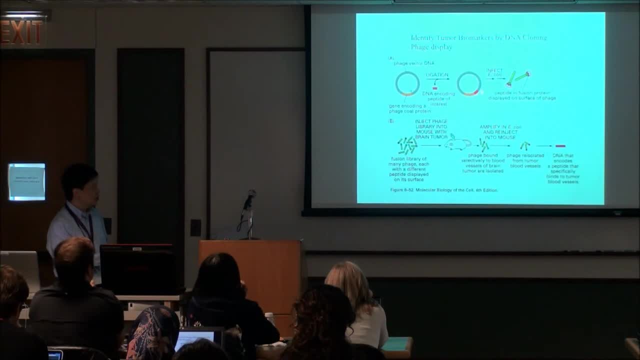 Is this one clear. This yellow thing will help this red peptide to go To the surface If you express this construct in the bacteria. So it's already well established technology. You can generate this kind of particularly this red zone using like random mutagenesis. 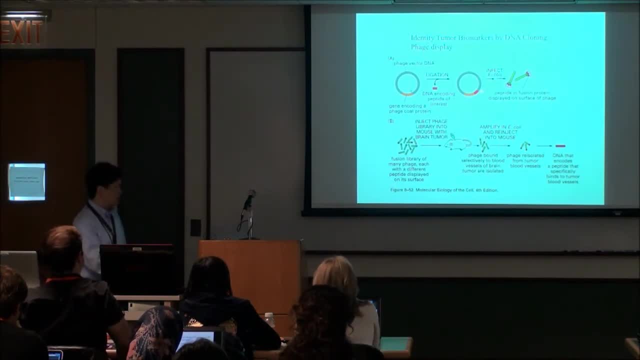 or library technology to generate a milling, so this different sequence of the red zones. And then if you insert this library after this yellow tag, you can imagine if you transform this DNA into the bacteria. Each bacteria would carry peptide with different sequence. Is it clear? 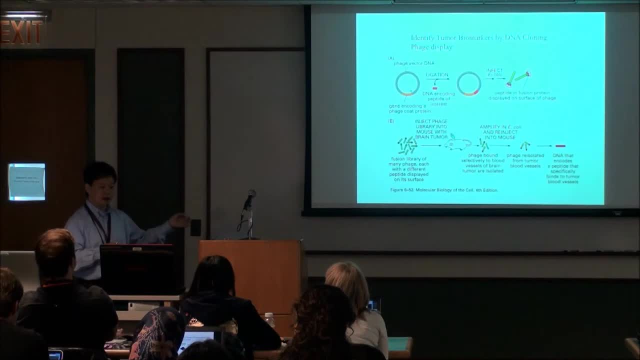 If you have a milling of bacteria, each bacteria will have different peptide on top, So you essentially generate a library of peptide expressed on the bacteria surface. Each peptide is different in sequence. So then, if you have this library, You have, for example, let's say, a milling of bacteria. 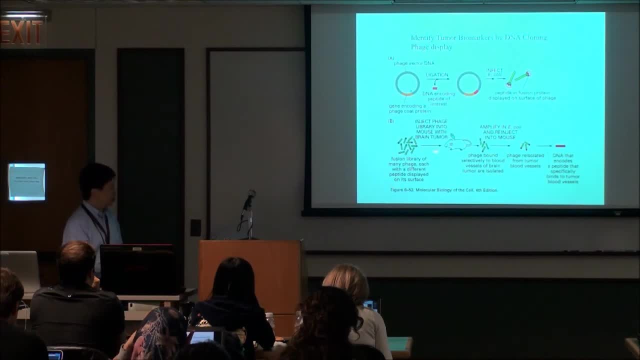 Okay, Expressing different peptide injecting the mice, okay. And then these mice, of course, have some tumor growing already, right. And then you inject this library And some of them, because all the peptide have different sequence, right. And some of them they will have specific affinity binding to the tumor, okay. 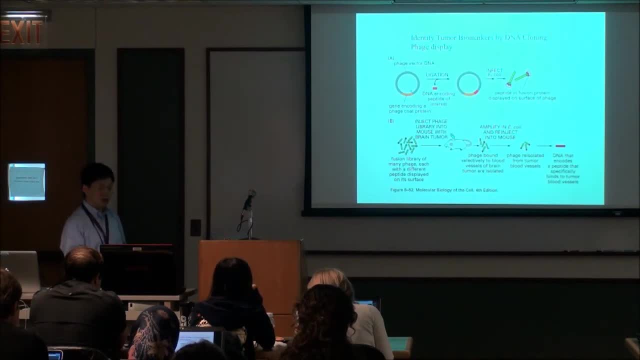 So after you inject that for a couple of days and they isolate the tumor And some of the bacteria will stick to the tumor right, And some of them, of course, easily, you know, wash out Because they don't have specific affinity binding to the tumor. okay, 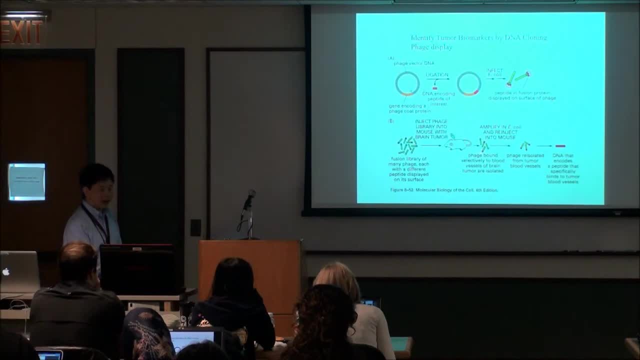 And then you collect the bacteria. These bacteria will have the peptide which have high affinity binding to the tumor. okay, And you purify these bacteria and, you know, amplify the DNA sequence, all this from bacteria, And you know which DNA sequence will generate the peptide which will have high affinity. 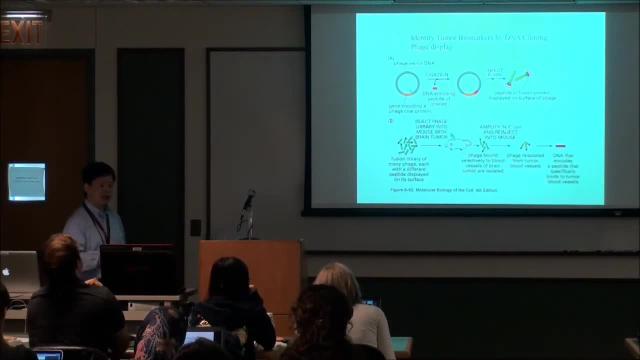 specifically targeting to the tumor, Is it clear? So, for example, finally you got this DNA sequence which you know will produce the peptide. If this peptide is put into the mice, it will go to the tumor. okay, So if you can imagine, if you already know this sequence, that will be very useful, right? 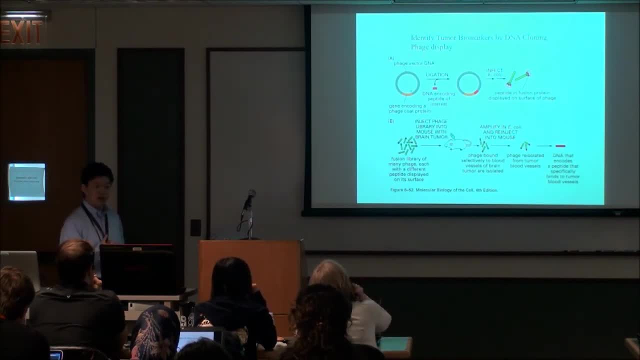 You can put another gene sequence which will produce like toxic compound. Or you can even directly add a toxic chemical to it with the peptide. if you inject in the tumor right, This thing will help you to go to the tumor and this toxic chemical will kill the tumor. 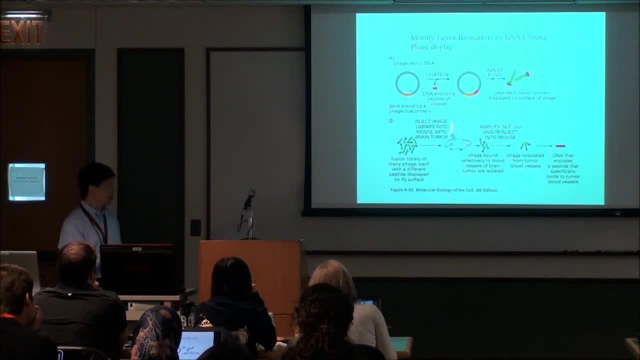 Is it clear. So this is a relatively high throughput. you know You don't need to know anything about which peptide will bind to the tumor. You generate a library- a million different kinds of peptides- right using the phage display, and it will automatically help you to select the peptide which will bind to the 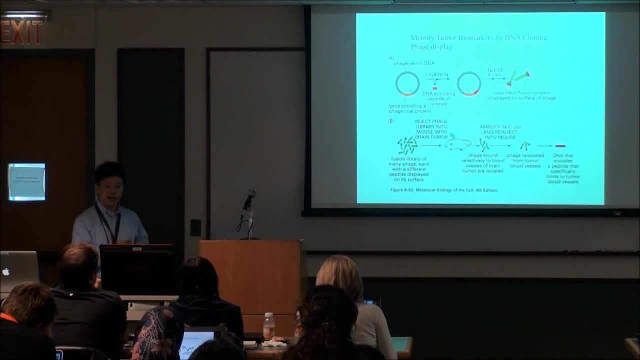 tumor. Is it clear? Okay, Is it clear so far, You don't need to know which one, which sequence, is good for the tumor. It will help you select the peptide which will specifically bind the tumor. A question So: do you guys like, does it take into account the introns and exons? 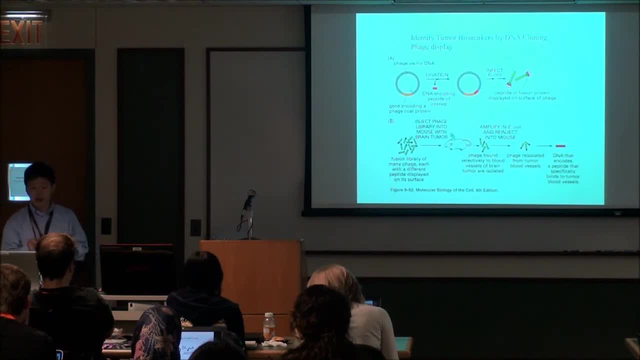 This one, you don't need to worry. These are all exons, exogenous protein for DNA segments. Okay Yeah, These are all designed. you know, plasma, Everything will be produced. Oh okay, Okay Yeah, Is it clear to you? 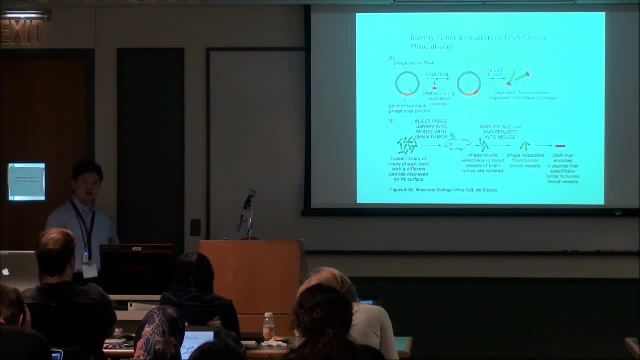 You can generate a library with different peptide sequence injecting the mice- okay, and the tumor will basically absorb all the peptide with high affinity to the tumor site, right. Then you collect the tumor- okay, you know which sequence it is, using the technology. 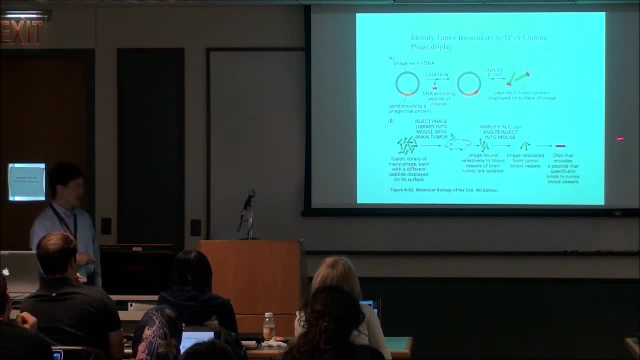 we already talked about right, And if you know which sequence it is, you can collect the tumor. And if you know the sequence, you can conjugate to a toxin right inject again, then it will go to the tumor site to kill the tumor. 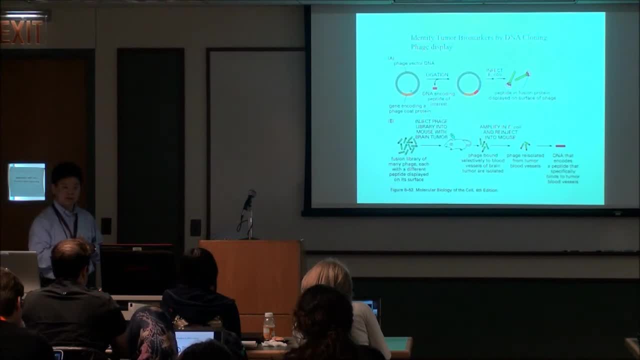 I know that it doesn't go to the other site. Very good question. Of course you have to select right. You know you collect from tumor. At the same time, you know you probably want to check whether this will go to other site. 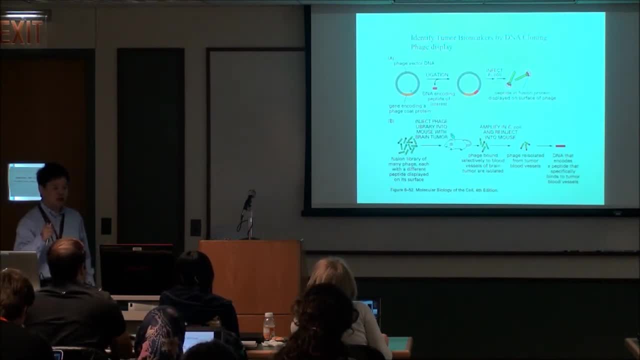 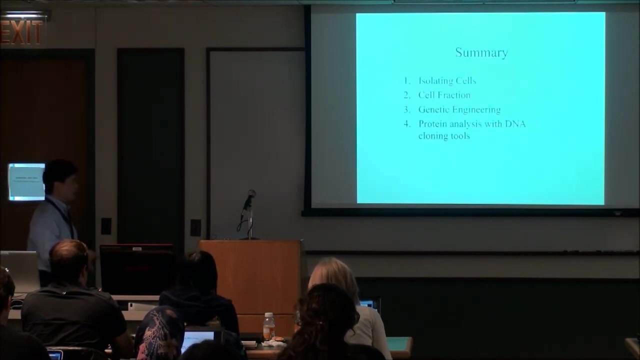 But because you can generate a library, you can always select to specifically choose the peptide which, with high specificity, Only go to tumors, right? Is it clear on this technology? Okay, So I think just this is a summary. You probably already know, right? 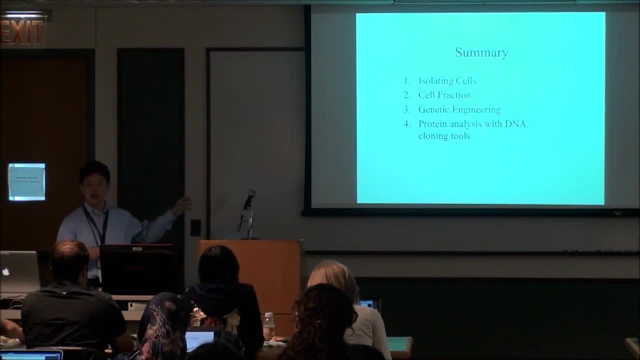 Basically, we covered how you can select a specific cell type from the tissue from the animal bodies and how you break apart the cell body, collect our protein inside, how you use different technology to study what are these proteins. which modification has happened on these proteins? 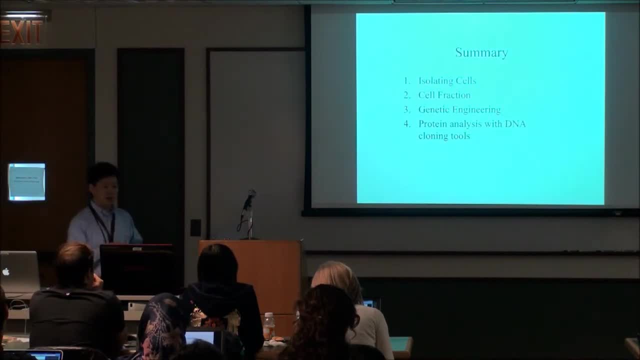 And we also talked about genetic engineering, which will be very powerful for you to manipulate and create hybridized proteins. And these hybridized proteins will help you to study the protein-protein interactions and help you to select the peptide or protein motif which will specifically target some. 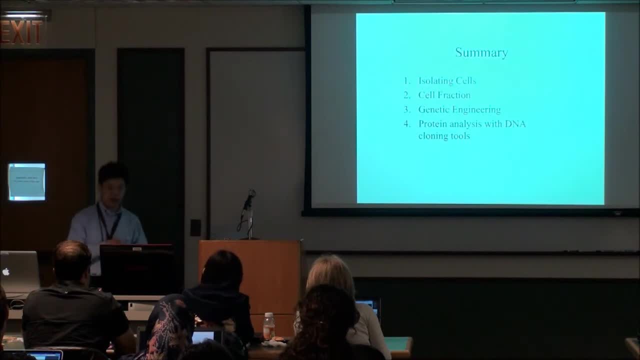 tumors or other disease site. if you want, okay, And this can also help you to do very high throughput. you know screening technology. You don't really need to know which peptide or which protein. Okay, If you have a protein motif well-bound to tumor, well-bound to the disease site, this 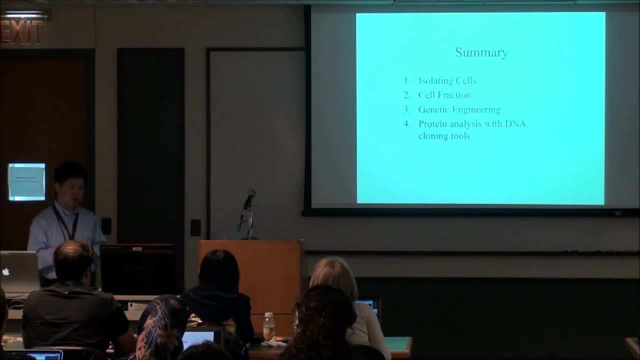 library will help you to quickly select. you know, choose the one which you are interested in. Okay, That's all for my talk. If there are any other questions, I'll be happy to answer. No more. Already asked everything, Okay. 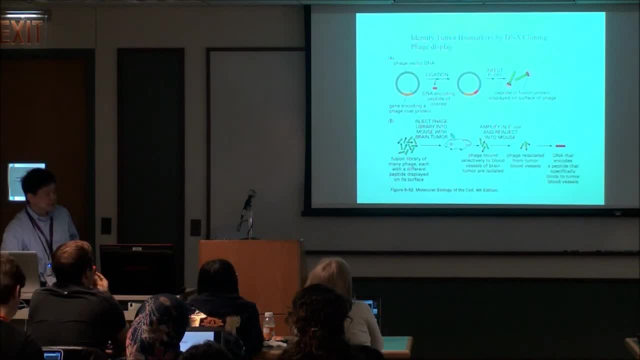 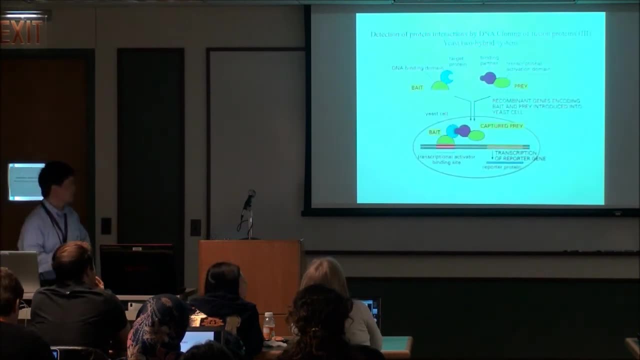 Which slide do you want to? On the slide of the: Okay, Okay, This one. Oh, this one. Yeah, This one, This one, This one, Okay. Molecular beacon? Yes, I think it's quite different. 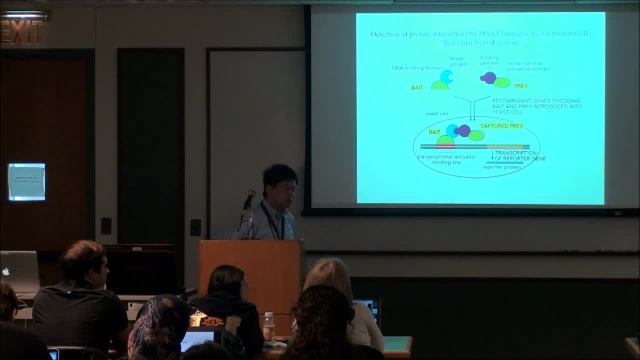 The molecular beacon. most of the time people are doing, like all directly talk about the interaction between the DNA or RNA sequence, whether they have, you know, hybridized site. So these are basically talking about a protein, whether the two proteins are intact to each. 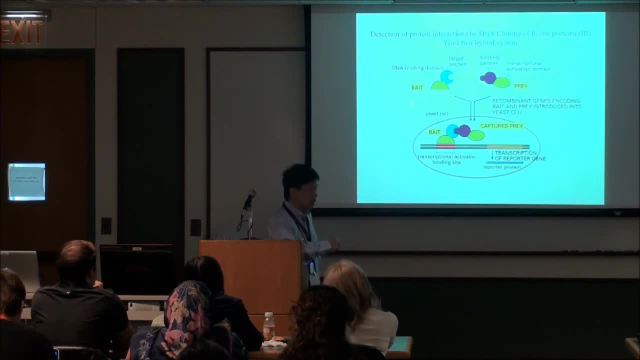 other. Yeah, So these are DNA sequence. hybrid DNA sequence will generate hybrid proteins, right, And this one will bind to the DNA segment and this one will turn on the gene expression. right, And if these two proteins are not intact to each other, they will be separate. 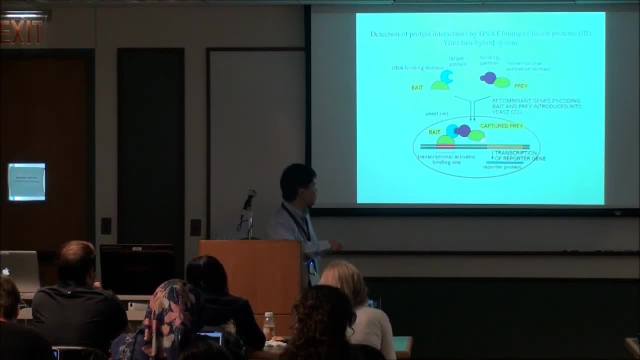 Although these will bind to the specific DNA segment, but these will not go to the site to turn on the gene expression. So basically, when the two proteins are intact to each other, this bait will pull and recruit the prey to the site to turn on the gene expression. 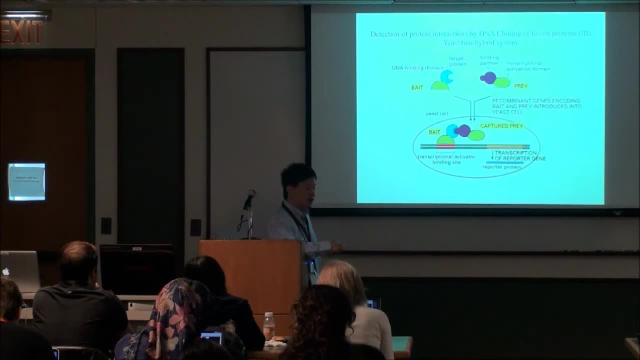 So, basically, based on the gene expression, you can know whether these two are intact to each other. If they're intact, you've got a lot of gene expression. If they don't, you don't have gene expression. Okay, So would you still use the blue-white selection before you could use PCR to just check if 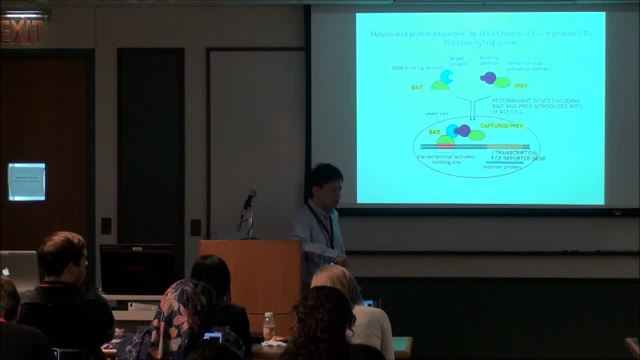 the gene expression is intact. Yeah, There was an interaction. This you don't need to do PCR. basically, You just- oh, you mean this gene expression you want to detect with PCR. Yeah, You can do that. The blue-white selection test. 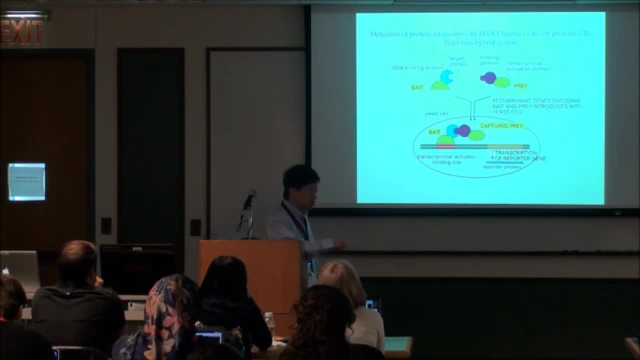 Yes, You can use PCR Or, you know, if it's convenient, you can also direct using, like green, frozen protein so that you can directly see color of the cell, Because after the gene is expressed, protein will be produced. 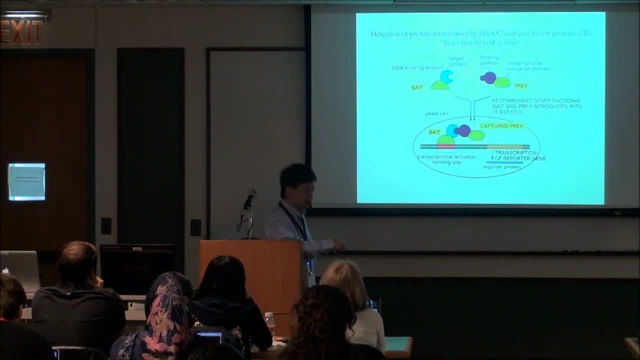